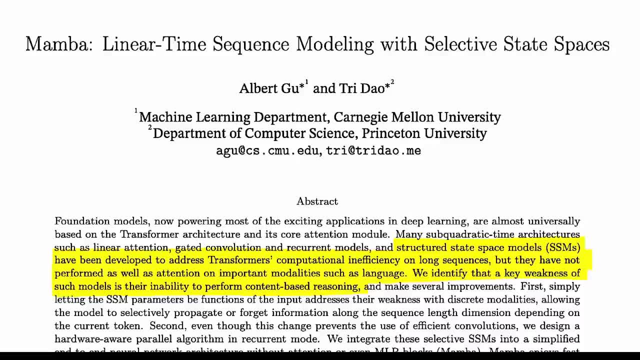 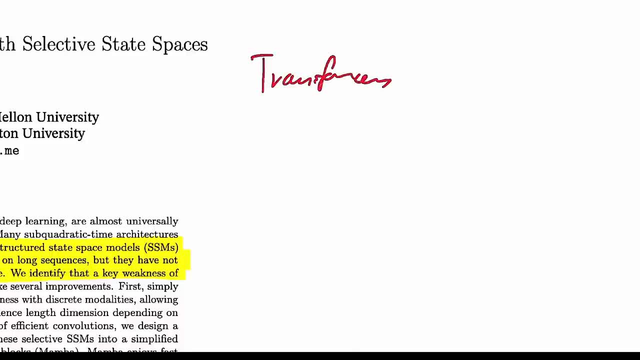 does it differ from all the other stuff that exists today? Because there are so much stuff. For example there are so there are the transformers and those obviously have their 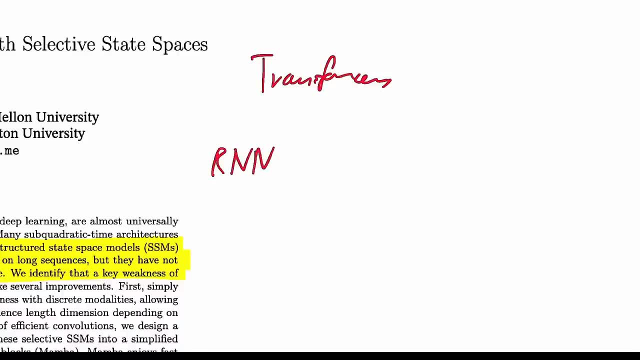 advantages and problems. Then there are on are like RNNs like recurrent neural networks and then there are these you know state space models like S4 or something like this. And there's always interesting trade-offs between all of those. Notably what we'll see is in the transformer you have if you have a sequence 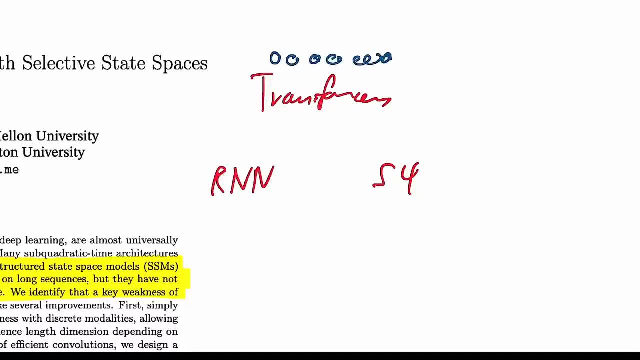 of stuff you have attention that essentially anything can look at anything else. And if you have causal attention if I look at this input I'm able to selectively look back at another input 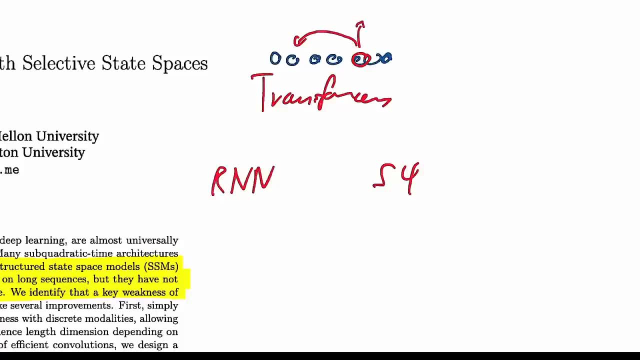 and sort of use that in the computation of the next layer here. Okay so a transformer 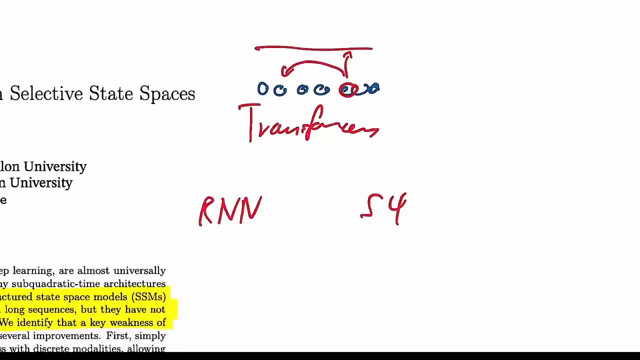 is able to dynamically and selectively look at individual elements of the past and address each one individually. But obviously you have a problem with that. So the problem with that 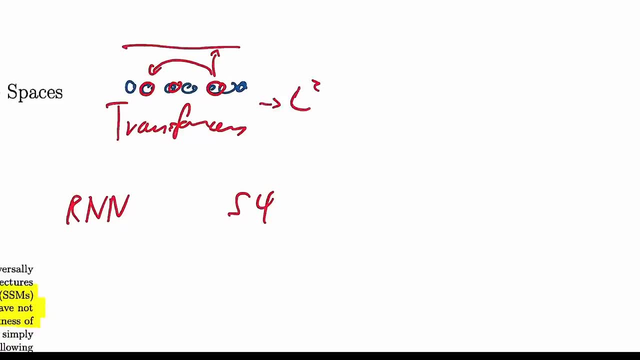 is that you have like L squared when L is the sequence length. L squared computations or N slash or and L squared memory requirements in order to do this. RNNs on the other hand 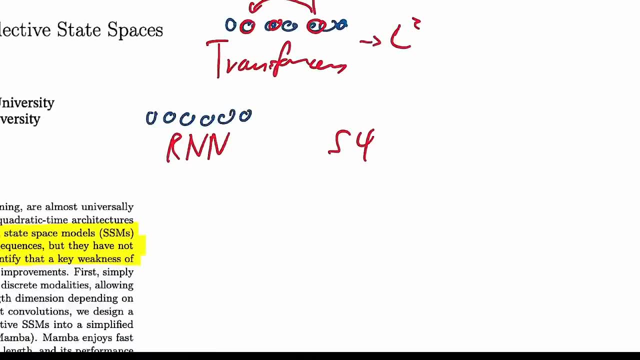 if you have a sequence there they if you consider this particular input and you want to compute the sequence length you can only look back one time step. In fact you can't even look at the last 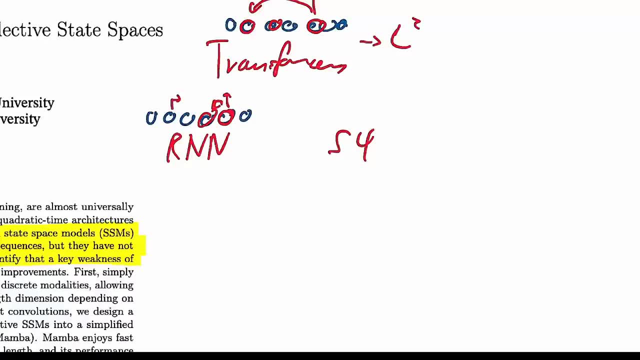 input. You what you will do is from each input you will compute a hidden state. So there is going to be some sort of a box here and you will update the box and then the next thing will come and it will update the box and then the next thing will come and it will update the box and so on. 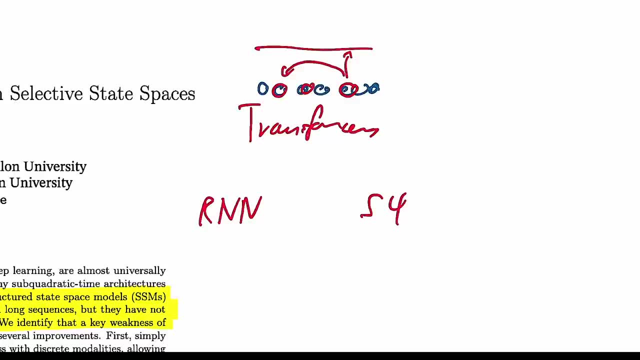 going to see in the next layer, And that's what we're going to see in the next layer, So you can use individual elements of the past and address each one individually, But obviously you have a problem with that. So the problem with that. 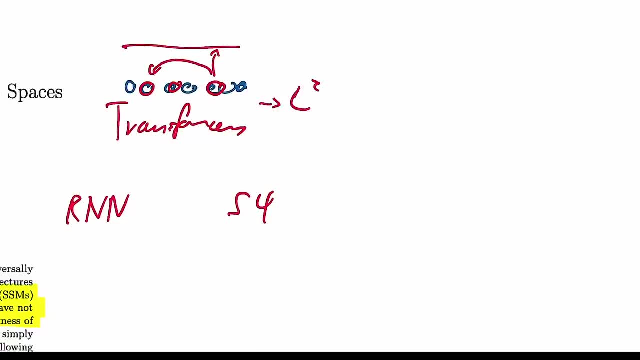 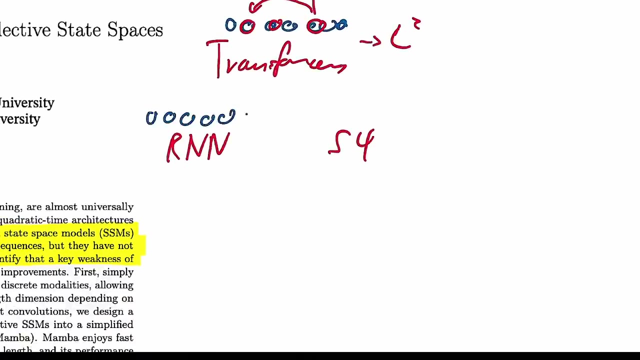 is that you have, like L squared, when, when L is the sequence length, l squared computations, or n slash or an l squared memory requirements in order to do this, RNNs. on the other hand, if you have a sequence there, they, if you consider this, 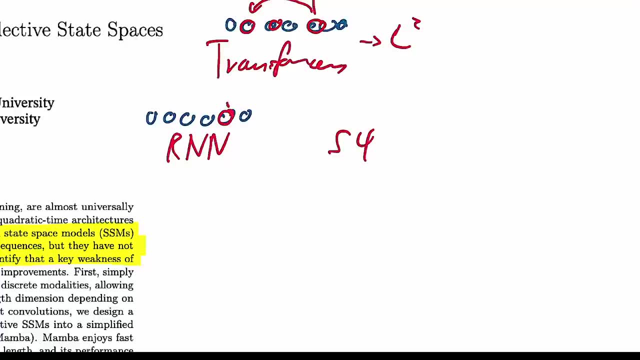 this particular input and you want to compute the next layer. you can only look back one time step. in fact, you can't even look at the last input. you what you will do is, from each input, you will compute a hidden state. so there is going to be some sort of a box here and you will update the 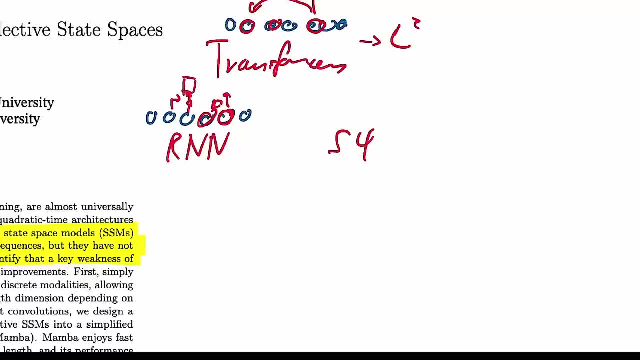 box, and then the next thing will come and it will update the box, and then the next thing will come and it will update the box, and so on. so you're only allowed to look at the last box and the current input if you want to decide what the next box here should be, and from the box you obviously 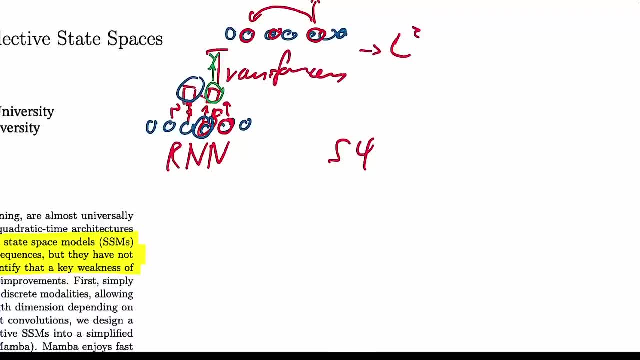 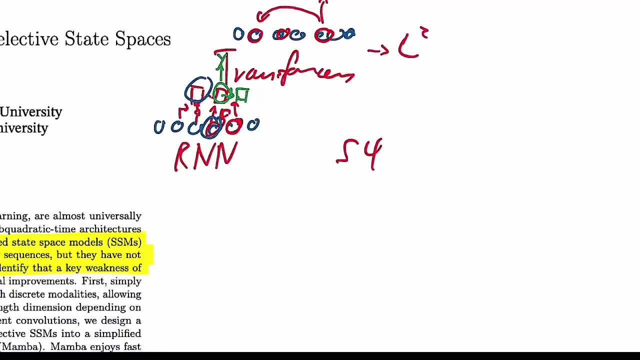 then compute the the outputs. so this is super restrictive in that you can only ever look at the last hidden state and the current input in order to compute the current output and the next hidden state, but also Also, this essentially scales to infinite lengths because it, instead of having you know, 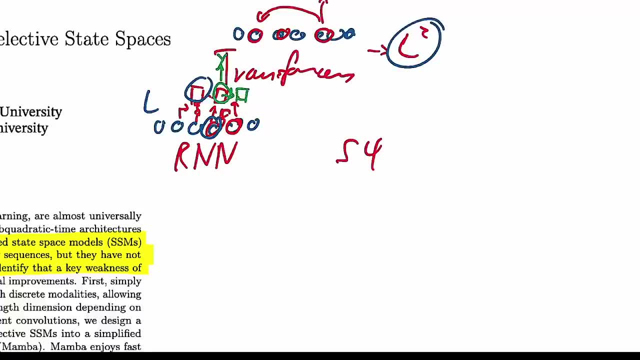 this much requirement of memory it only has. actually it doesn't even it has L computation. So you compute as many elements as you have right, But then the memory requirements are really. they're really all of one, They're really only how big is the hidden state? 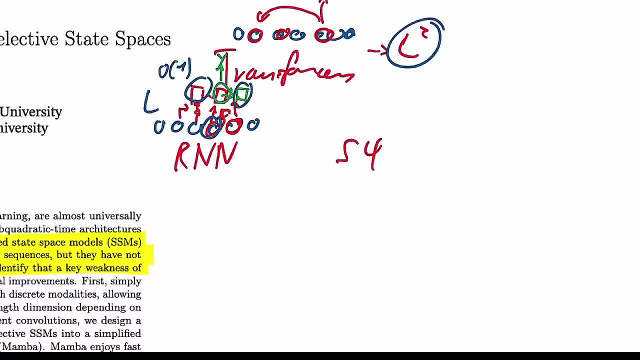 and how big are the inputs and outputs? Now, if you want to do backprop here- that's when it becomes, you know, a bit more iffy- then you will actually have to remember the whole sequence of intermediate values in order to backprop the gate. 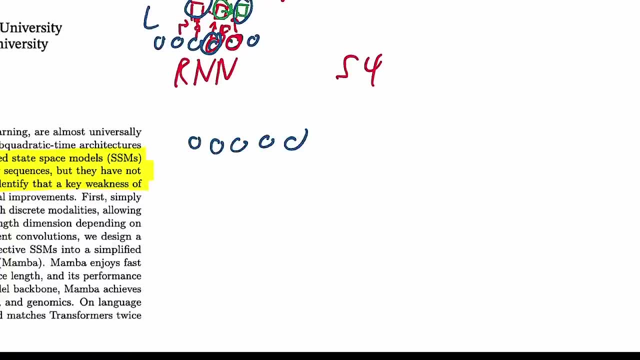 So RNNs use a thing that's called backprop through time And I know I know this is super old school and before most of you were born. but again, consider the thing where you compute the hidden state out of the last hidden state and the current input. 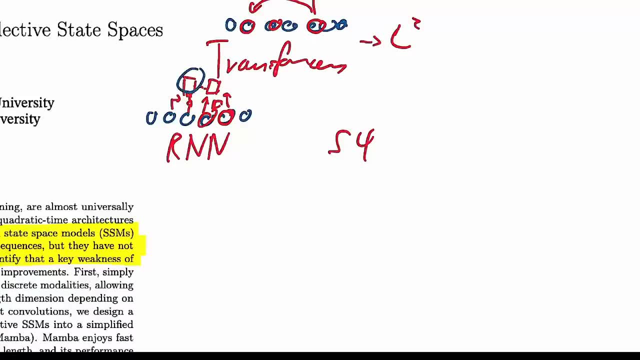 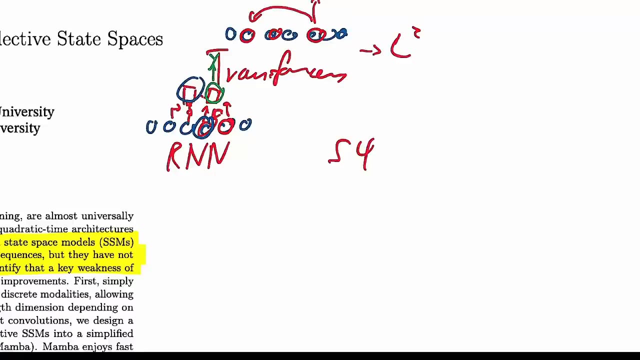 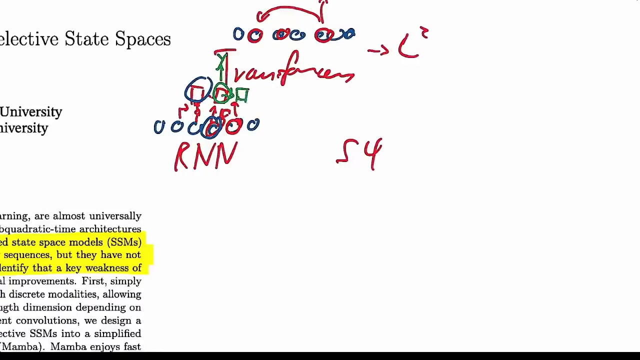 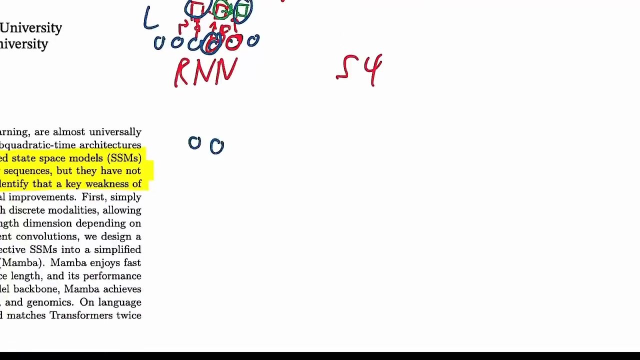 So you're only allowed to look at the last box and the current input if you want to decide what the box should be. And from the box you obviously then compute the outputs. So this is super restrictive in that you can only ever look at the last hidden state and the current input in order to compute the current output and the next hidden state. But also this essentially scales to infinite lengths because instead of having this much requirement of memory, it only has... actually it doesn't even... it has L squared. So it doesn't even have any computation so you compute as many elements as you have right but then the memory requirements are really they're really all of one they're really only how big is the hidden state and how big are the inputs and outputs now if you want to do backprop here that's when it becomes you know a bit more iffy then you will actually have to remember the whole sequence of intermediate values in order to backprop the gate so RNNs use a thing that's called backprop through time and I know I know this is super old school and before most of you were born but again consider the thing where you compute the hidden state out of the last hidden state and the current input you compute the next hidden state from that and eventually you'll have some sort of output let's say the whole sequence only has one output you can do this with many outputs too but what you want to know is 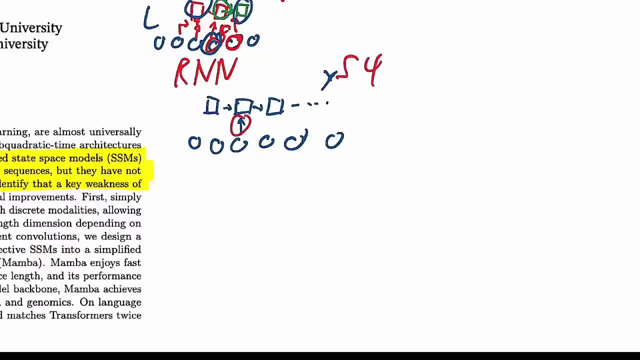 well how does the way you compute the hidden states that compute this particular transition here or this particular one how should I change that because I have some sort of loss over here well you need to backprop through 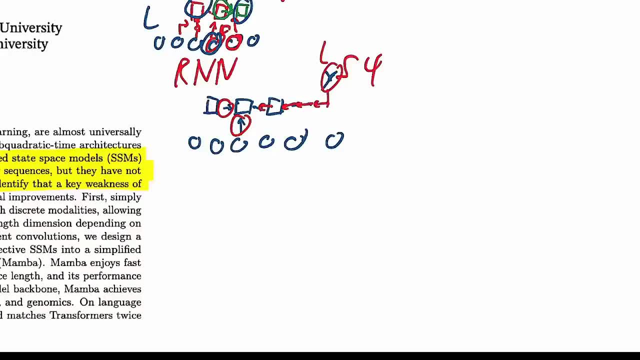 all of these computations so through all of the computations that generate the hidden states from each other and then back through this computation in order to do that that's called backprop through time and because you come you backprop through so many time steps 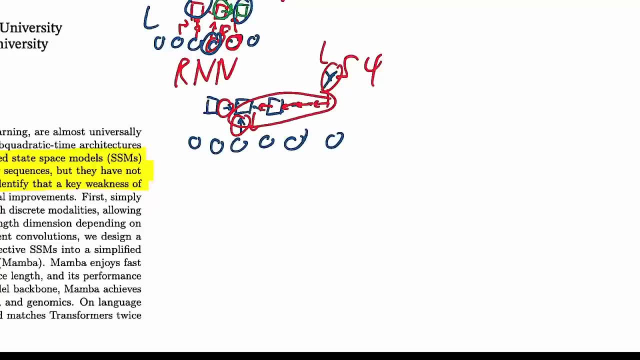 this is often either prohibitively expensive memory wise or you'll just get this vanishing or exploding gradient problems because essentially you have operation upon operation upon operation which are often multiplications solutions to that are things like the LSTM that have built-in 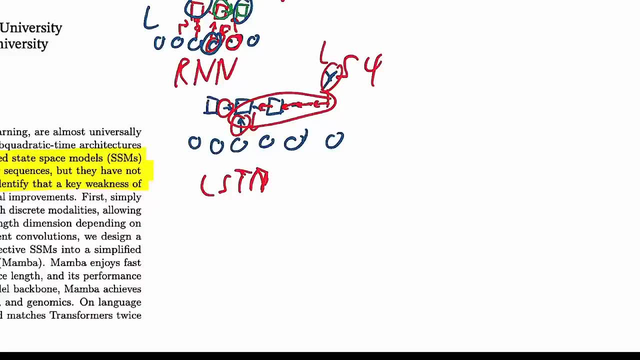 gating mechanisms but the important part to know is there is a hidden state and that goes through some transfer so there is a function and the function 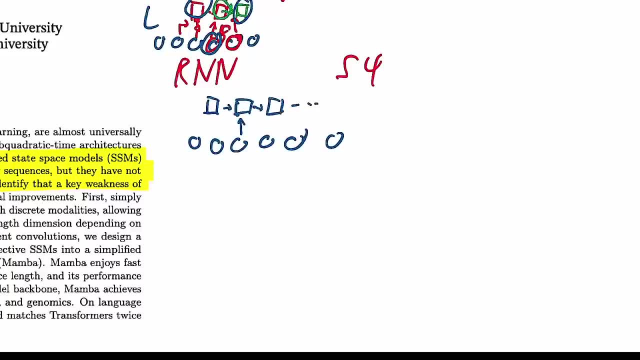 you compute the next hidden state from that, and eventually you'll have some sort of output. Let's say, the whole sequence of all the inputs and outputs is one, so it only has one output. You can do this with many outputs too, But what you want to know is: 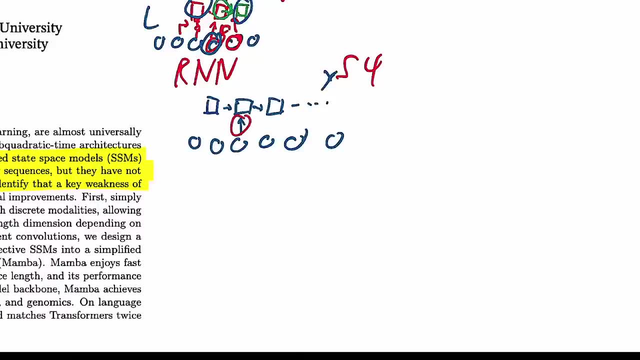 well, how does the weights that compute this particular transition here or this particular one? how should I change that because I have some sort of loss over here? Well, you need to backprop through all of these computations, So through all of the computations. 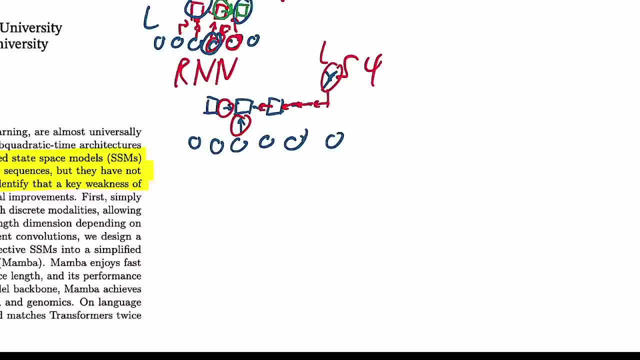 that generate the hidden states from each other and then back through this computation in order to do that. That's called backprop. So backprop through time, And because you backprop through so many time steps, this is often either prohibitively expensive, memory-wise. 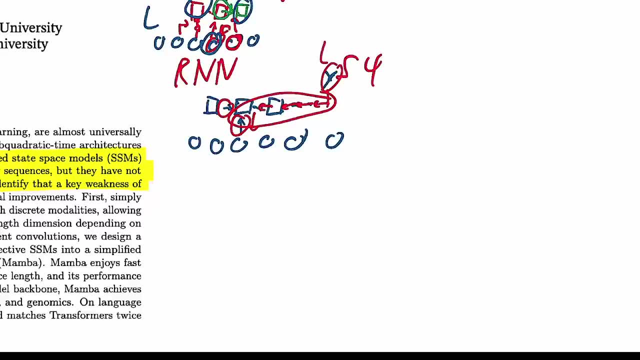 or you'll just get this vanishing or exploding gradient problems, because essentially you have operation upon operation upon operation, which are often multiplications. Solutions to that are things like the LSTM that have built-in gating mechanisms. But the important part to know is: 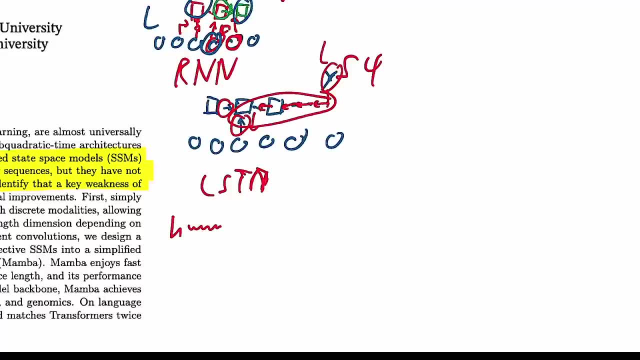 there is a hidden state and that goes through some transfer. So there is a function and the function of the next hidden state, T plus one, depends on the last hidden state and the current input. Let's see T plus one some, yeah. 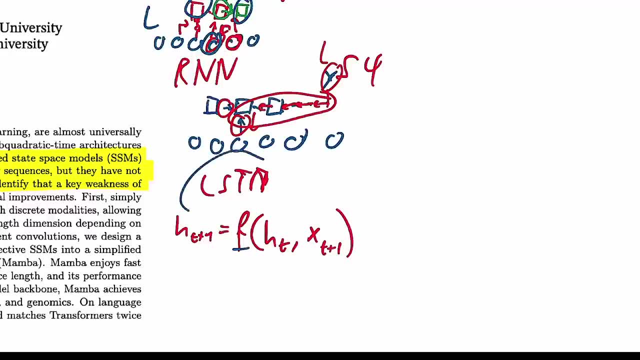 And this function here. it can be pretty much anything In an LSTM. it's a complicated gating thing in a simple recurrent network. It's just I multiply the last hidden state by some weight and then this by some weight, but it is. 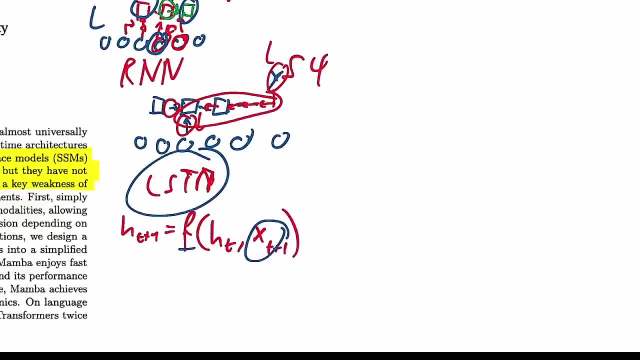 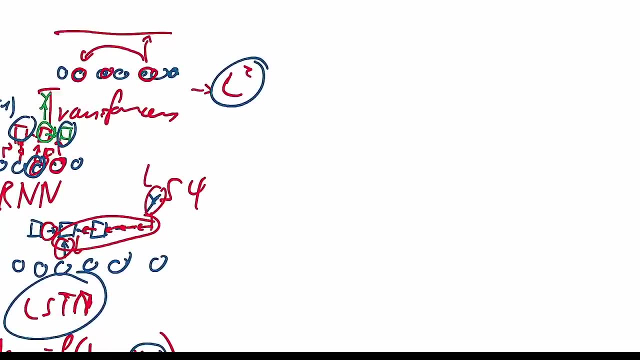 and then I add a non-linearity or something like this: Now, what about this S4 type of thing? And that's where this paper starts off. This paper starts off by saying, hey, look at these state space models. They've been pretty. 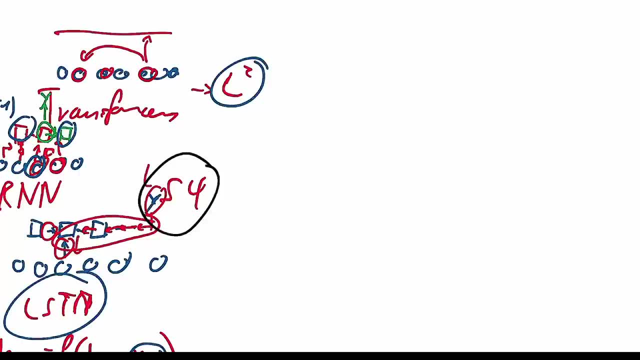 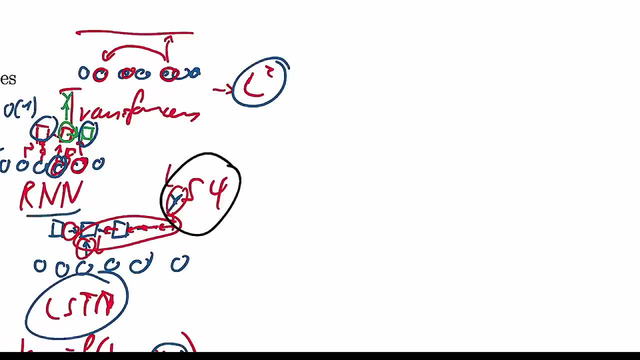 we've built some of these and they have some nice properties. What are those The nice properties? The nice properties are that they essentially are an RNN essentially, but when they have a sequence and a sequence of inputs, they can essentially compute all of the outputs. 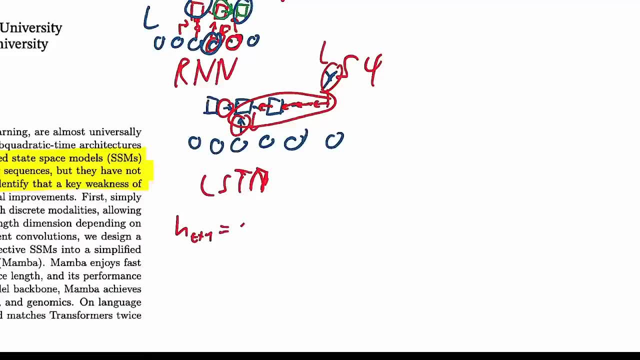 of the next hidden state t plus one depends on the last hidden state and the current input t plus one some yeah and this function here it can be pretty much anything in an LSTM it's a complicated gating thing in a simple recurrent network it's just I multiply the last 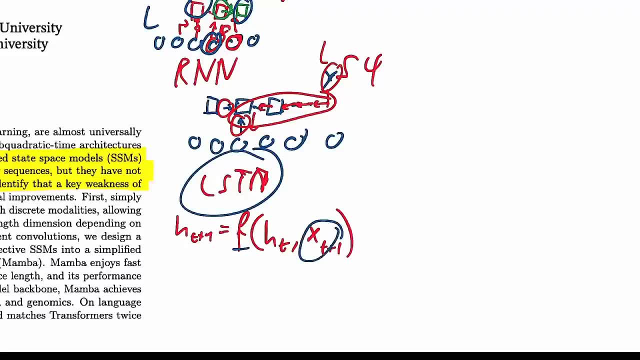 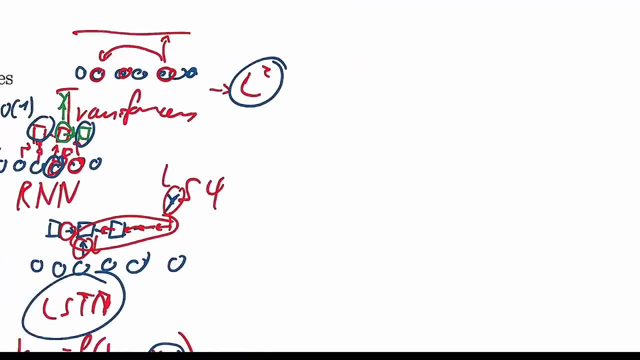 hidden state by some weight and then this by some weight but it is uh and then and then I add a non-linearity or something like this now what about the this s4 type of thing and that's 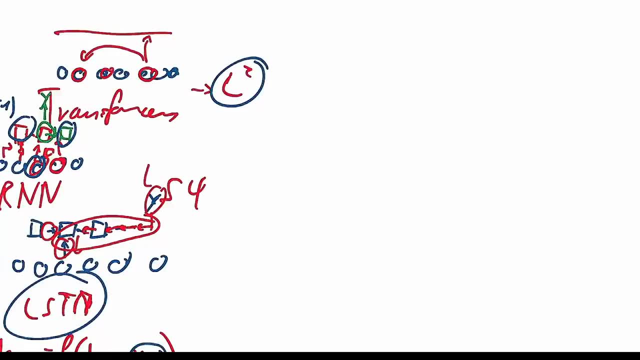 where this paper starts off this paper starts off by saying hey look at these these uh state space models they've been pretty we've built some of these and they have some nice properties 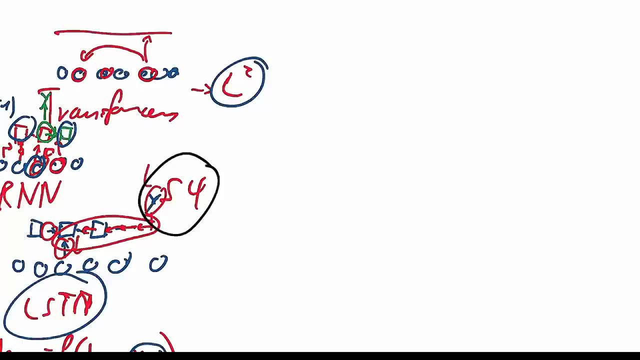 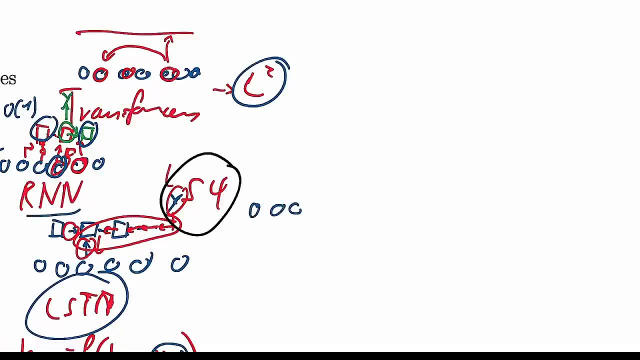 what are those nice properties the nice properties are that they essentially are an RNN essentially but when they have a sequence 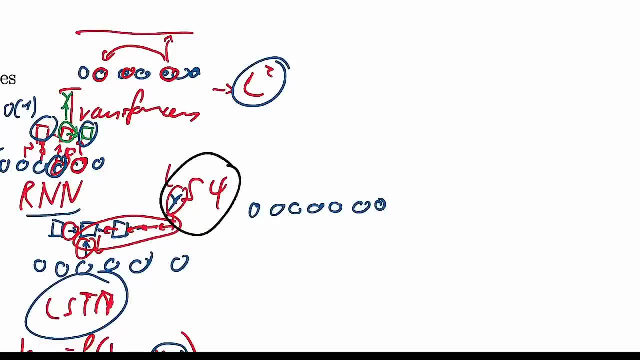 and uh so a sequence of inputs they can essentially compute all of the outputs if there are multiple outputs or that single output over here 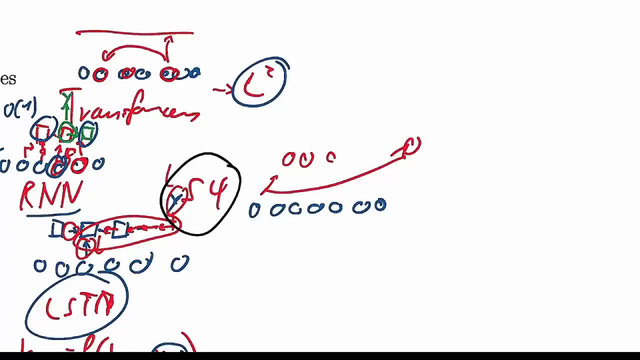 in one swoop so they can essentially compute it like zoom um in one big swoop and so if they have all the inputs they can just formulate this as a convolution operator and there are multiple 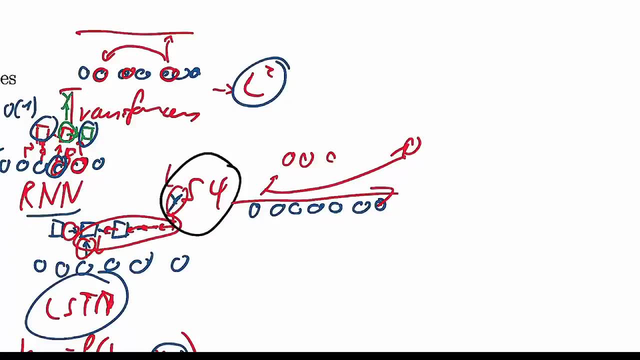 why that's the case but two main reasons first reason there is no non-linearity going from the 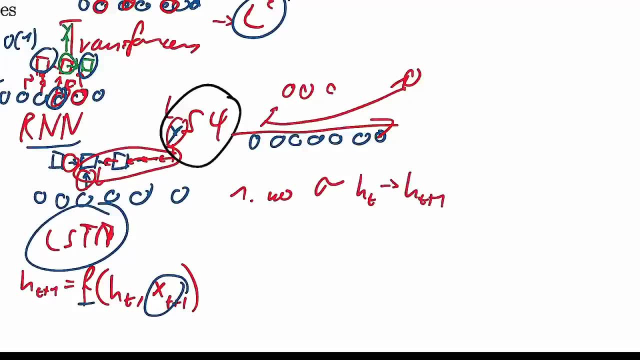 last hidden state to the next hidden state right so that this this is a completely linear transition if you will we'll go a little bit into what i mean by this obviously here 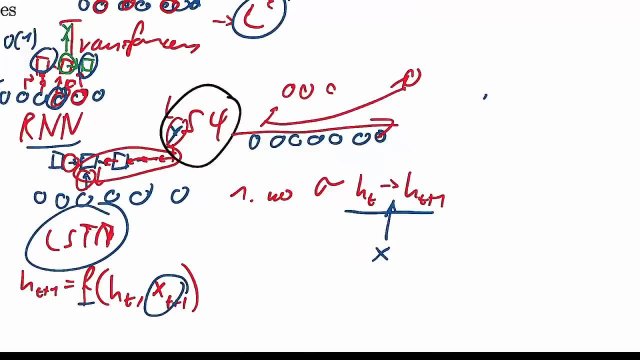 here some kind of x is coming in and that doesn't necessarily need to be linear but sort of the backbone of this going through time from hidden state to hidden state are linear computations 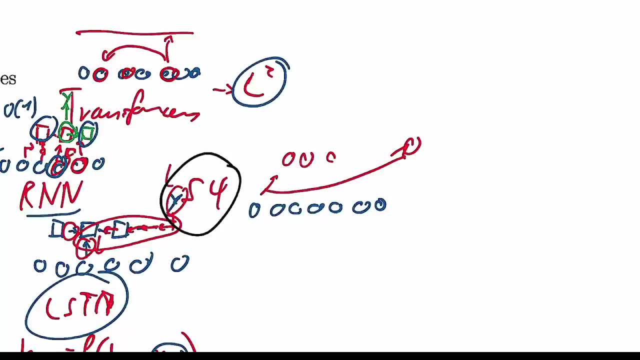 if there are multiple outputs or that single output over here in one swoop. So they can essentially compute it like zoom in one big swoop, And so if they have all the inputs they can just formulate this as a convolution operator. 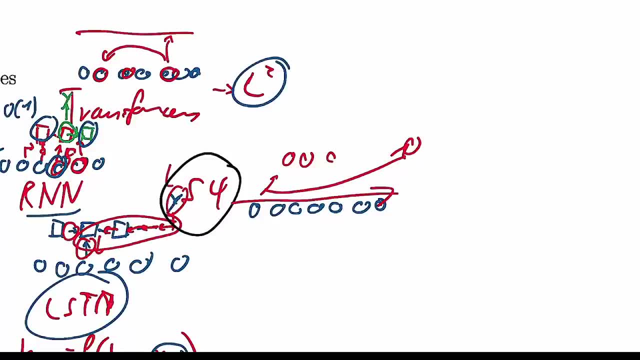 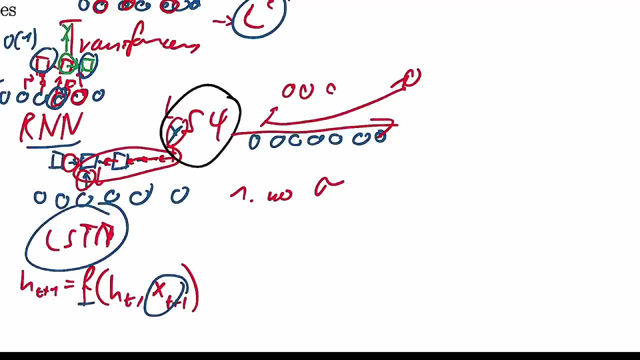 And there are multiple reasons why that's the case, but two main reasons. First reason: there is no non-linearity going from the last hidden state to the next hidden state, right? So this is a completely linear transition. if you will, We'll go a little bit into what I mean by this. 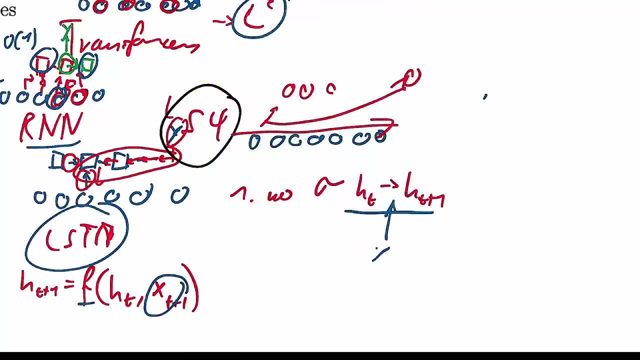 obviously here some kind of X is coming in and that doesn't necessarily need to be linear, but sort of the backbone of this- going through time from hidden state to hidden state- are linear computations. So no non-linearity involved in that. What does that? 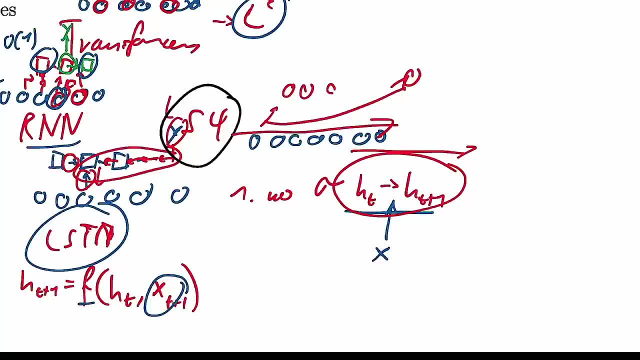 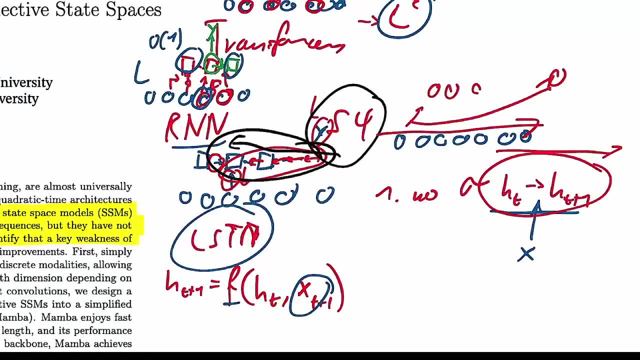 what that will mean is that essentially the whole this whole path here, this whole back prop through time thing, is going to be at least the path that goes back the hidden states until it branches off into the individual elements. That is essentially one big matrix multiple. 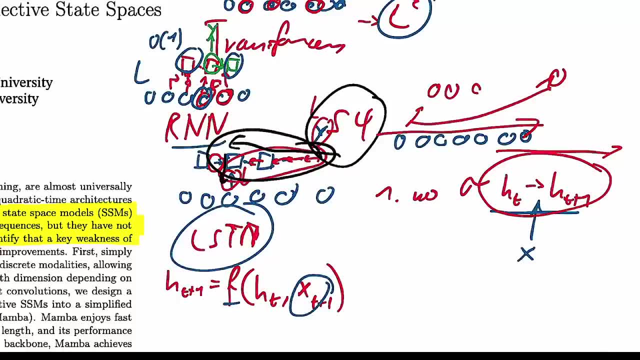 like one big linear operation, And that is a lot more well-behaved than if you also have the non-linearities in between. Now, obviously, you can still have exploding or vanishing gradients and so on, So you could also- you can- still have that. 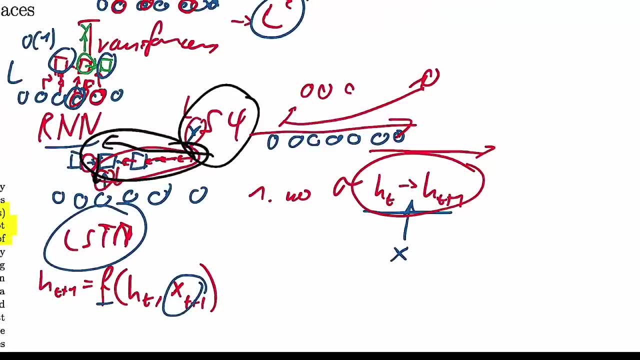 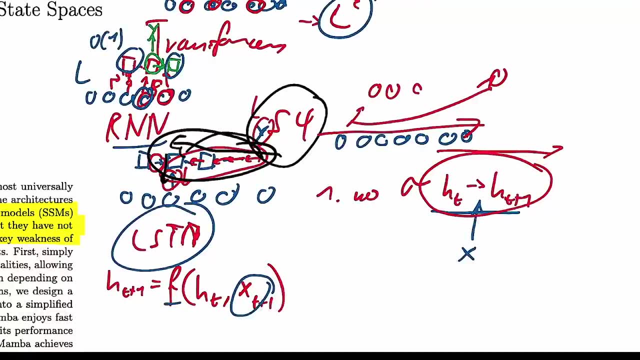 but it is a lot more easy, let's say, than having complicated gating mechanisms there, And what it means is that you can just kind of jump ahead to any point that you want, because you can always. you always know what the full operation is. 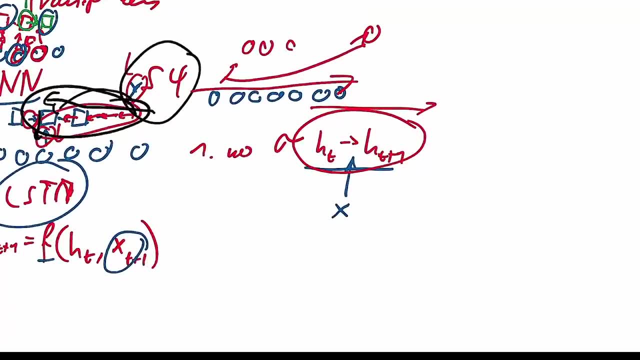 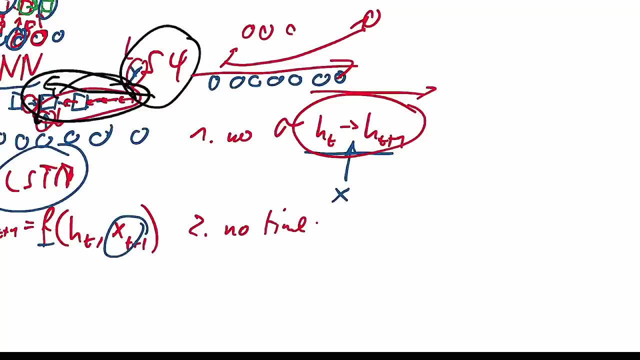 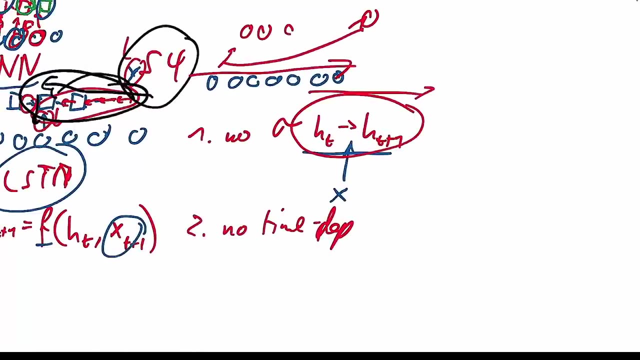 You always have a closed form to that Second. okay, what's second? There is no time dependence, So there's no time dependence of these things and no input dependence. What that means is that the transition from state one to state two is going to be the same. 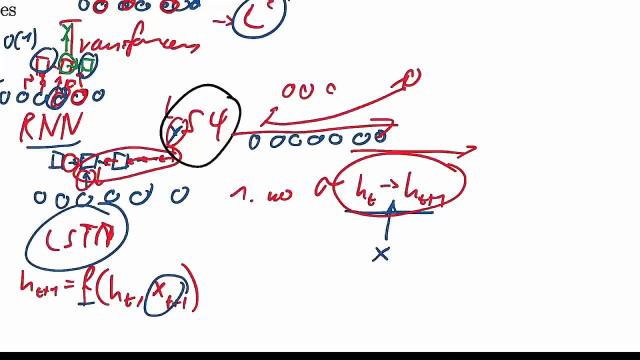 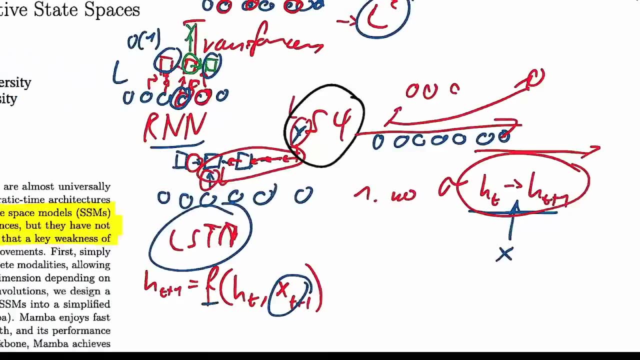 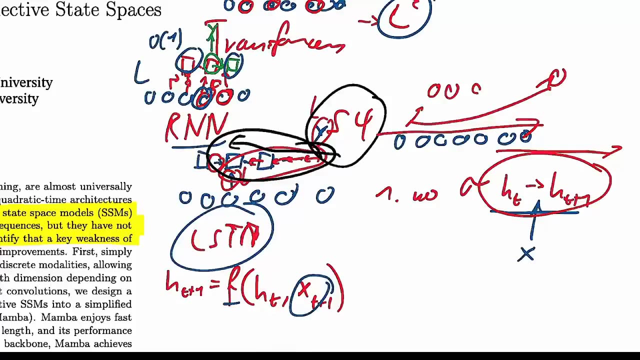 so no non-linearity involved in that what does that what that will mean is that essentially the whole this whole path here this whole back prop through time thing is going to be at least the path that goes back the hidden states until it you know branches off into the individual elements 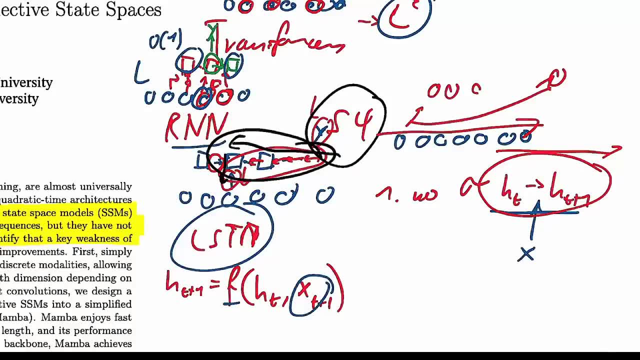 that is essentially one big matrix multiple like one big linear operation and that is a lot more well behaved than if you also have the non-linearities in between now obviously you can 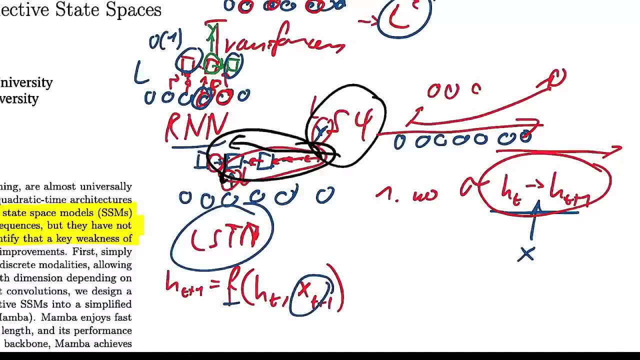 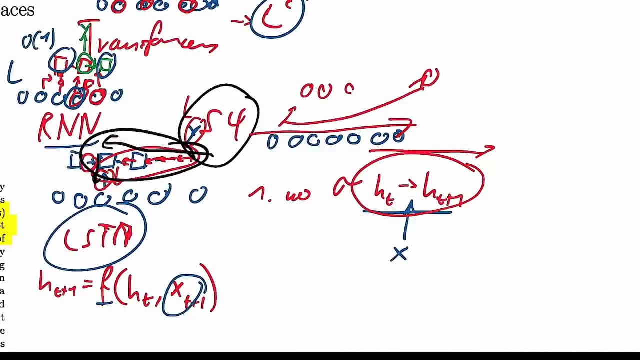 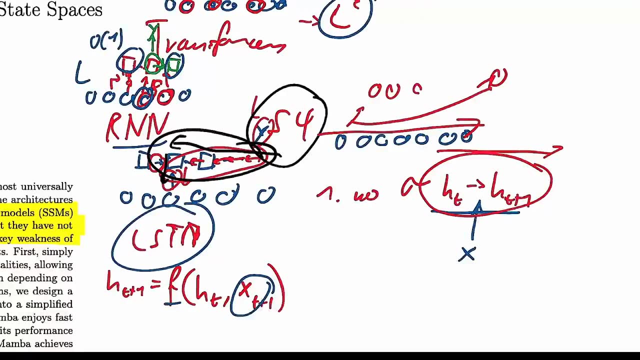 still have exploding or vanishing gradients and so on so you could also you can still have that but it is a lot more easy let's say than having complicated gating mechanisms there and what it means is that you can just kind of jump ahead to any point that you want because you can always 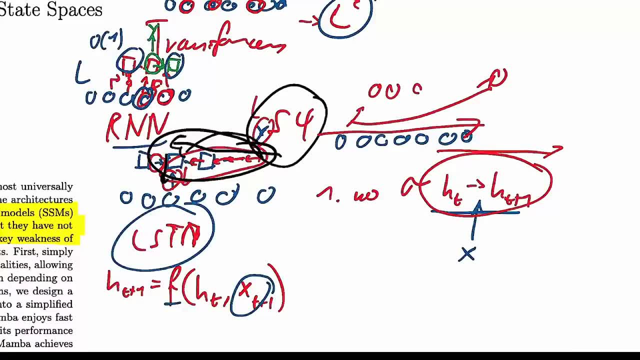 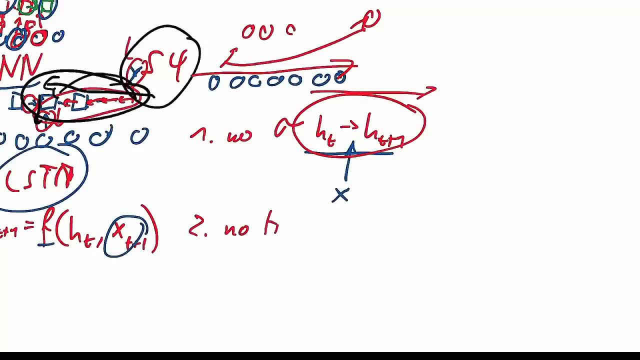 you always know what the full operation is you always have a closed form to that second okay what's second there is no time dependence so there's no time dependence of these things and no input 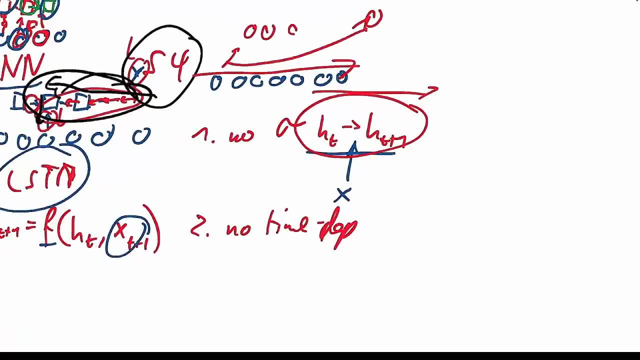 dependence what that means is that the transition from state one to state two is going to be the same as the transition from state two to state three now again there is going to be inputs in these um that obviously don't always compute the same function but the transition between the time steps and how you incorporate new information is always the same so all the matrices that are 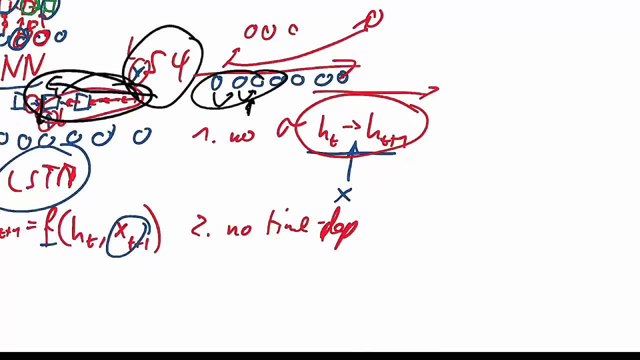 involved in here essentially are all the same and not dependent on the input at all and therefore you can just kind of 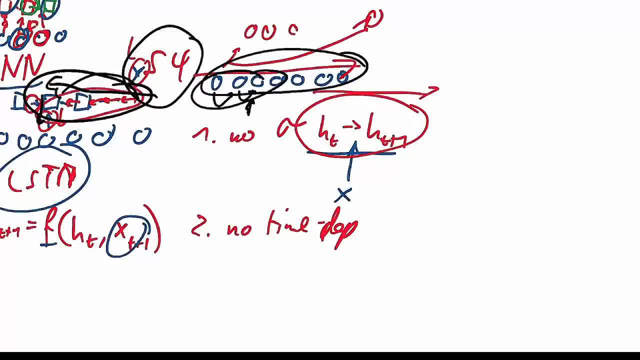 pre-compute all of the aggregation right here and then all you have to do is kind of multiply in your individual inputs from the time steps and you can just compute the whole thing as as one 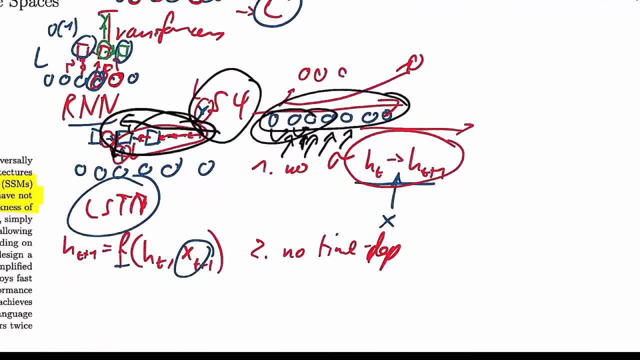 big computation so that's what we're going to look at the question is where do the these uh where does mamba fit in mamba is an 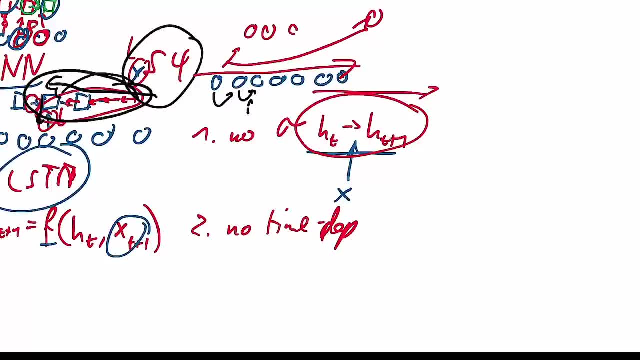 as the transition from state two to state three. Now, again, there is going to be inputs in these that obviously you don't always compute the same function, but the transition between the timesteps and how you incorporate new information is always, let's say, 2020.. 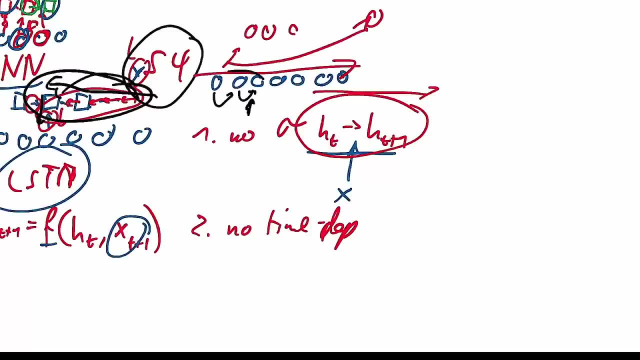 always the same. So all the matrices that are involved in here essentially are all the same and not dependent on the input at all, And therefore you can just kind of pre compute all of the aggregation right here And then all you have to do is kind of multiply in your 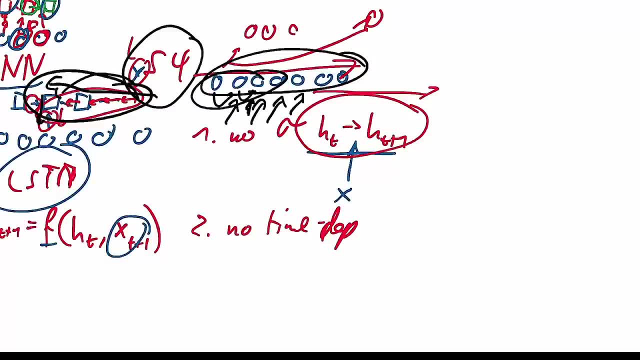 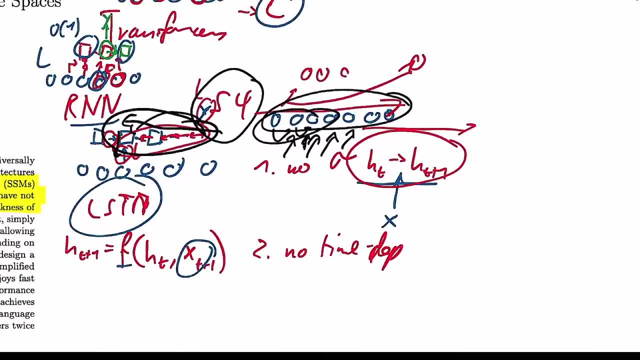 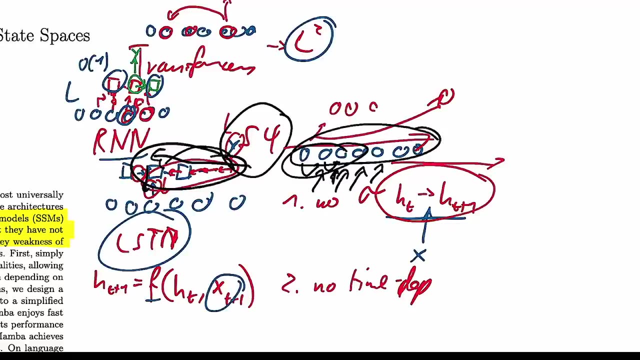 individual inputs from the time steps And you can just compute the whole thing as as one big computation. So that's what we're going to look at. The question is, where do the these? where does Mamba fit in? Mamba is an architecture that makes use of what they call selective state spaces. 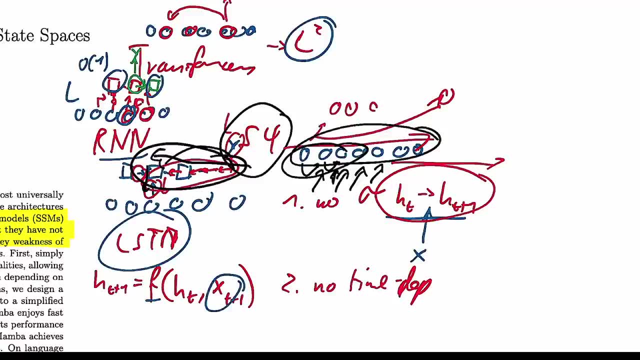 and selective state spaces relaxes this property of S4 a bit, And what I mean by the property that the transition from time step to time step is independent of the input. it relaxes that a little bit And therefore it moves the input from time to time step to time step. 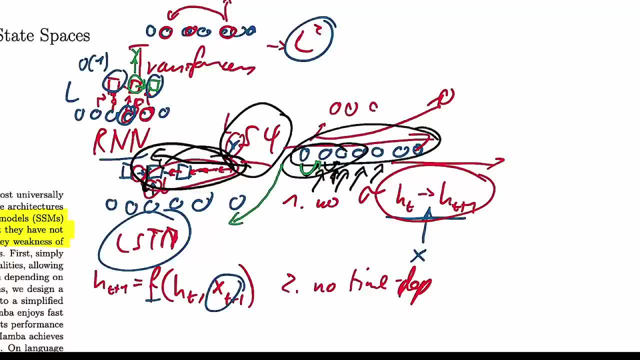 S4 a little bit closer into the direction of LSTMs, And and, but it remains, it retains this property, that the, the backbone here- is computable by one swoop, And we're gonna, they're gonna do this as a, as a prefix sum, as a parallel scan. It's, it's compute computable as one swoop, And 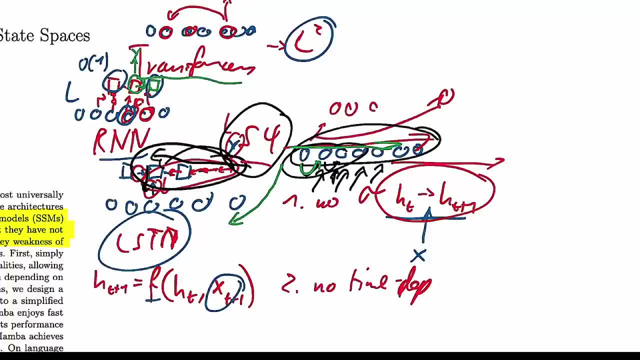 therefore, during training it looks more like a transformer where you can just compute all of the forward passes of the whole sequence in one go, instead of like the LSTM, where the forward pass no matter whether you know all the inputs already. you have to compute the forward pass one after another. 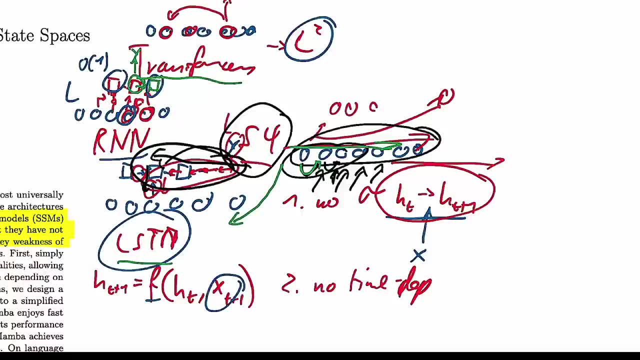 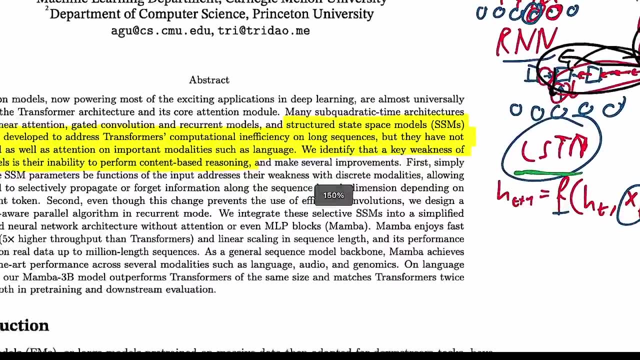 So during training it looks more like a transformer And during inference it actually looks more like an, like an LSTM. All right, So we'll dive in into the paper And I just. I have a few sections highlighted, not too much, especially the. 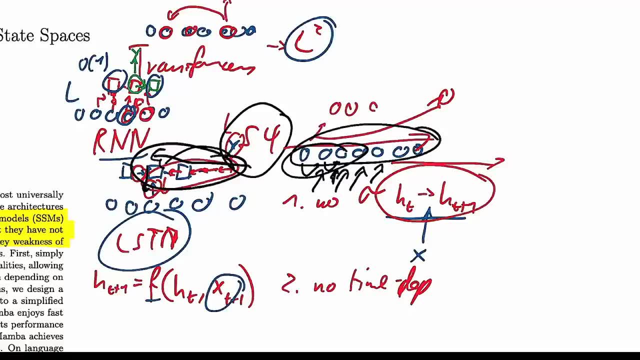 it just it looks just kind of a charged point so that's what you take in the brain 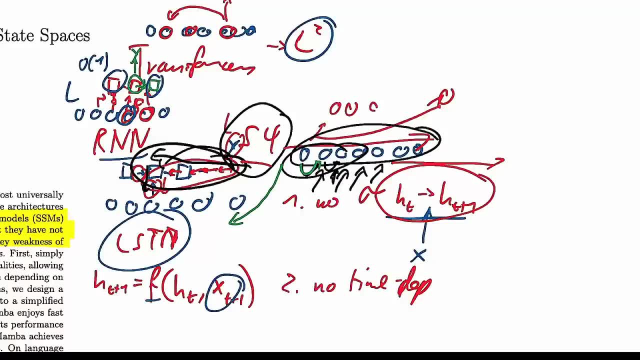 now let's see how this works let's take this look and look to go over this size and let's take this 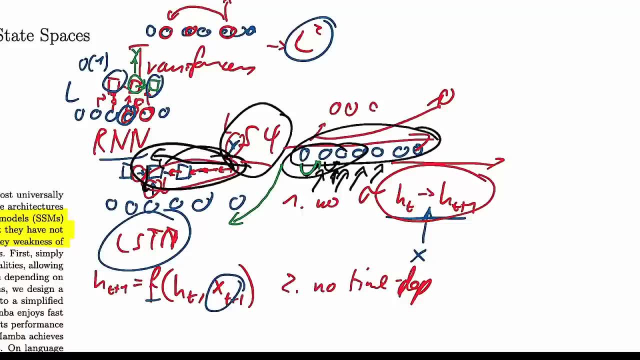 But it remains, it retains this property that the backbone here is computable by one swoop. 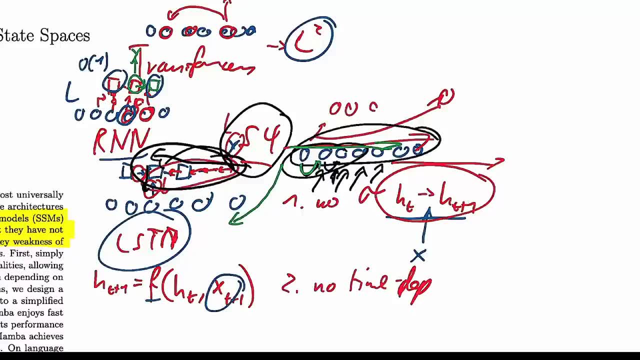 And they're going to do this as a prefix sum, as a parallel scan. It's computable as one swoop. 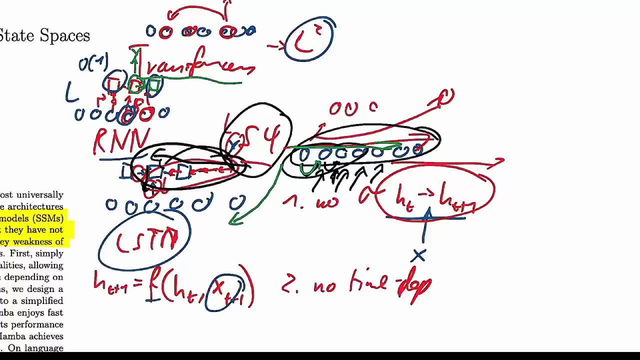 And therefore, during training, it looks more like a transformer, where you can just compute all of the forward passes of the whole sequence in one go, 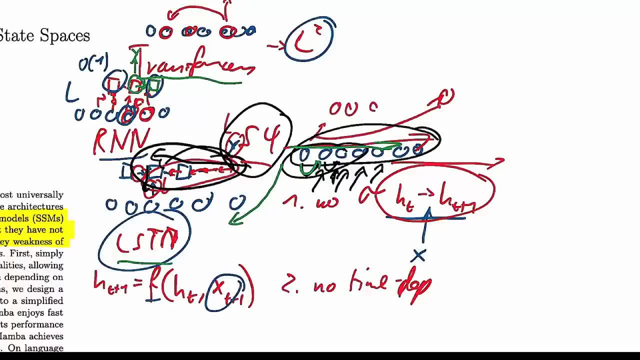 instead of like the LSTM, where the forward pass, no matter whether you know all the inputs already, you have to compute the forward pass one after another. 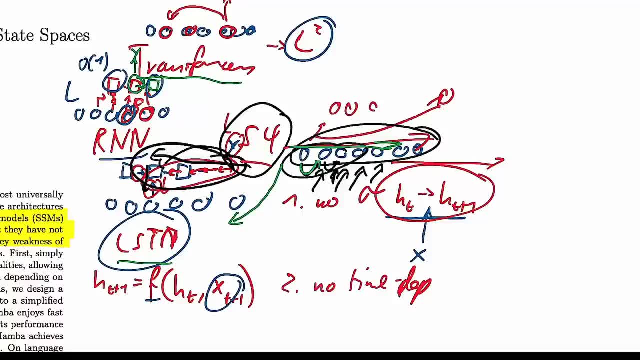 So during training, it looks more like a transformer. And during inference, it actually looks more like an LSTM. All right. 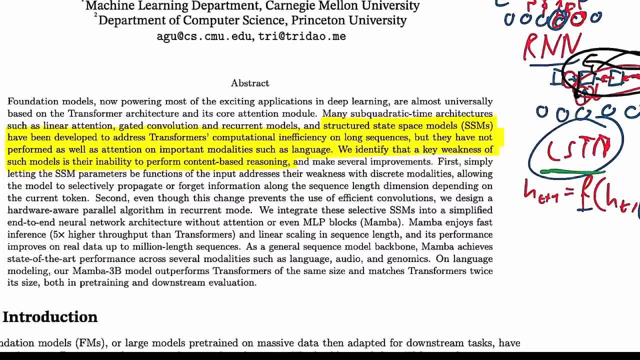 So we'll dive into the paper. And I have a few sections highlighted. 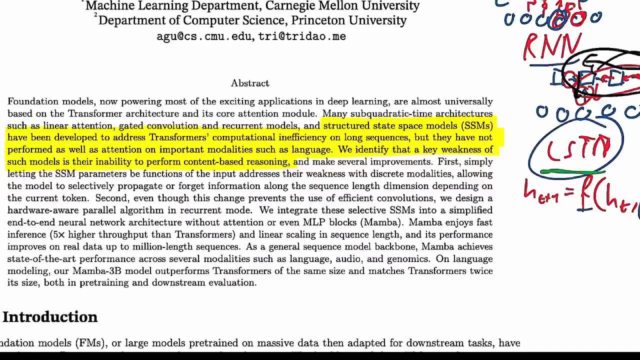 Not too much, especially the experimental results. You're very welcome to look at those. 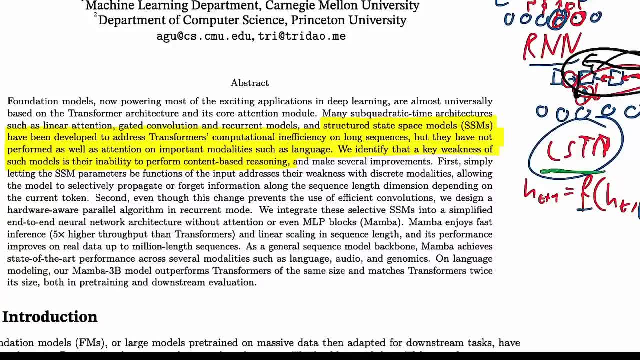 The result is going to be that it is a strong competitor to transformers so far. 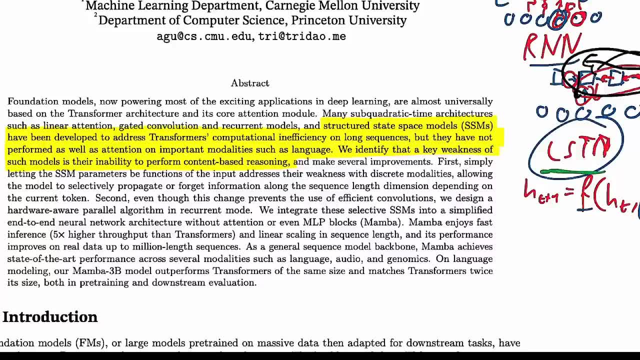 They have not made experiments up to the bigs, like up to the big transformers and big. 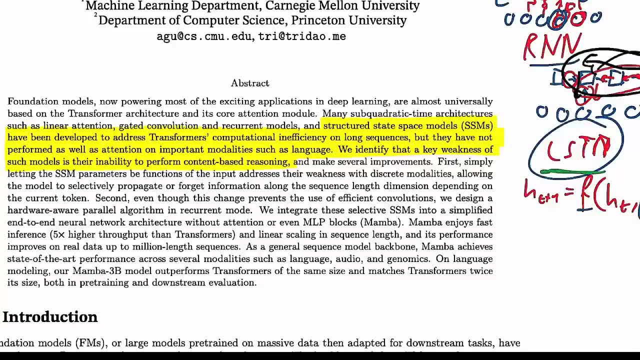 So I believe they have made experiments up to about 1 billion parameters. That's obviously really big in conventional terms. 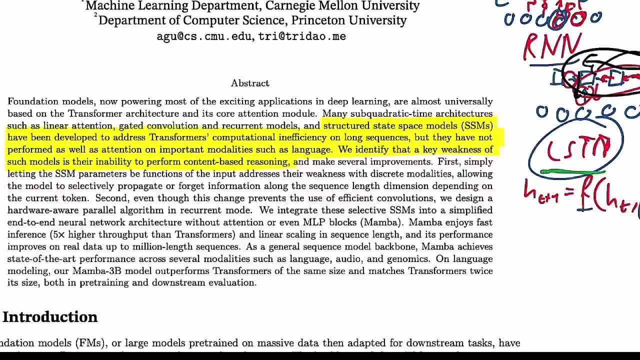 experimental results. you're very welcome to look at those. the result is going to be that it is a strong competitor to transformers. So far they have not made experiments up to the big like up to the big transformers and big. So I believe they have made experiments up to about 1 billion. 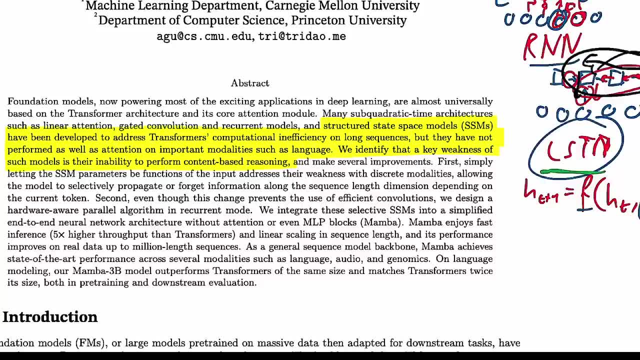 parameters, That's obviously really big in conventional terms, But for language modeling the smallest ones start at like 7 billion. So that remains to be seen, But the scaling laws seem to be promising. The other thing is that they say themselves: it really excels at when you need. 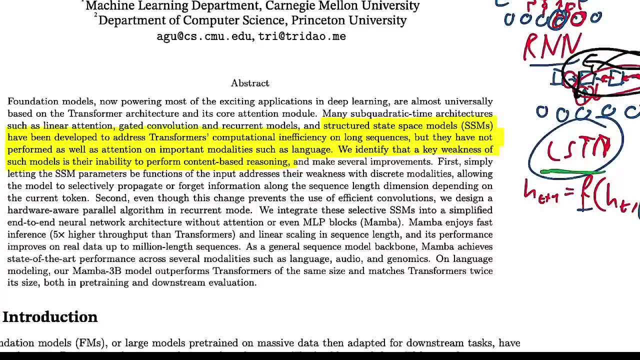 really really long sequences, like DNA modeling or audio waveforms and so on. They're having a long context, And being efficient with that is probably more important than this. you know, super ability to have transformers to focus in on individual states. All right, So they say: 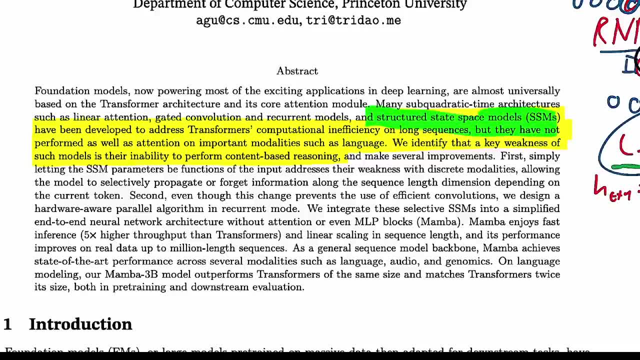 structured states based models- sorry- have been well up to address transformers, computational efficiency on long sequences, but they've not performed as well as attention on important modalities such as language. we identify a key week, that a key weakness of such models is their. 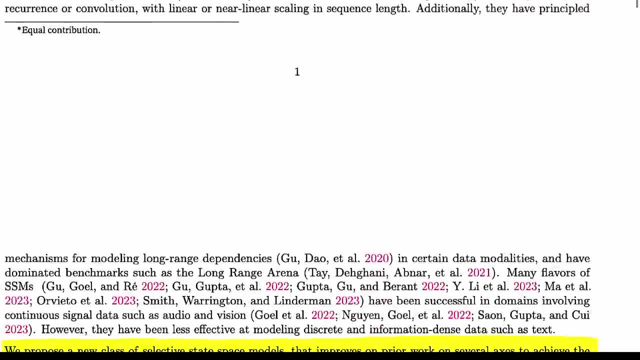 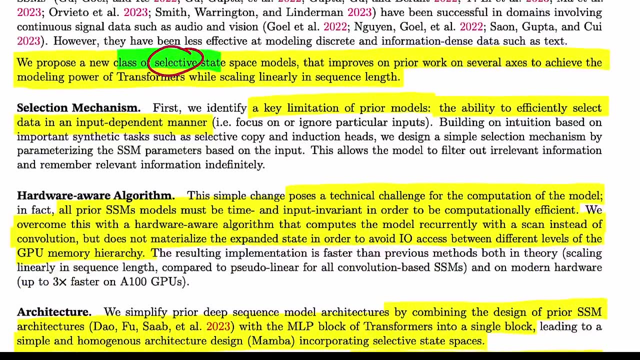 inability to perform context based reasoning. What does that mean? They say we propose a new class of selectors. And what does that mean? We propose a new class of complex data, which is a relatively small amount of data, And what we propose is a much larger range of data than the average number of. 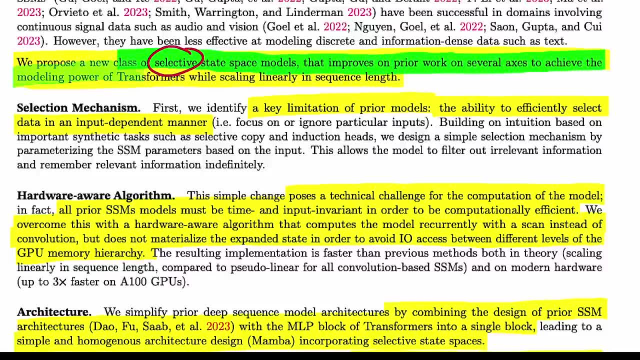 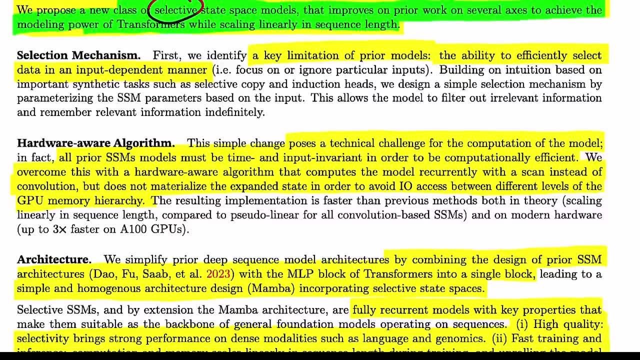 data, And this is the data we propose. So the different aspects of pre-existing model structure move in that direction. we propose a more correct method of looking at the data. we propose a more realistic solution to the model structure, a more�y way of looking at the model structure. 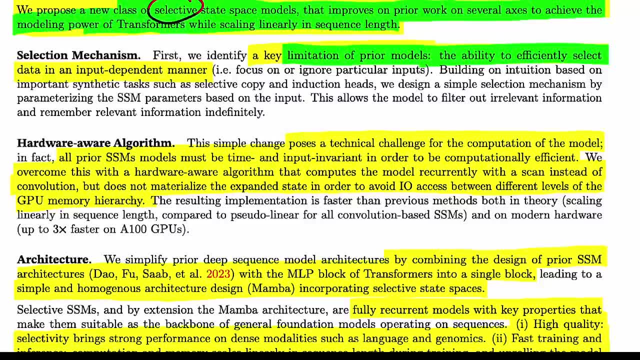 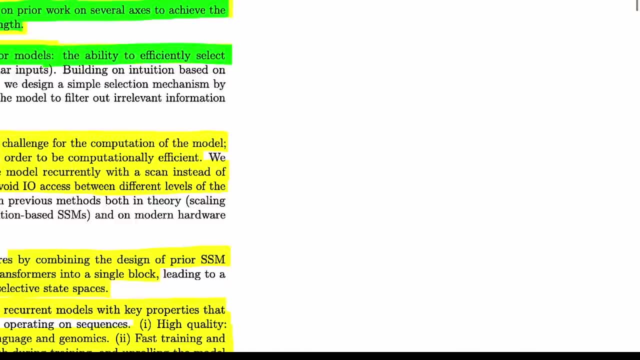 and we propose a much more efficient model structure. Another, more efficient way of looking at the model structure is we propose a more objective state based model right. the selective is the difference instead of the structured. that in pole improves on prior work on several axes to achieve. 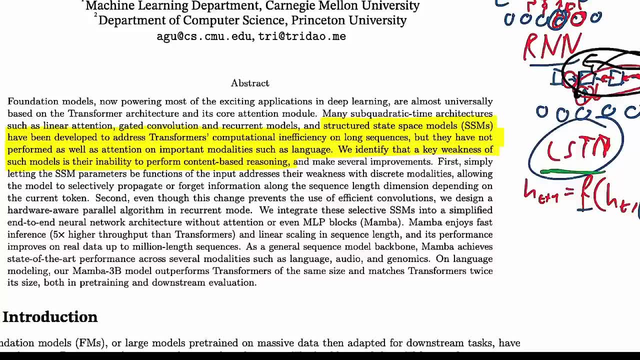 But for language modeling, the smallest ones start at like, 7 billion. 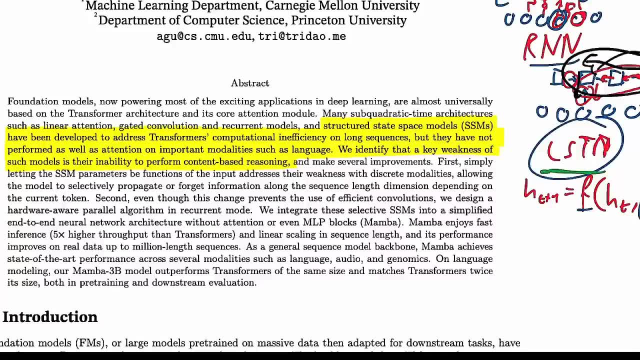 So that remains to be seen. But the scaling laws seem to be promising. 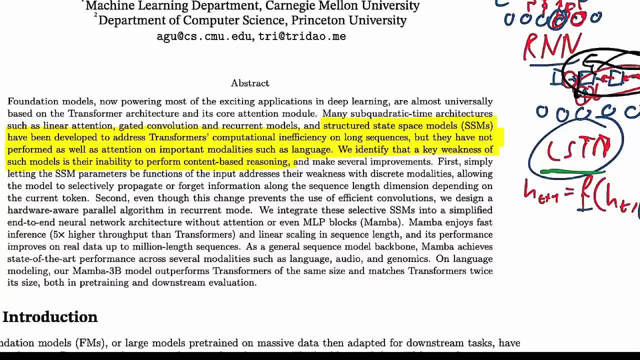 The other thing is that they say themselves, it really excels at when you need really, really long sequences, like DNA modeling or audio waveforms and so on. 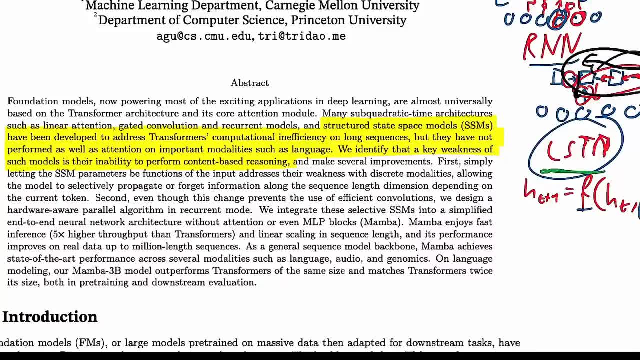 They're having a long context and being efficient with that is probably more important than this, you know, super ability of transformers to focus. In on the individual states. 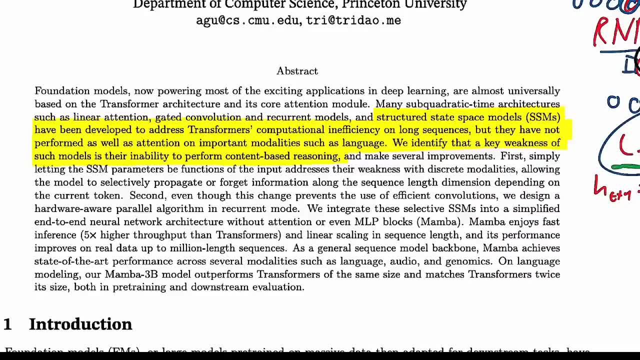 All right. So they say structured state space models, sorry, have been well up to address transformers, computational efficiency on long sequences, but they've not performed 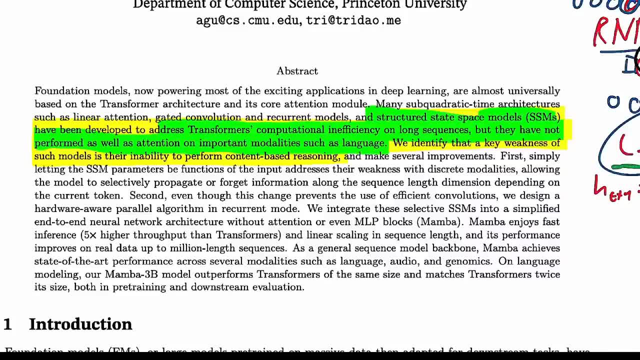 as well as attention on important modalities, such as language. 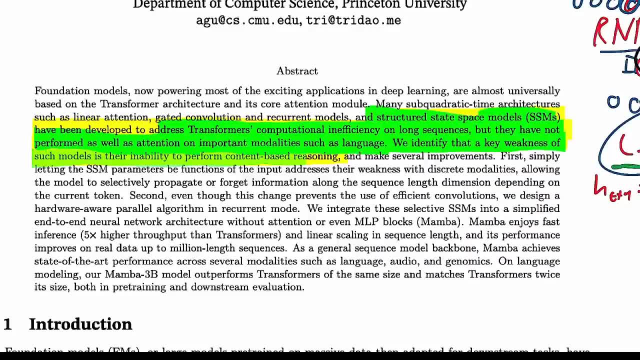 We identify a key week that a key weakness of such models is their inability to perform context based reasoning. 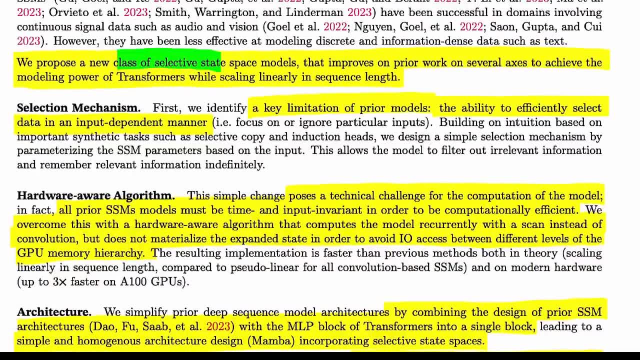 What does that mean? They say we propose a new class of selective state space model, right? The selective is the difference. 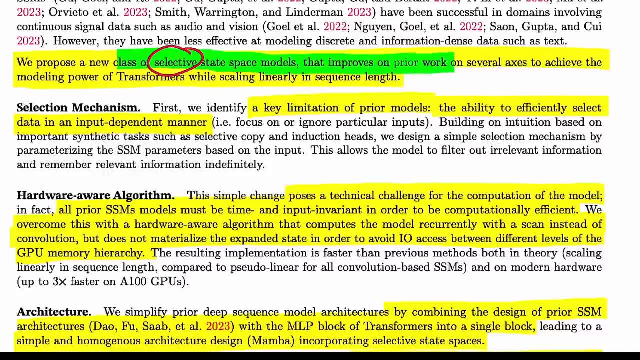 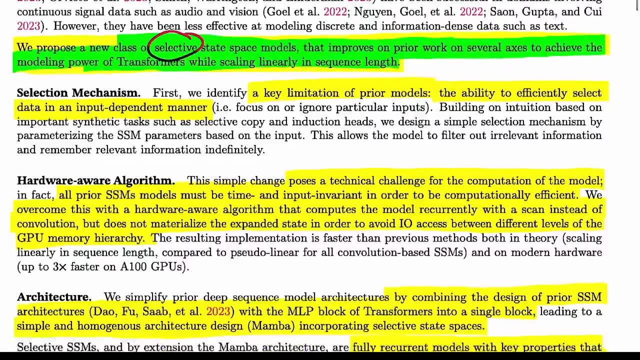 Instead of the structured that in poll improves on prior work on several axes to achieve the modeling power of transformers while scaling linearly in sequence length. 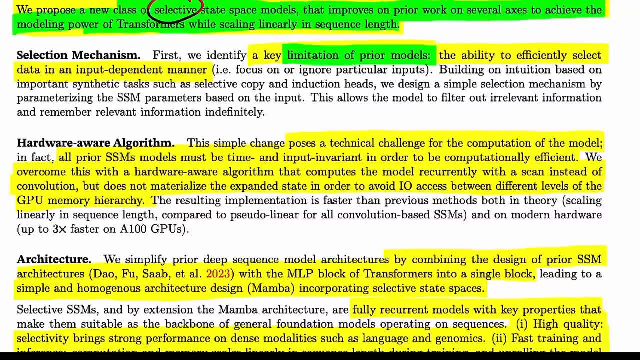 So they say a key ability, key limitation of prior models, the ability to efficiently select data in an input dependent manner. 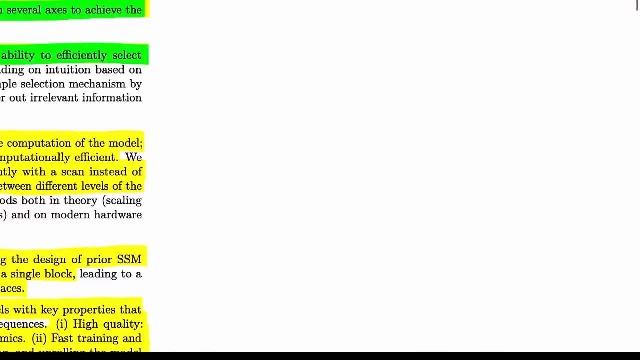 Again, what does, what does that mean? You have a previous hidden state. You have a current input. And you want to build the next hidden state T plus one, what structured state space models do is they have, they'll have some kind of per parameterized function. 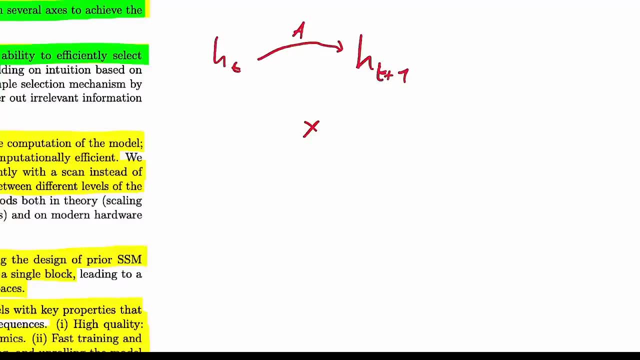 Let's call that a, and they'll have some sort of, uh, they'll have some sort here. Let's call that B even though it's, it's slightly different, but, and the result is going to be that H T. 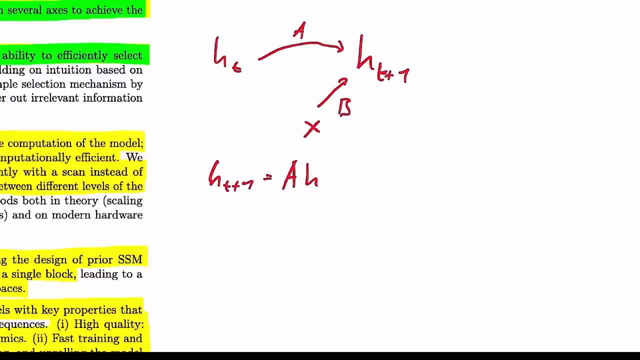 Plus one is going to be equal to something like a H T plus B X. Okay. 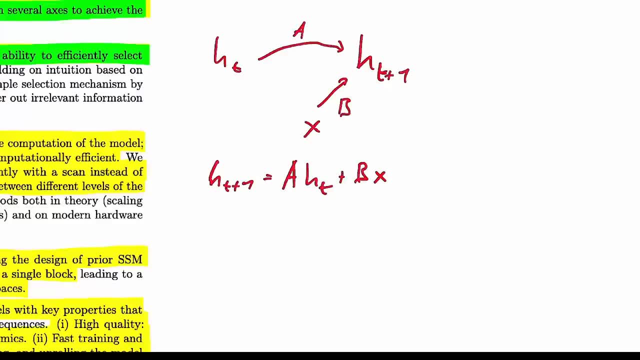 Again, not exact representation, but in principle, this and this is in SSMs. 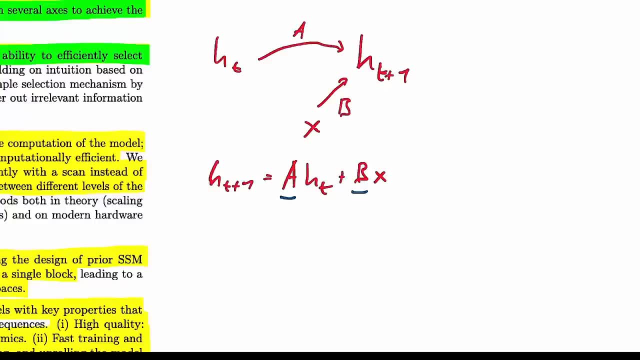 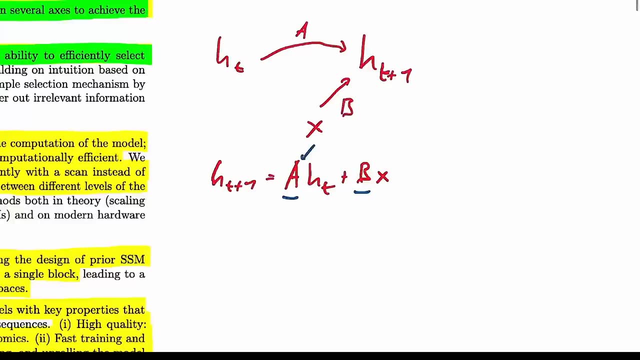 Like is going to be completely fixed for the whole sequence always. So you learn one set of parameters or, you know, one, a and one. Can you do that? 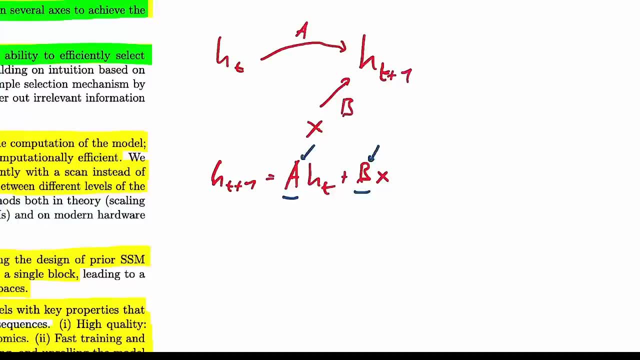 So, so it looks like a whole set of parameters, but in a very, very detailed way. 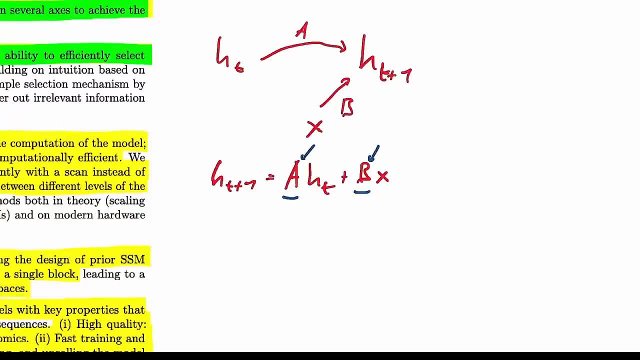 So we say a, B or of course, you use an initial variable. 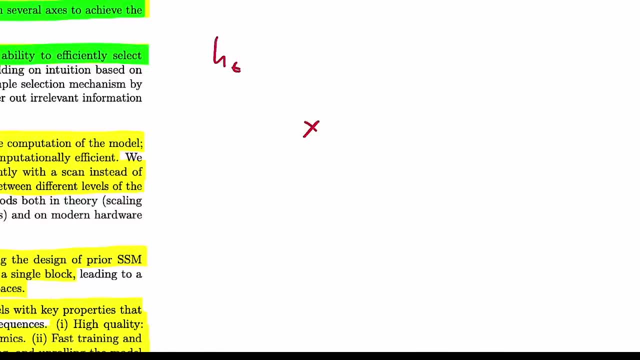 you have a previous hidden state, you have a current input and you want to build the next hidden state, t plus one. what structured state space models do is they have? they'll have some kind of parameterized function- let's call that a- and they'll have some sort of- uh, they'll have. 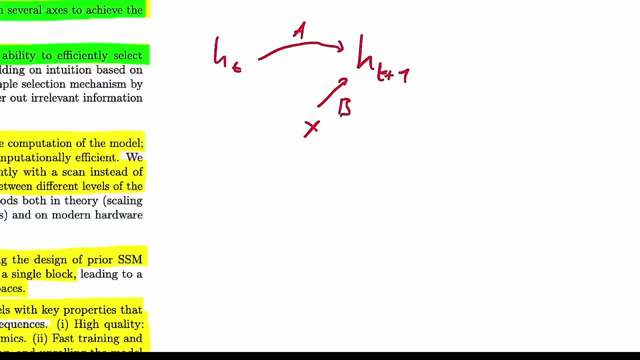 some sort here. let's call that b, even though, like it's, it's slightly different, but and the. the result is going to be that ht plus 1 is going to be equal to something like a ht plus b x. okay, again, not exact representation, but in principle this- and this is in ssms like- is going to be completely. 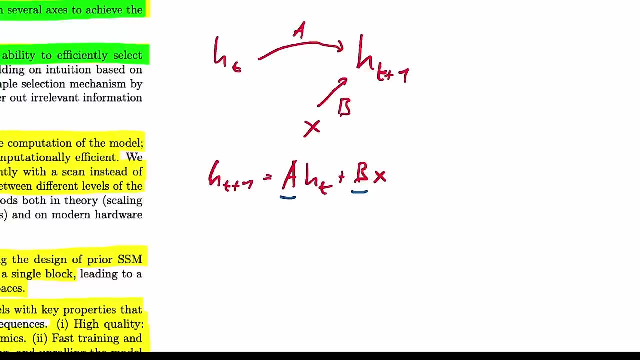 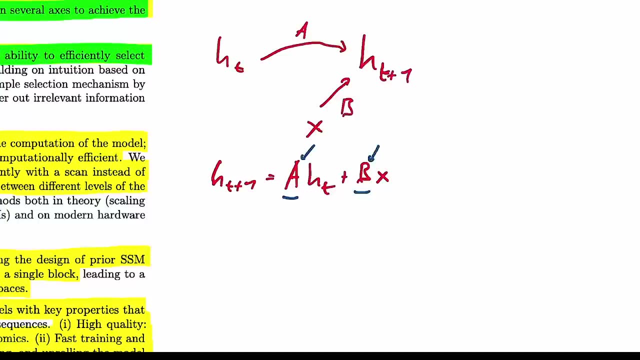 fixed for the whole sequence always. so you learn one set of parameters for you know, one a and one b for the entire model. okay, now this obviously is very, very different from transformers where a, like the attention matrix, is built dynamically at each single forward pass, you know, for each single. 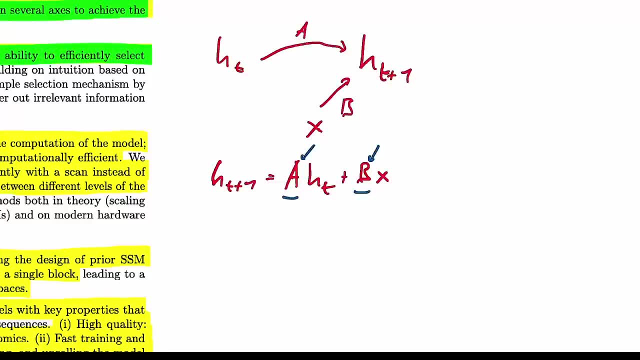 uh, for each single token, you compute queries and keys and values and therefore the aggregation. how you build the next hidden state is very dependent on on everything, on the input, on the past and so on. in this particular case, super fixed, you can see this is even more restrictive. 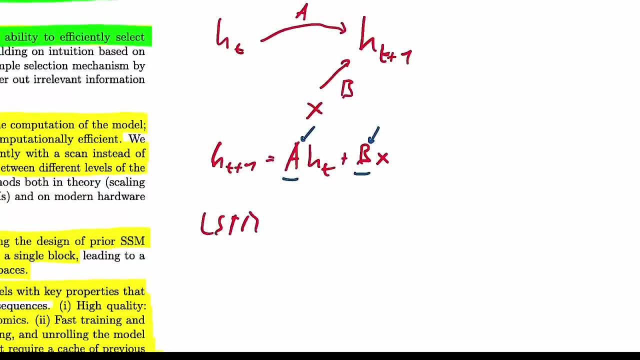 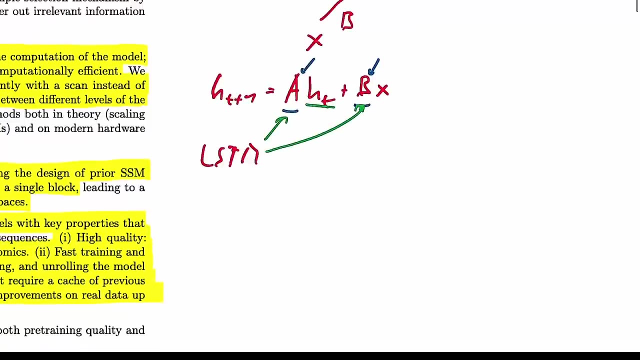 than something like an lstm. like in something like an lstm, as we discussed before, what you can do is you can make this and this actually dependent on the last hidden state. so in an lstm, you'll see that the last hidden state will be transformed into, you know, blue, and then this gives you the a. 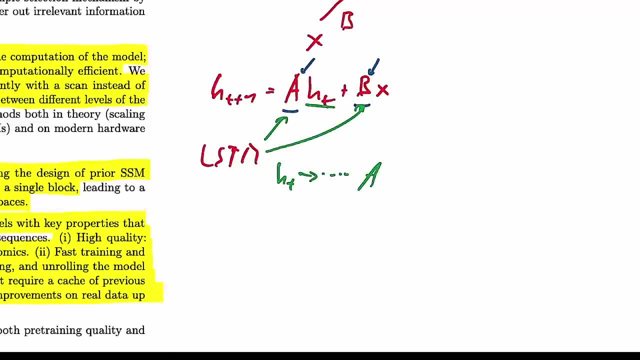 matrix, like in some sort of a gating way, and then x will be multiplied by by a and so on. so i don't have an lstm cell in my head, but in an lstm the propagation of the signals can be dependent on the previous hidden state and on the input. okay, 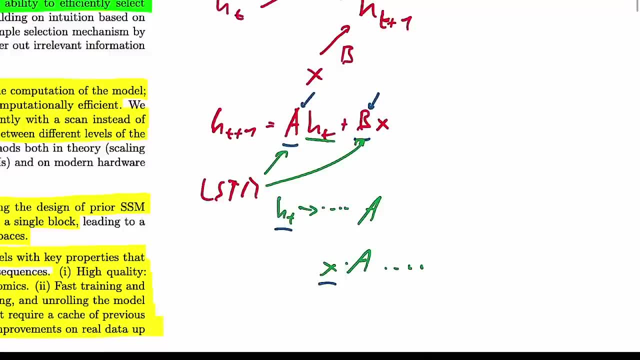 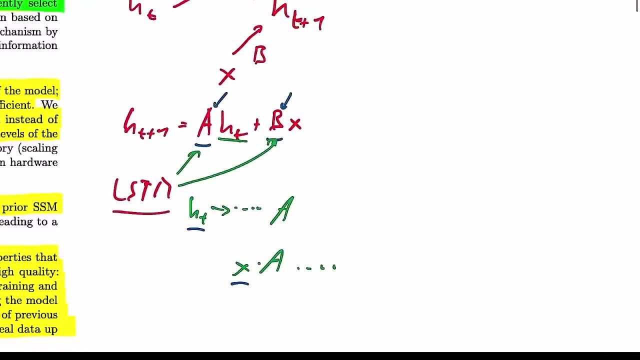 so that's the difference between the state space models and, like the, fully like general recurrent neural networks. what s what mamba is going to do? mamba is going to say: we allow the transition to be dependent on the current input, not on the previous hidden state, but on the current input. 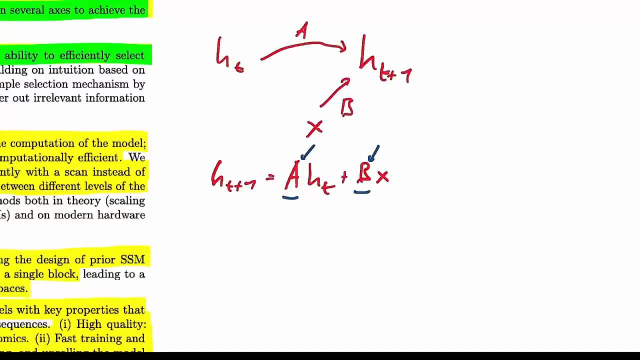 Okay. Now this obviously is very, very different from transformers where a like the attention matrix is built dynamically at each single forward pass. You know, for each single, uh, for each single token, you compute queries and keys and values, and therefore the 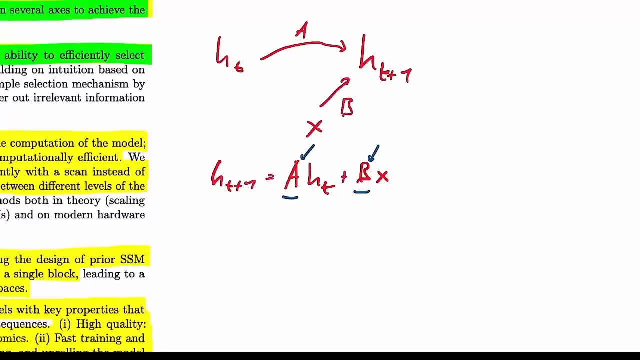 aggregation, how will you build the next hidden state? It's. Okay. Yeah. 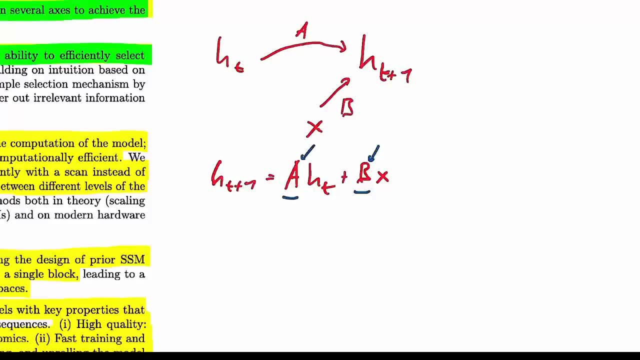 Very, yeah. case super fixed you can see this is even more restrictive than something like an LSTM like in 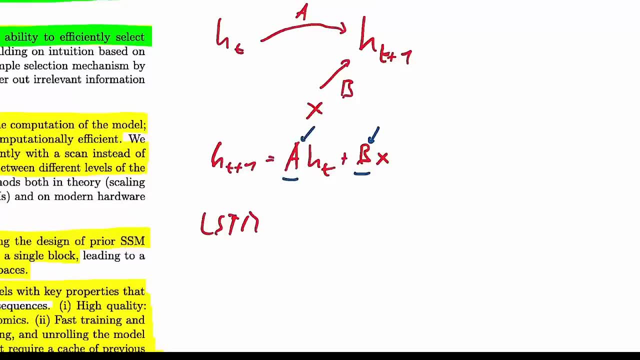 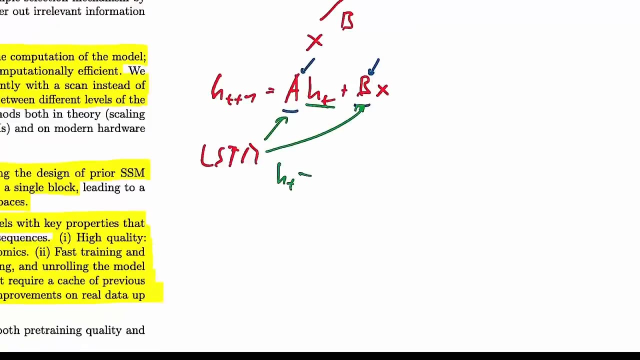 something like an LSTM as we discussed before what you can do is you can make this and this actually dependent on the last hidden state so in an LSTM you'll see that the last hidden state will be transformed into you know blue and then this gives you the a matrix like in a in some sort of a gating way and then x will be multiplied by by a and so on so I don't have an LSTM cell in my head but in an LSTM the propagation of the signals can be dependent on the previous hidden state and 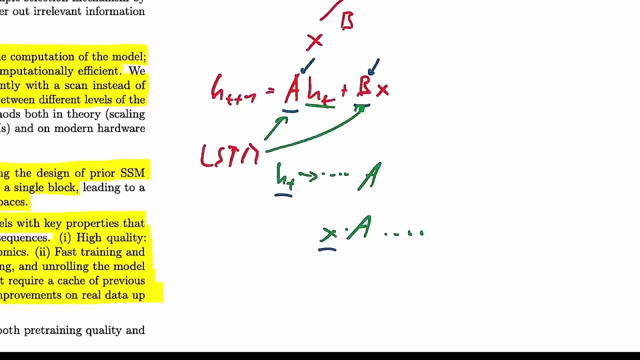 on the input okay and and that's the difference 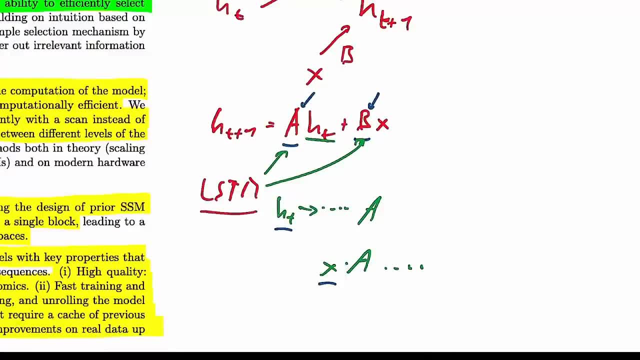 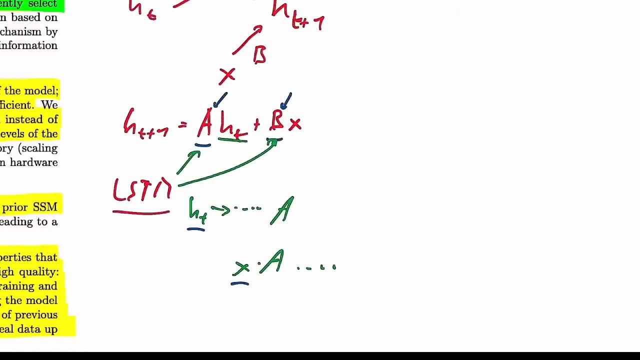 between the state space models and like the fully like general recurrent neural networks what as what mamba is going to do mamba is going to say we allow the transition to be dependent on the current input not on the previous hidden state but on the current input and you should already be able to see if you do that it still means that sort of this backbone going from hidden going from hidden state to next hidden state is going to be a fixed computation given by this a matrix and that's 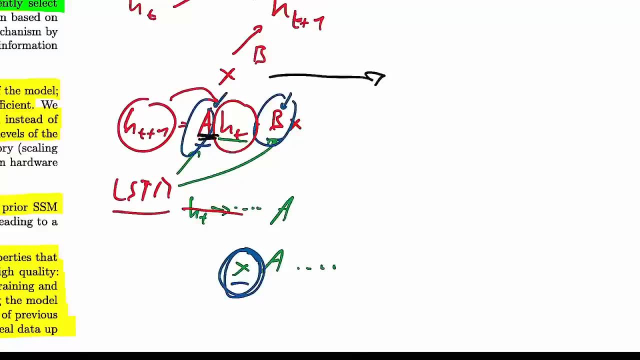 why we can sort of pre-compute it throughout all of time because that a is going to be fixed and not dependent on the input although what we'll see is that in fact how the how the input is 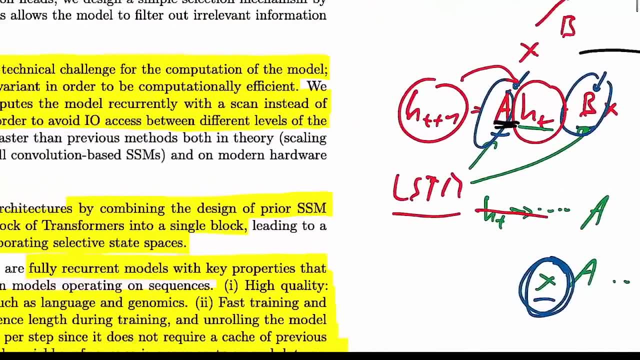 computed into and in the next hidden state is going to be influenced by the by the input and 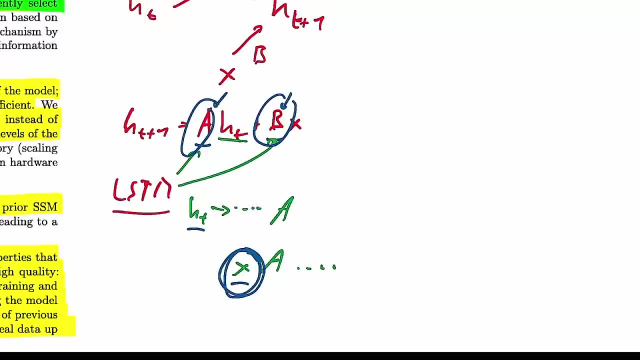 and you should already be able to see. if you do that, it still means that sort of this backbone of the current input is going to be the same as the previous one, so you can see that the next hidden state is going to be a fixed computation given by this, a matrix, and that's why we can sort of 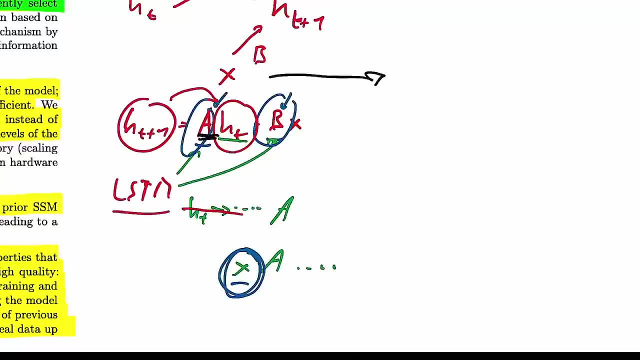 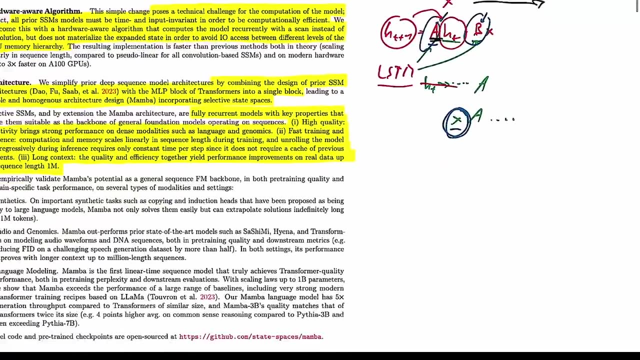 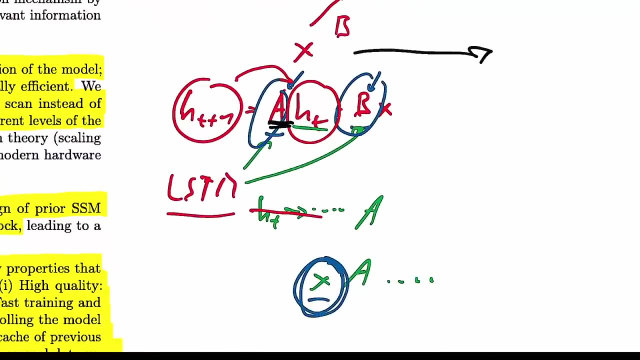 pre-compute it throughout all of time, because that a is going to be fixed and not dependent on the input, although what we'll see is that, in fact, how the- how the input is computed into and in the next hidden state- is going to be um influenced by the next hidden state. 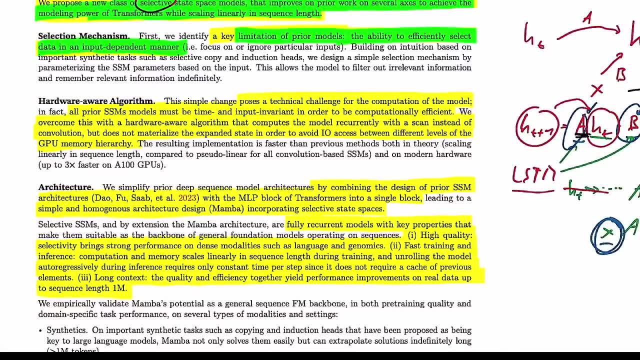 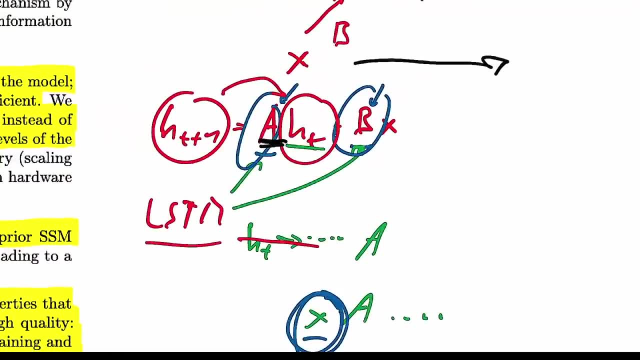 by the input, but not by the previous hidden state. okay, so i hope i've made this clear. a is going to be dependent on the input, b is going to be dependent on the input, but they're not going to be dependent on the last hidden state or any thing of the past. 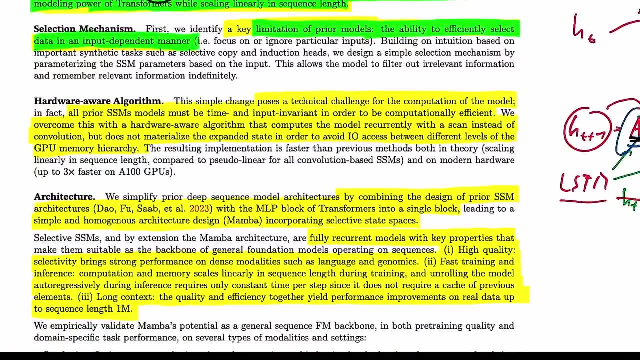 so it's kind of a trade-off between the state space models of the past and neural networks. um yeah, so they say: okay, this poses a challenge for the computation of the model. all prior, sorry, all prior- ssm models must be time and input invariant in order to 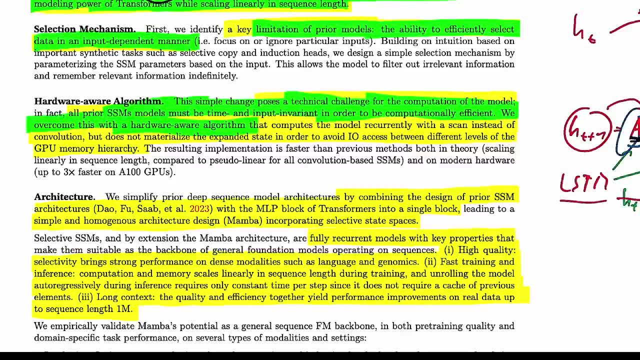 be computationally efficient. we overcome this with a hardware aware algorithm that computes the model recurrently, with a scan instead of a convolution. so they say essentially we sort of make it really fast on gpu, even though we have an algorithm, rhythmically a different, we have a different algorithm. we need to compute something. 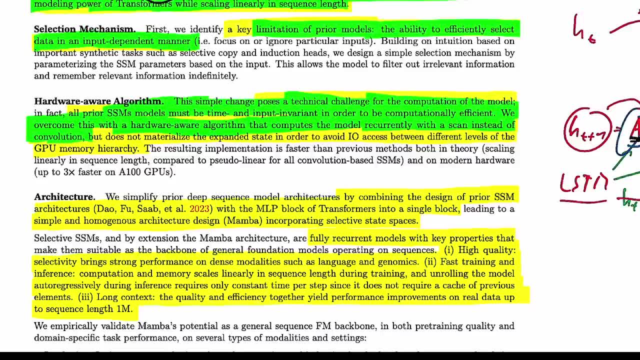 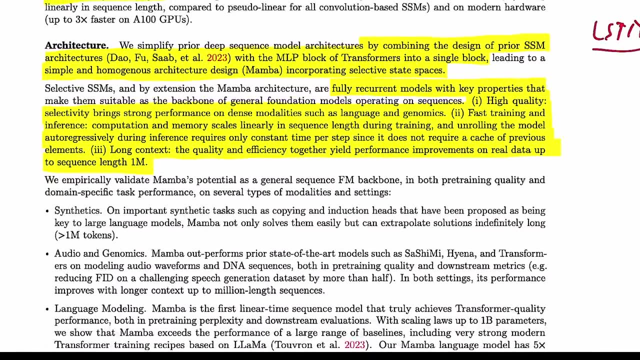 making the actual recurrence, or actually recurrently, but we do it in a way that fits really well onto gpus and therefore, uh, it's actually in in the end, it's actually faster. and, yeah, they make this into a model um called mamba. mamba is, mamba is not the same. 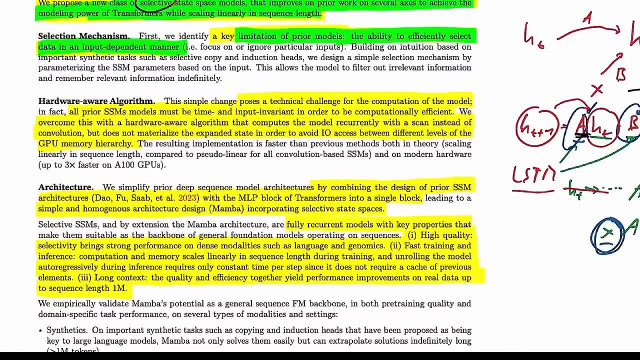 that's why it eles are so recurrent neural networks okay so we that's why the history of like here 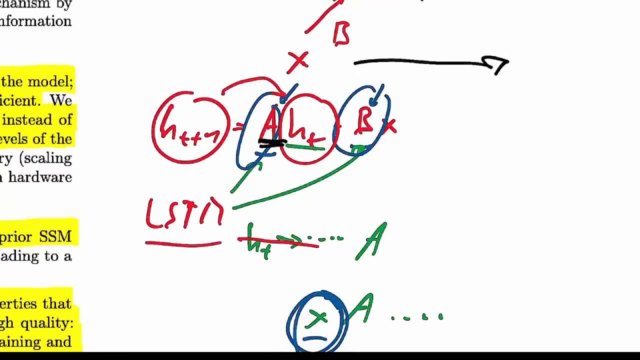 and so we have something more important now than before right after we have一个 in which we have 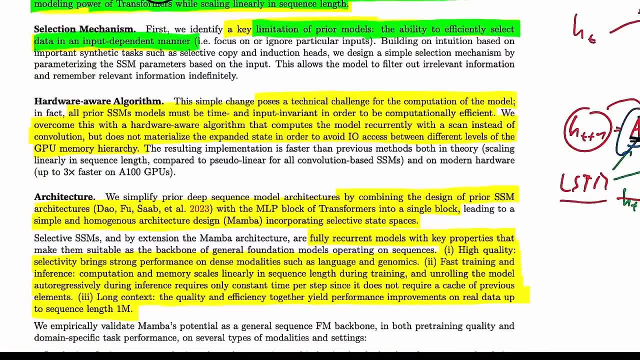 one end which means we will actually be able to see exactly what the choice that the remainder will be 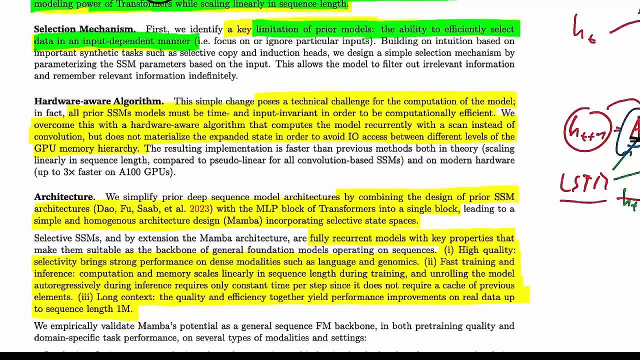 and so so a question is what's going to be and first then this next the last such step is that what we would have because this willNEY3A712枚 know and most of it and that's what you'reид postponed but not by the previous hidden state okay so I hope I've made this clear a is going to be dependent on the input b is going to be dependent on the input but they'rre not going to be dependant on the previous hidden state and anything of the past so it's kind of a tradeoff between the state space models of the past and recurrent neural networks 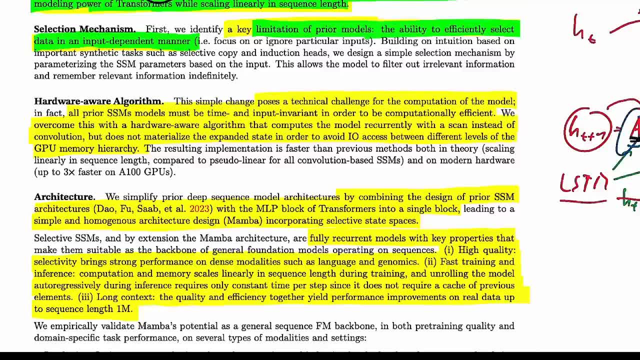 for Weise of the recurrent neural networks Um, yeah, so they say, okay, this poses a challenge for the computation of the model. 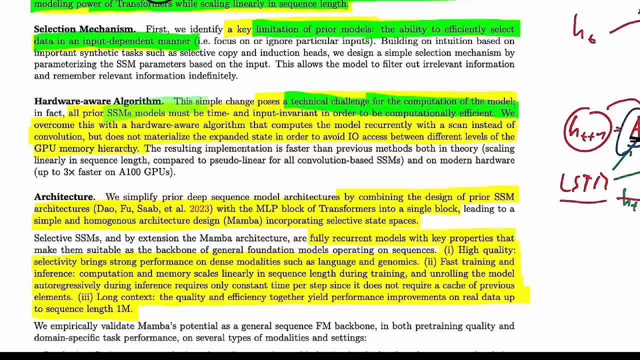 All prior, sorry, all prior SSM models must be time and input invariant in order to be computationally efficient. 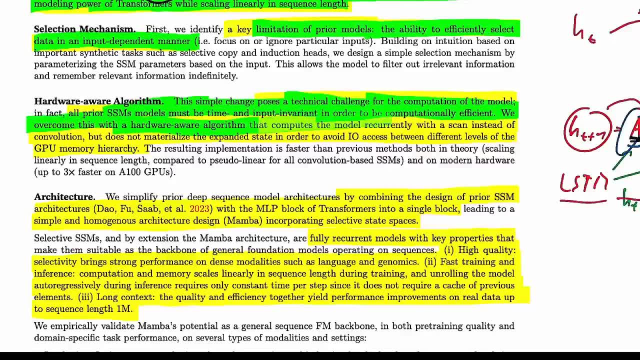 We overcome this with a hardware aware algorithm that computes the model recurrently with a scan instead of a convolution. 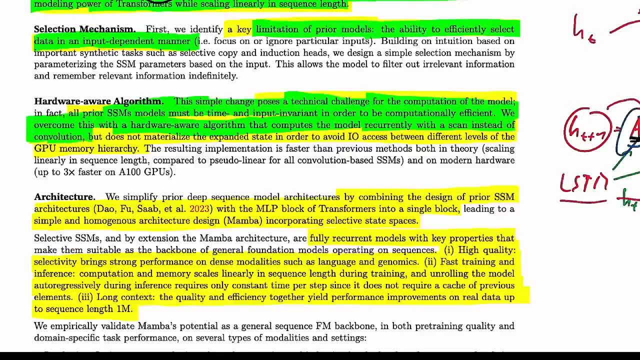 So they say, essentially, we sort of make it really fast on GPU, even though we have an algorithmically, a different, we have a different algorithm, we need to compute 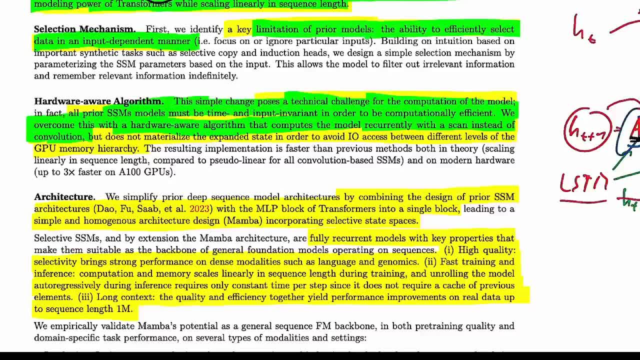 something, making the actual recurrence, or actually recurrently, but we do it in a way that fits really well on two GPUs. 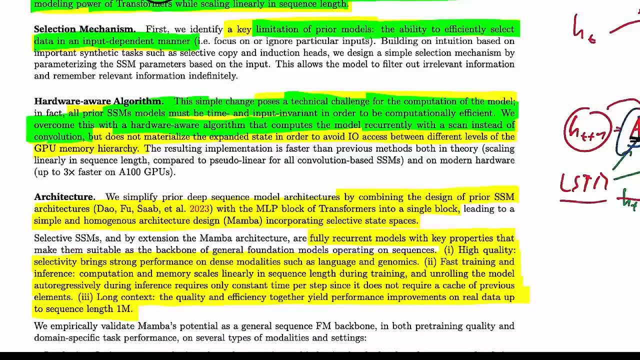 And therefore, it's actually in the end, it's actually faster. 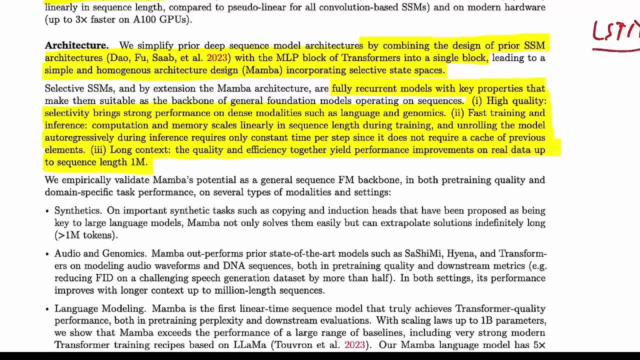 And yeah, they make this into a model called Mamba. Mamba is, Mamba is not the same as Select. 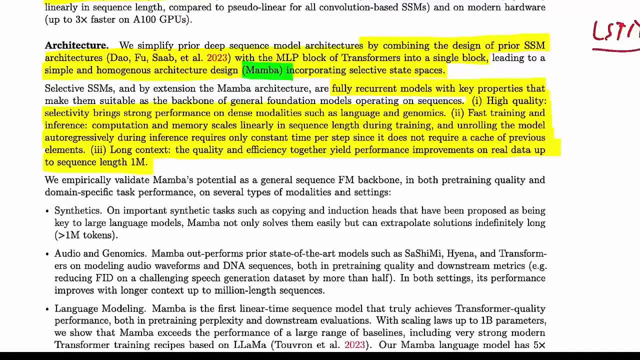 Selective state spaces, selective state space, uh, are a part of Mamba, uh, and then combined with some other stuff like, uh, 1D convolutions and up projections and gating that becomes the Mamba architecture. 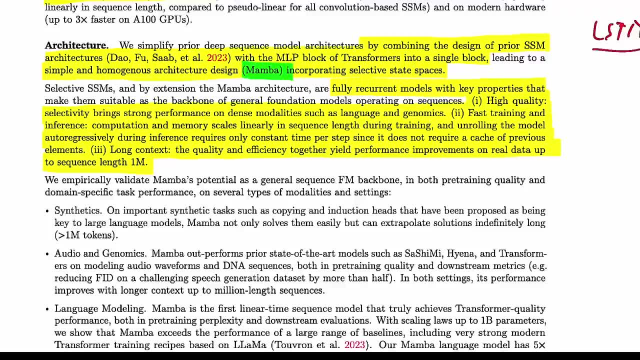 as selective state spaces. selective state space, uh, are a part of mamba and then, combined with some other stuff, like 1d convolutions and up projections and gating, that becomes the mamba architecture. it's attention free, uh. therefore it's. it avoids the quadratic bottlenecks. It's attention free. 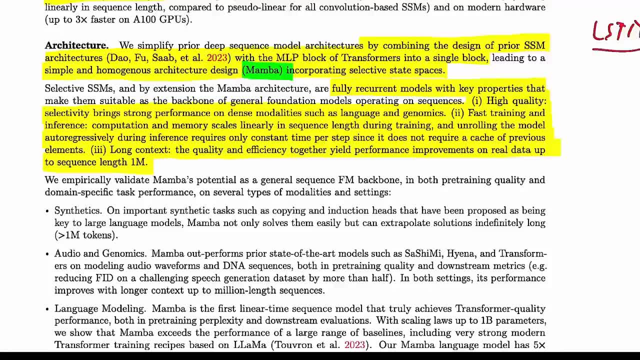 Uh, therefore it's, it avoids the quadratic bottlenecks of attention, of attention based models, such as transformers. So they say... 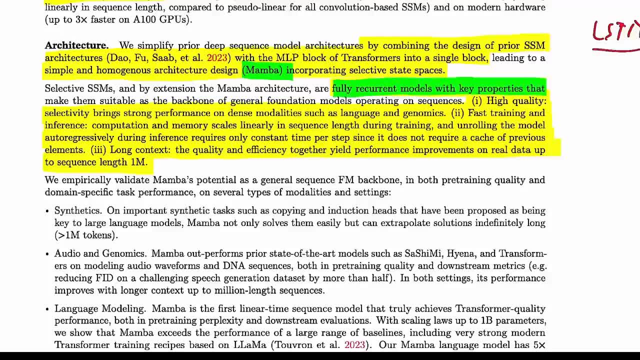 These are fully recurrent models with the key property, uh, for example, high quality. Selectivity brings strong performance on dense modalities, such as language and genomics. 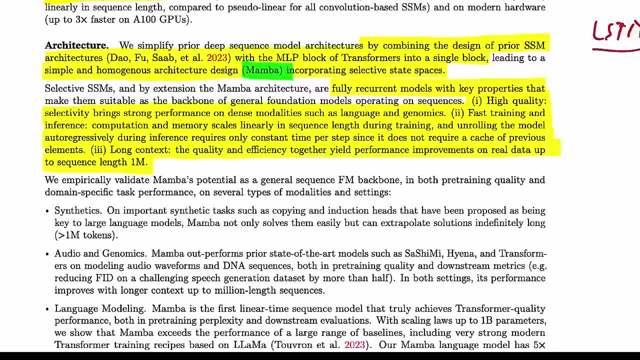 of attention, of attention-based models such as transformers. so they say these are fully recurrent models with the key property uh. for example, high quality selectivity brings strong performance, and that on dense modalities such as language and genomics. i think that's going to be the biggest sticking points. so they have recognized that. you know this. 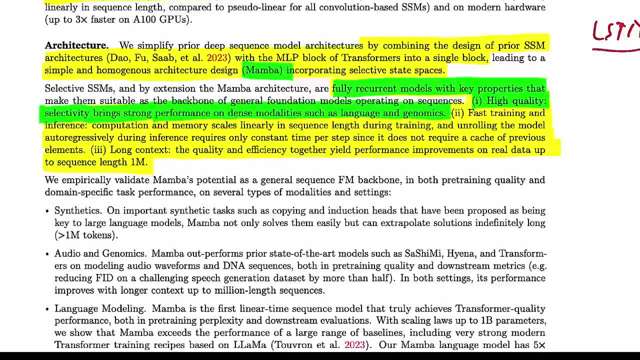 super scalable thing like s4 is not really suitable for language because you need to be a little bit data dependent in your transitions from you know through the hidden states. and now they say, well, selectivity brings strong performance, which, because they added selectivity, they added this dependence on the input of the transition- now gives them a bump in performance. 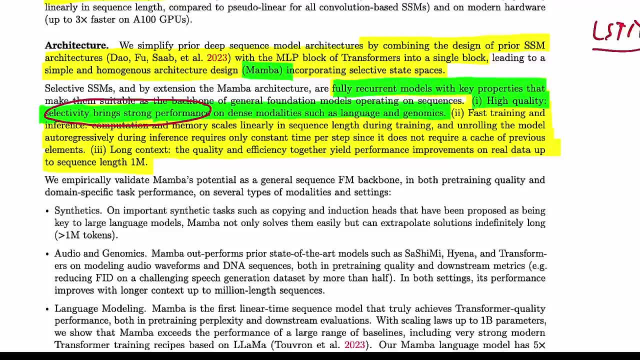 the jury is still out whether in the future they'll say, yeah, it's better, but still, in order to really reach the performance of transformers, we also need to make that transition actually dependent on the hidden states and at that point early in one dimension, and so we're trying to knock them back to essentially lstms. 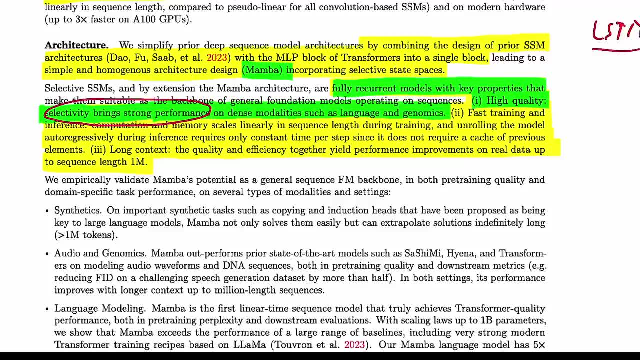 but it could be that the dependence on the input- just the input- already makes them as strong as transformers on a lot of important benchmarks. fast training and inference, computation and memory scales linearly in sequence length during training, and unrolling the model autoregressively during inference requires only constant time per step. 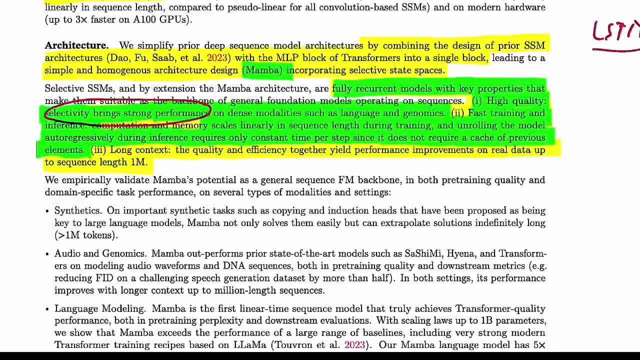 acquire a cache of previous elements. so there's no key value cache and so like. in transformers, you literally just have to remember the last hidden state, and then producing one additional token during inference is just, it's just two matrix multiplications or something like this, right, so no attention, no, no, nothing, just multiply it in and you have it. and long context: the quality. 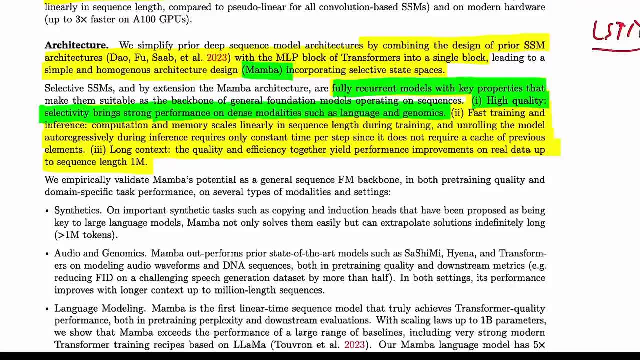 I think that's going to be the biggest sticking points. So they have recognized that, you know, this super scalable thing like S4 is not really suitable for language because you need to be a little bit data dependent in your transitions from, you know, through the hidden states. 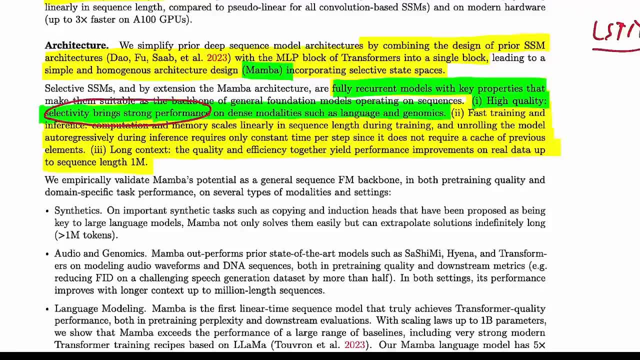 And now they say, well, selectivity brings strong performance, which, because they added selectivity, they added this dependence on the input of the transition, um, now gives them a bump in performance. 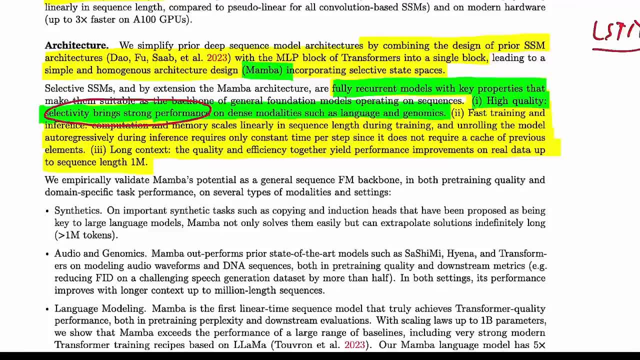 The jury is still out whether in the future they'll say, yeah, it's better, but still in order to really reach the performance of transformers, we also need to make that transition 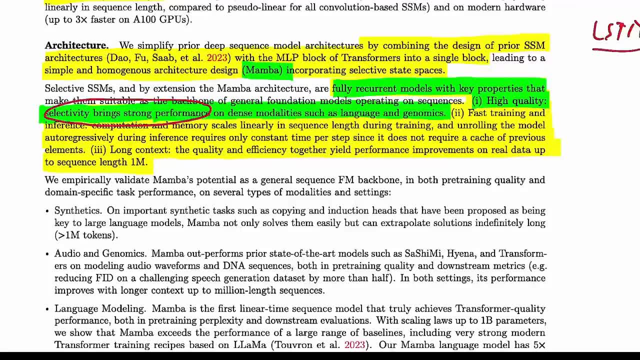 actually dependent on the hidden states. And at that point, we're back to... 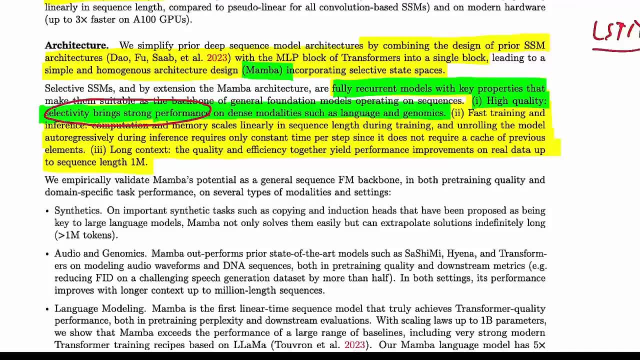 Essentially LSTMs, but it could be that the dependence on the input, just the input, um, already 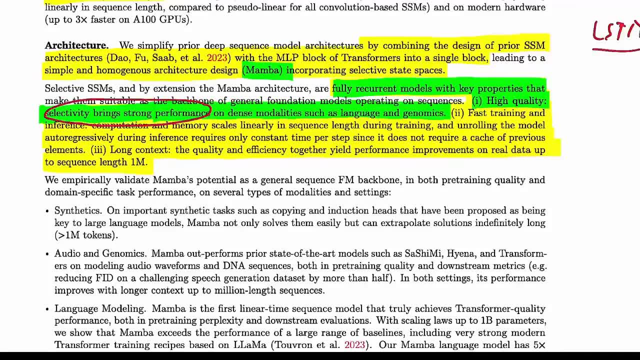 makes them as strong as transformers on a lot of important benchmarks, fast, fast training and inference, uh, computation memory scales linearly in sequence length during training and unrolling the model autoregressively during inference requires only constant time per step, since it does not require a cache of previous elements. 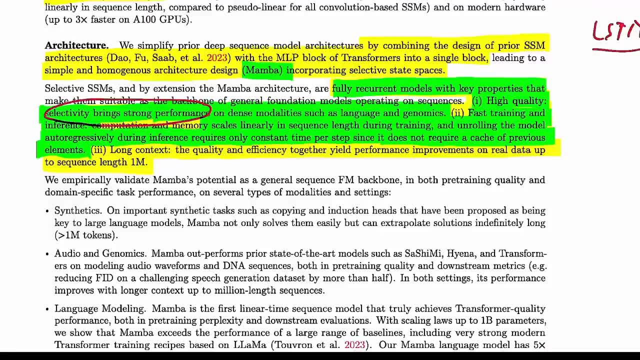 So there's no key value cache. And so like in transformers, you literally just have to remember the last hidden state and then producing one 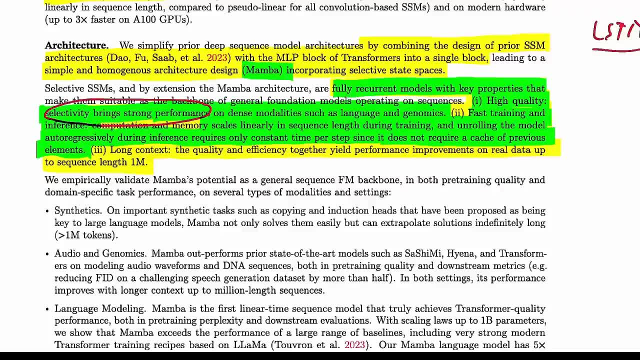 additional token during inference is just, it's just two matrix multiplications or something like this, right? So no attention, no, no, nothing. Just multiply it in and you have it. 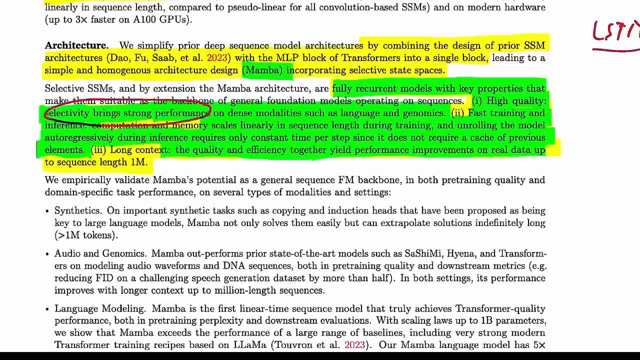 And long context, the quality and efficiency together yield the performance improvements on real data up to sequence length on million. 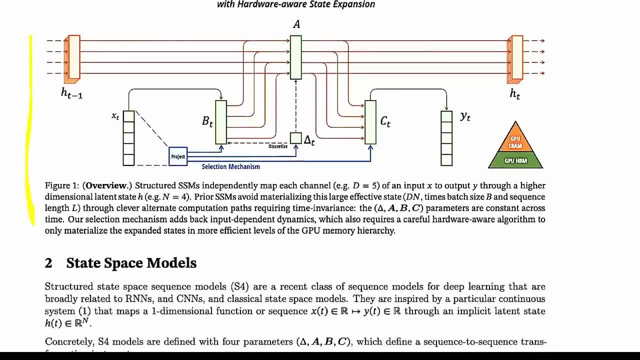 All right. So this is the, the, the architecture is a bit distributed throughout the paper. 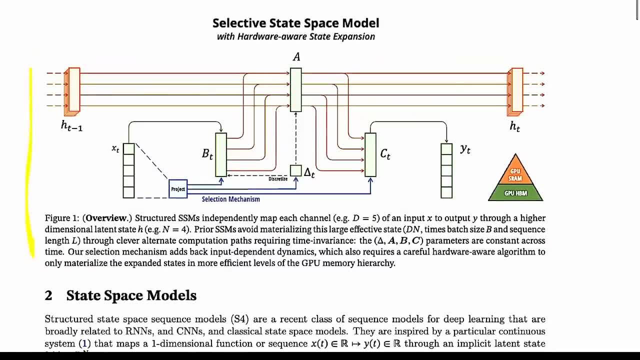 This is the selective state space, um, part of this. There's going to be a more extensive thing here. 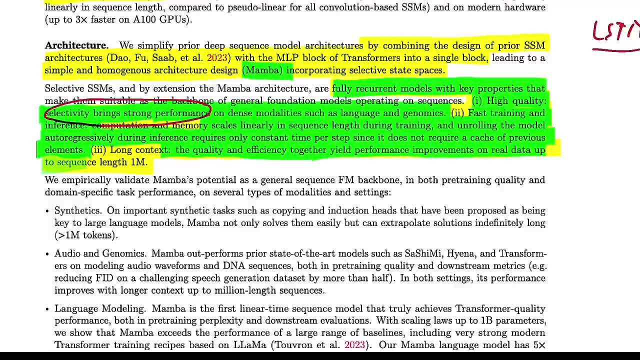 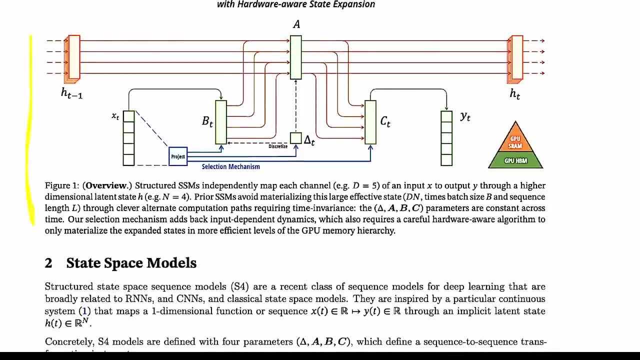 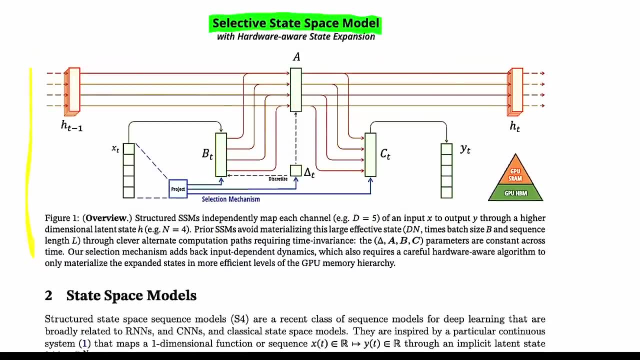 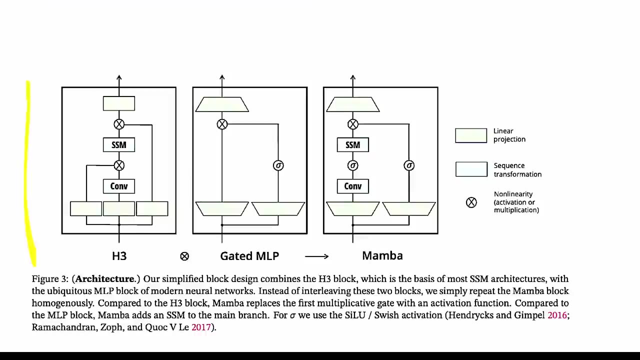 and efficiency together yield the performance improvements on real data up to sequence length on million. all right, so this is the. the architecture is a bit distributed throughout the paper. this is the selective state space, um part of this. there's going to be a more extensive thing here, um. so the mumba architecture consists of the part i've just shown you. 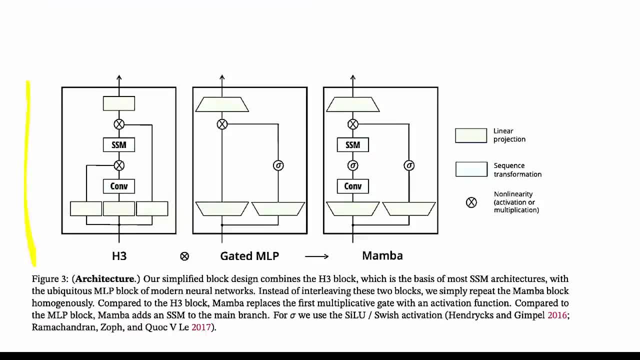 Um, so the Mamba architecture consists of the part I've just shown you, but also of other things. So you have to imagine these things are going to be layered on top of one another. And. And then, um, essentially you'll, you'll always consider the entire sequence as one during training. 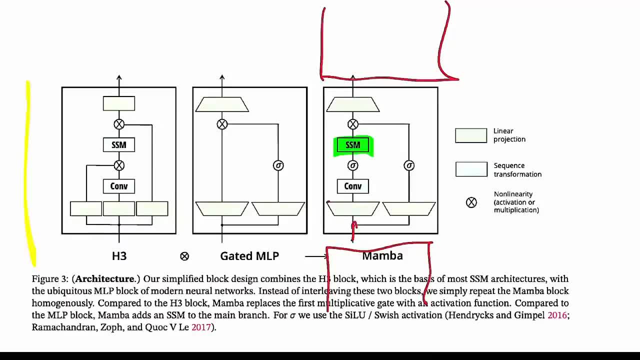 Um, so if we go in here, uh, this here, for example, this is a linear projection. So you project up in dimensions and you project each token individually, like in a transformer, then you do a one D convolution. There is some non-linearity in there. 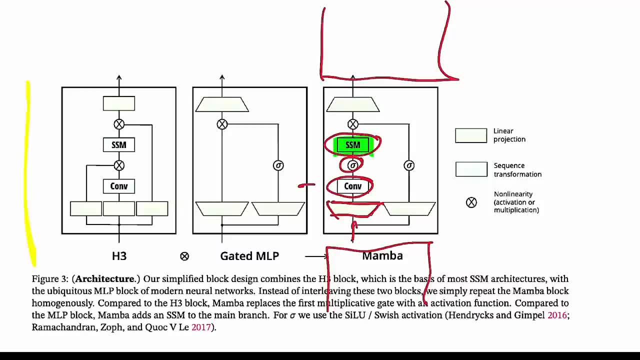 Then comes that, uh, SSM now in these two things, you want to consider. The whole sequence as one during training, right? However, in the projections right here, they, as far as I understand, go just individually over tokens, like the MLPs in a transformer. And then there is also this extra mechanism right here, which is a gating mechanism. Like you're used to from, from other gated architectures. 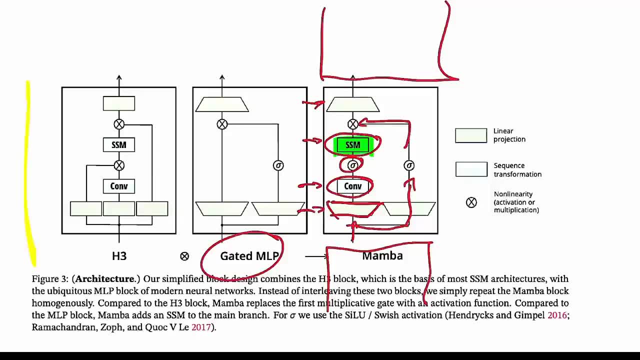 Again, this doesn't go between time steps. That's important to note. This goes from layer to layer, right? So as you go up the layers. 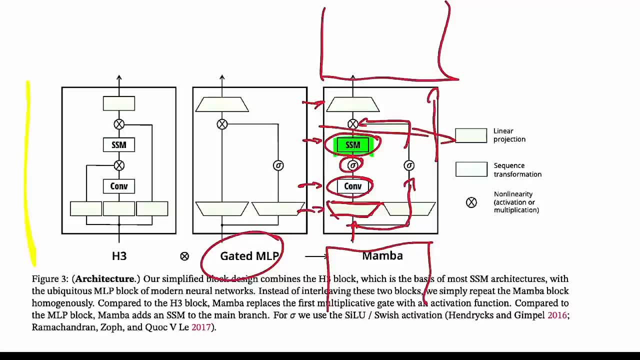 The time would be some sort of, the time steps aren't even shown here. There's no time direction in this particular diagram. 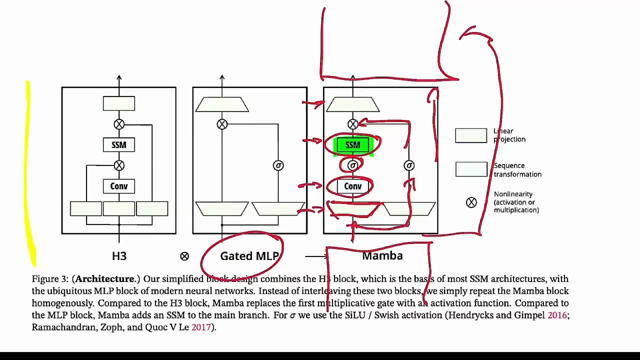 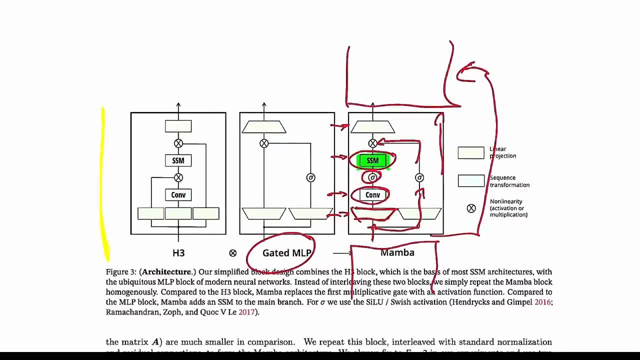 There is also residual connections like that go, uh, out, out the way and so on. Um, yeah, so the Mamba is an architecture that includes this new, uh, selective state spaces. 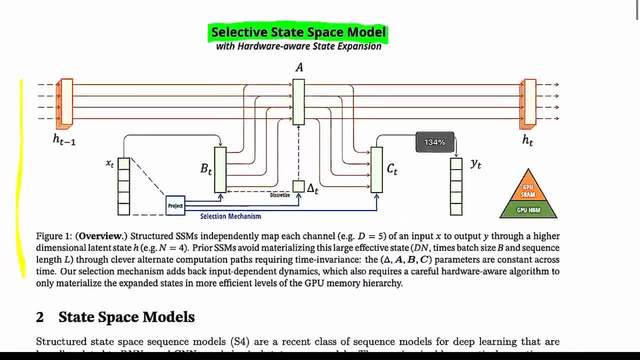 That selective state space layer looks about like this. And here we now have a time direction. 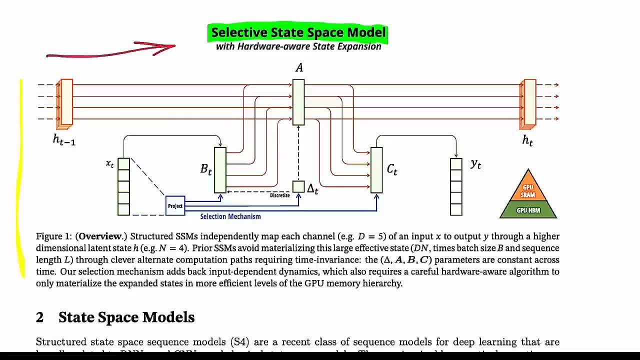 So here we now consider how do we compute, um, one token in this sequence, given that we have to accumulate this hidden state, uh, over time. 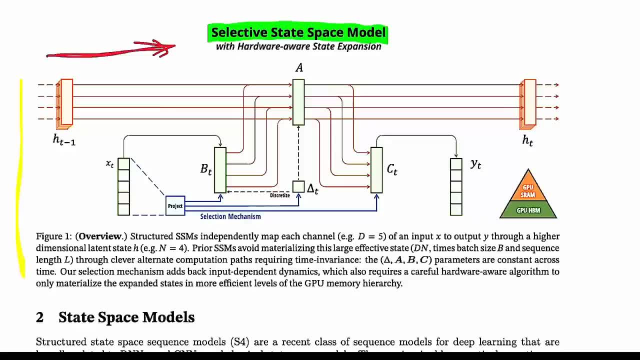 And again, we can do this either during training, where we try to compute all of them as fast as possible, or during inference where we just do one of these time steps. 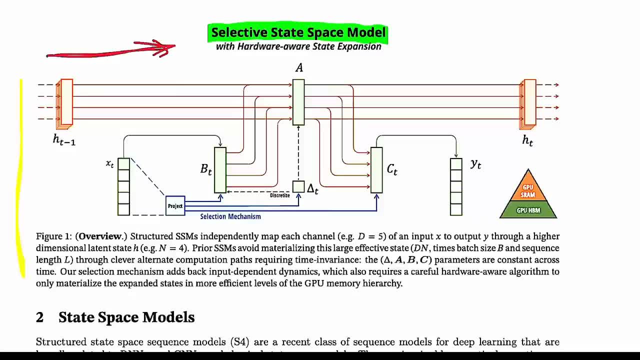 So as you can see, the backbone is just going to be, we have this, we multiply, we multiply. Essentially there is a. 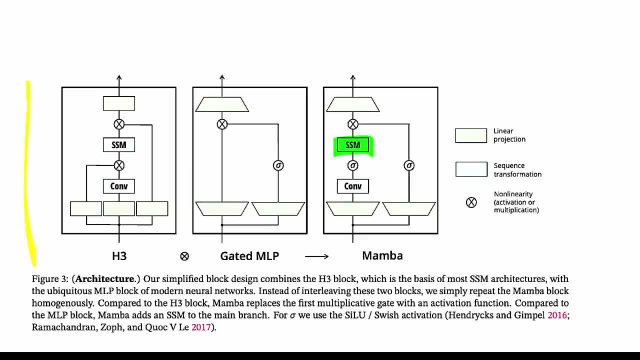 but also of other things. so you have to imagine these things are going to be layered on top of one another. so you have to imagine that the architecture is going to be layered on top of one another, and then, um, essentially you'll always consider the entire sequence as one during. 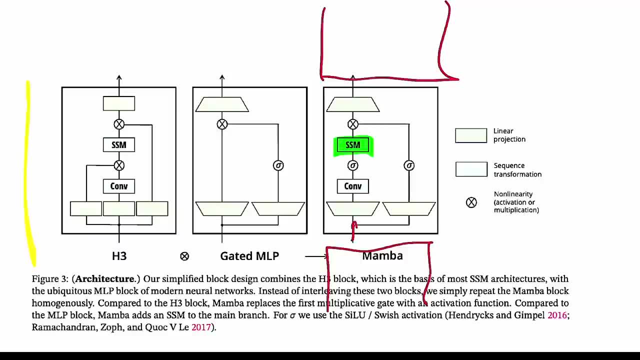 training. um, so if we go in here, uh, this here, for example, this is a linear projection, so you project up in dimensions and you project each token individually, like in a transformer. then you do a 1d convolution. there is some non-linearity in there. then comes that ssm. now, in these two things, 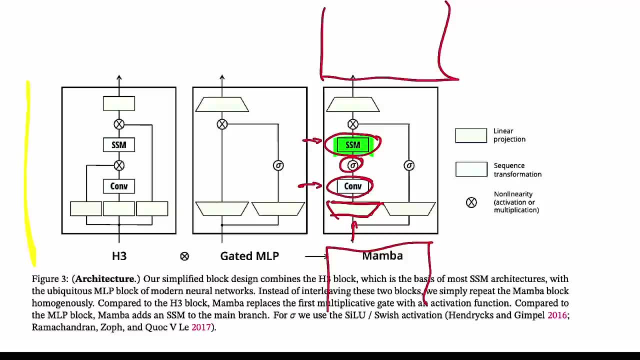 you want to consider the whole sequence as one during training, right. however, in the projections right here, they, as far as i understand, go just individually over tokens like the, the mlps, in a transformer, and then there is also this extra mechanism right here which is a gating mechanism. 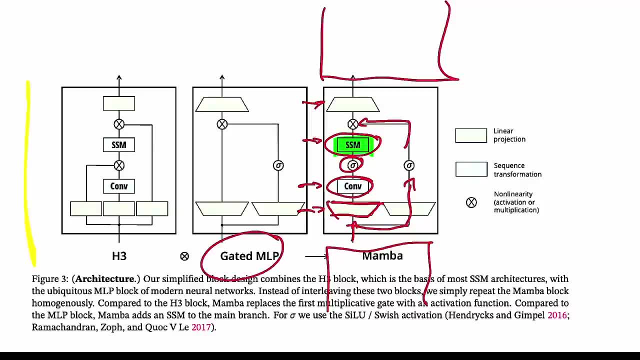 like you're used to, from from other gated architectures. again, this doesn't go between time steps. that's important to note. this goes from layer to layer, right? so you want to consider the whole sequence as one during training, right? however, in the projections, as you go up the layers, the time would be some sort of the time steps aren't even shown here. 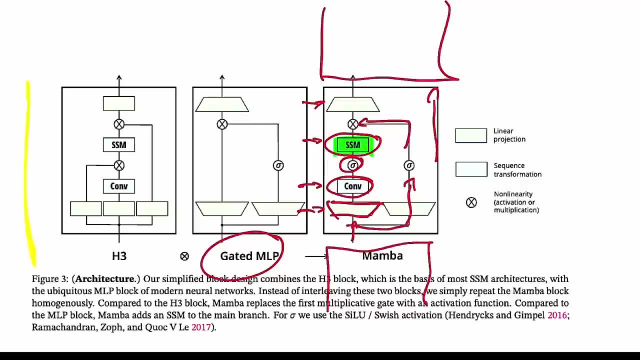 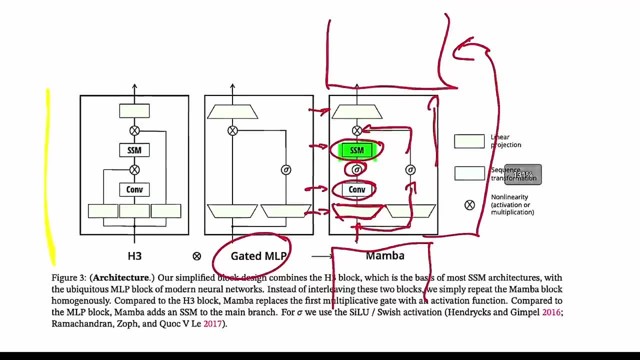 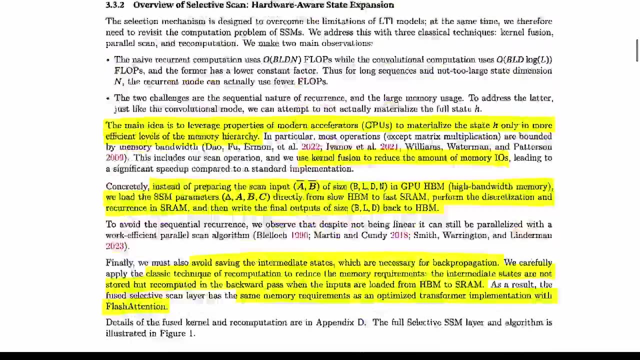 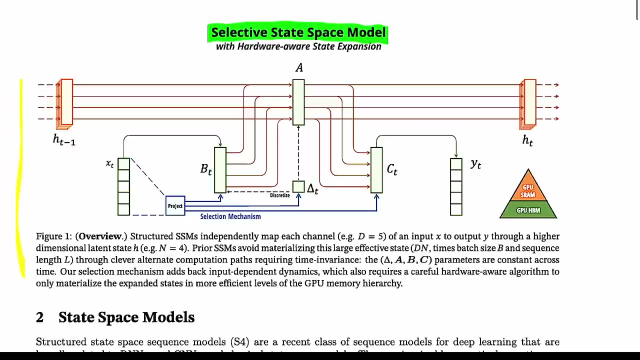 there's no time direction in this particular diagram. there is also residual connections like that go out out the way and so on. um yeah, so the mamba is an architecture that includes this new selective state spaces. that selective state space layer looks about like this: and here we. 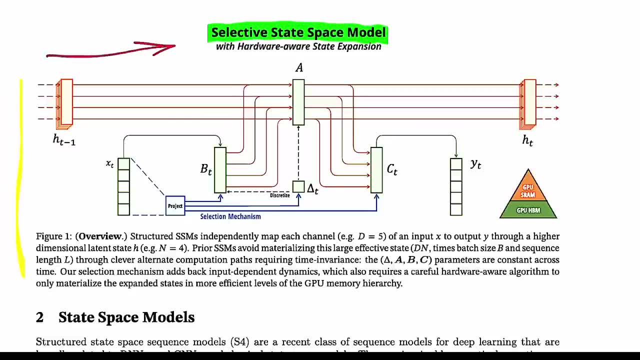 now have a time direction, right. so here we now consider: how do we compute um one token in this sequence, given that we have to accumulate this hidden state, uh, over time and again. we can do this either during training, where we try to compute all of them as fast as possible, or during 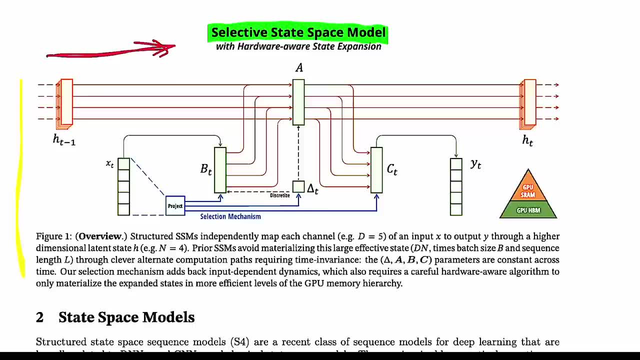 inference, where we just do one of these time steps. so, as you can see, the backbone is just going to be: we have this, we multiply, we multiply. essentially, we have this and then we have this, and then we have actually, there is a, there is a this, this, a matrix right here that we're going to use, and there is 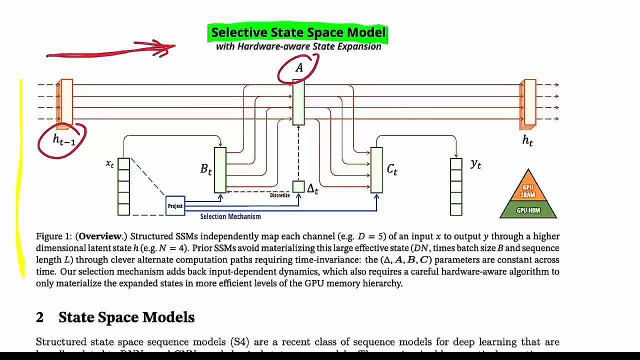 There is a, this, this a matrix right here that we're going to use, and there is the input that somehow comes in. And from these two things, we're going to produce that next hidden state. 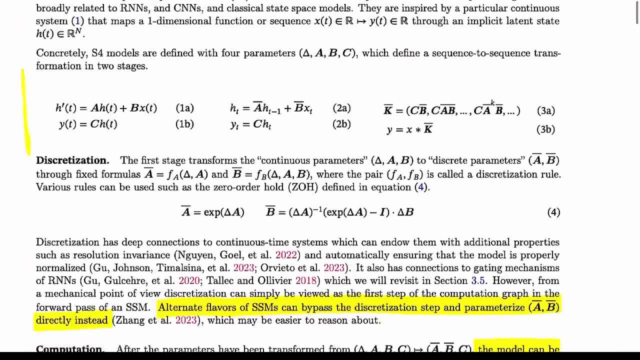 Now, what is all of this right here? Um, all of this is part of this, uh, state space architecture. How does that look? 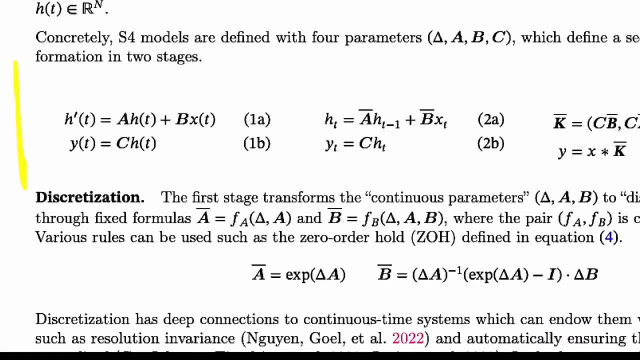 There is a technicality in here, which is called discretization. Now. The. The. 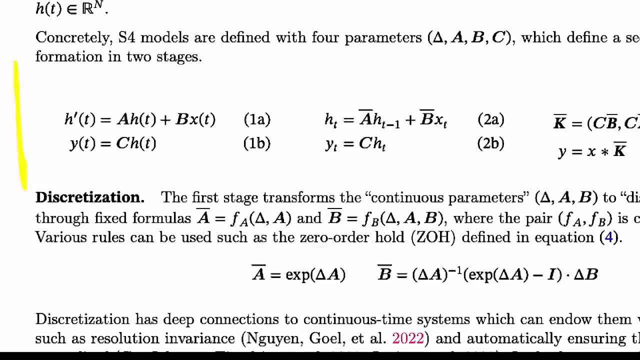 The theory behind state space models and, and so on is, uh, was developed for continuous time systems. 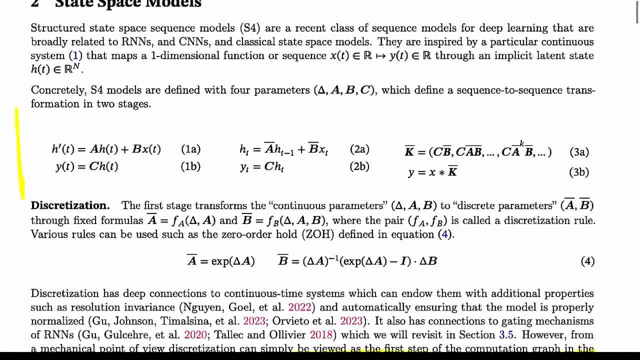 And if you want to make them into discrete, you, if you want to be sort of correct, you can't just, uh, you can't just apply the same thing. 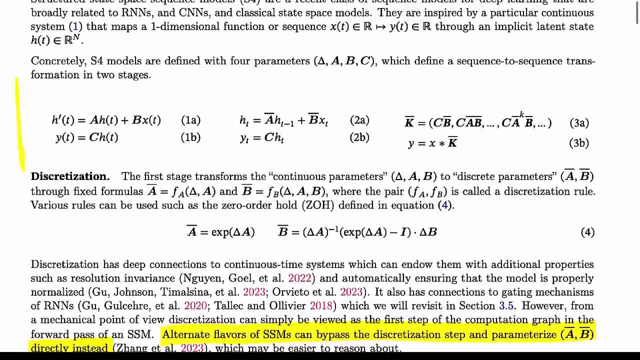 Um, if you do it in the way they do it here, it has some nice properties such as I, I believe your, your kind of time step in independent, uh, you automatically scale it. The, the things to the correct scaling and so on. 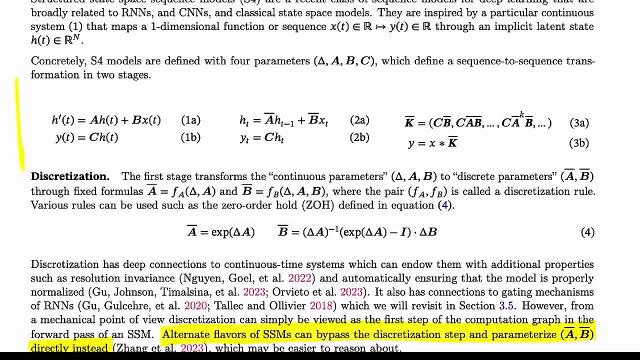 However, whenever you hear discretization, um, just you're free to also just kind of ignore it for the purposes of understanding what's going on from a deep learning perspective. 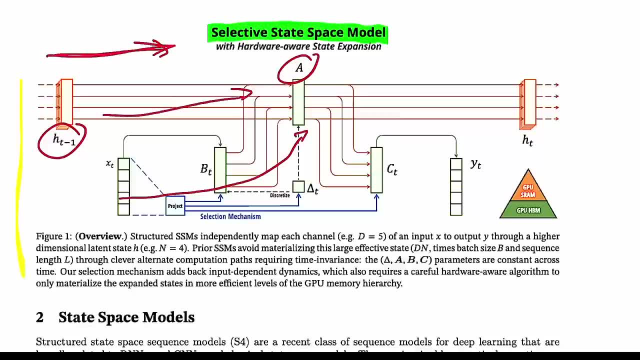 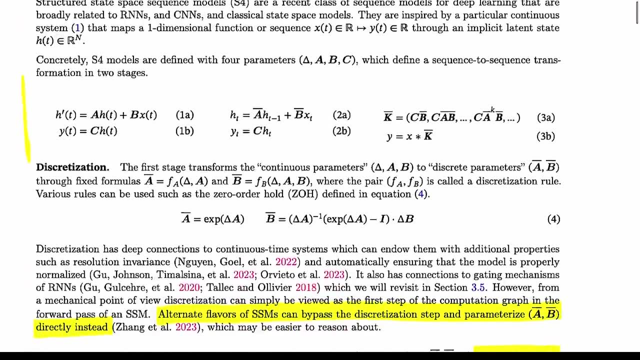 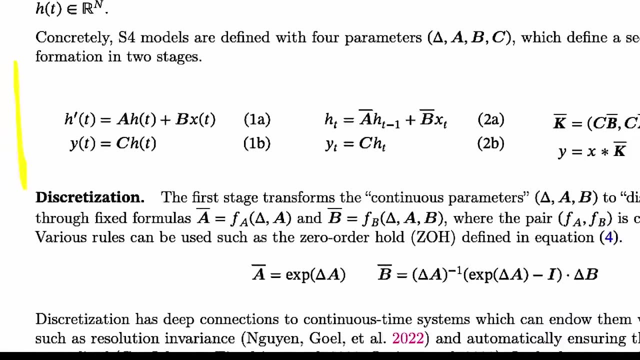 the input that somehow comes in, and from these two things we're going to produce that next hidden state. now, what is all of this right here? um, all of this is part of this state: space architecture. how does that look? there is a technicality in here, which is called discretization. now, 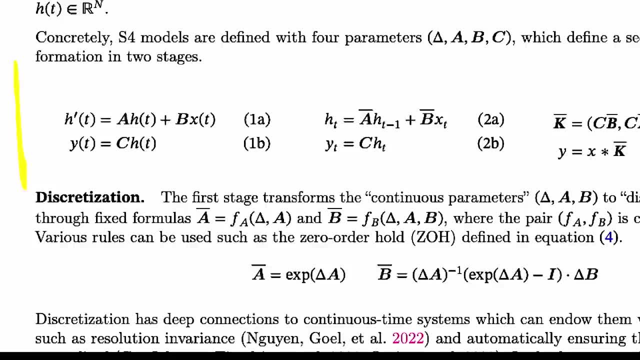 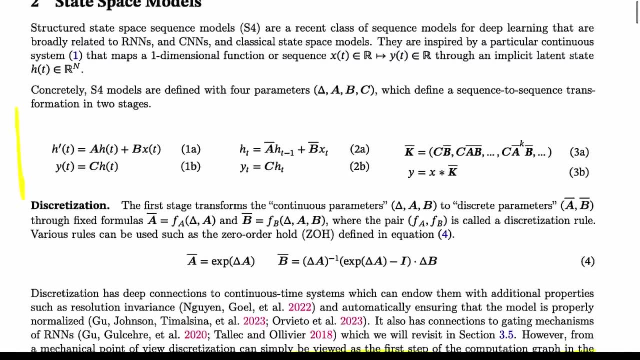 the, the theory behind state space models and and so on. is was developed for continuous time systems and if you want to make them into discrete, you, if you want to be sort of correct, you can't just, uh, you can't just apply the same thing. um, if you do it in the way they do it here, it has some nice. 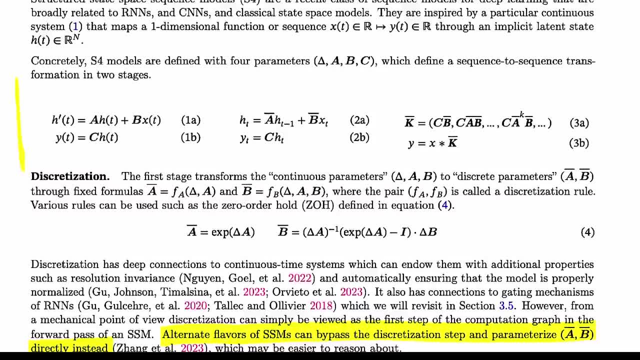 properties such as: i believe your your kind of time step in independent, uh, you automatically scale it, the things to the correct scaling, and so on. however, whenever you hear discretization, um, just you're free to also just kind of ignore it for the purposes of understanding what's going. 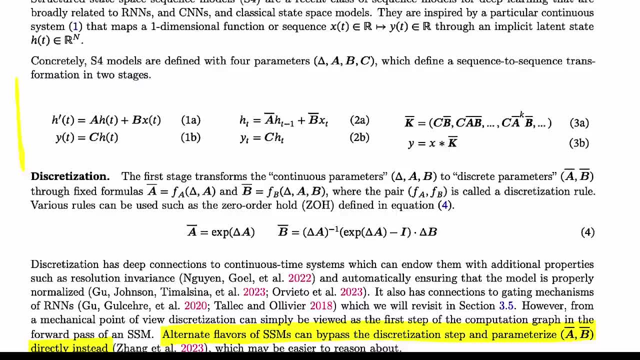 on from a deep learning perspective and from a data flow perspective. i'm sorry, albert, if you're listening, this must be really offensive. um, and i apologize for that, uh, um, we can do another video where we dive into sort of into more of the background behind these models and so on. i'm maybe 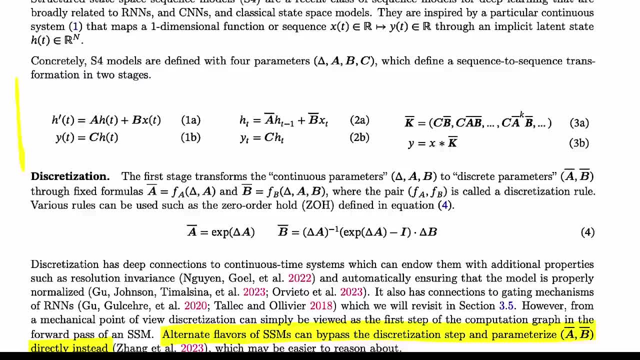 not the best person to explain that, but we'll do our best to understand, kind of, what's going on here on a more high level. so you have- they call them- four parameters. okay, these are. these are matrices or vectors that just have learnable parameters. you'll use this. this here is the sort of like a. 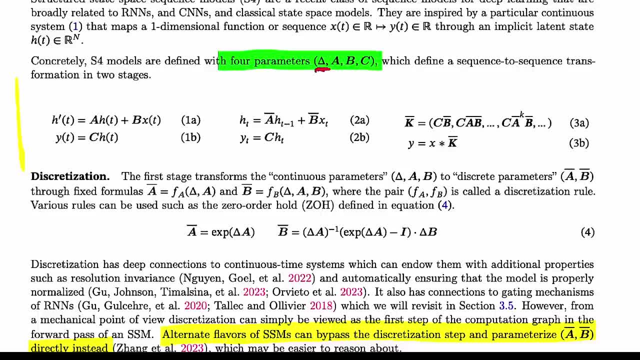 parameterization. parameterization- no sorry, discretization parameters. this here controls how one hidden state is propagated forward. this here controls how much of the input is propagated into the new hidden state, and this here controls how the hidden state is is processed into the output state. so you can see: 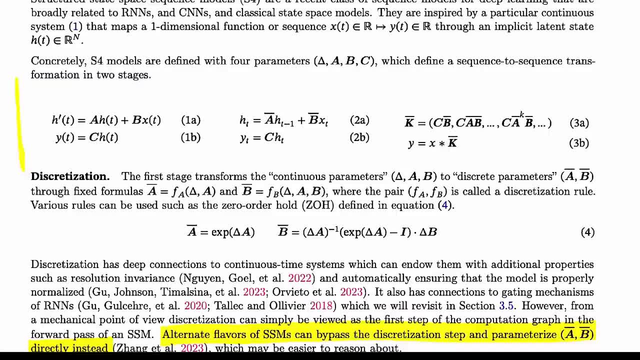 And from a data flow perspective, I'm sorry, Albert, if you're listening, this must be really offensive. Um, and I apologize for that. Uh, I'm we can do another video. Yeah. 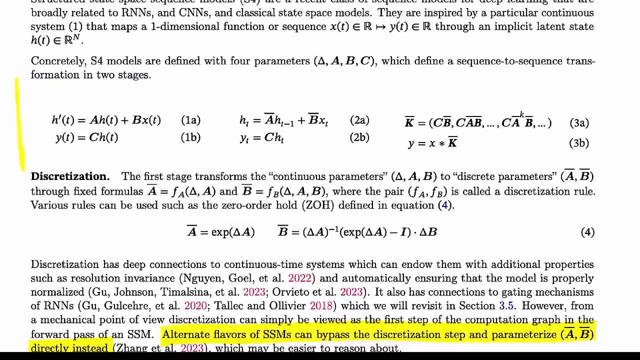 dive into sort of into more of the background behind these models and so on i'm maybe not the 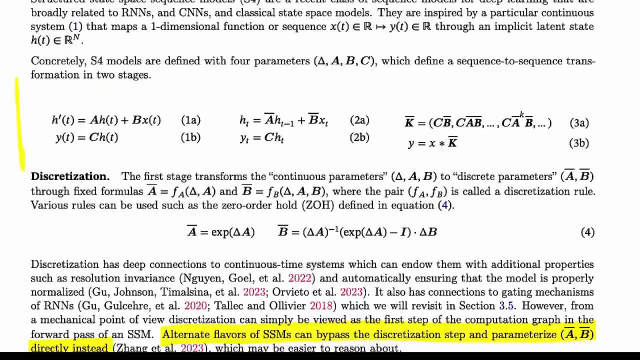 best person to explain that but we'll do our best to understand kind of what's going on here on a more high level so you have they call them four parameters okay these are these are matrices or 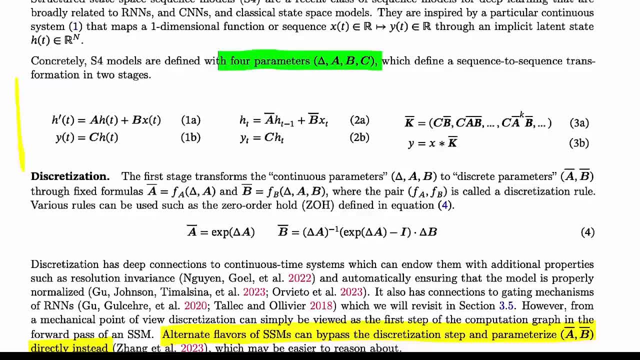 vectors that just have learnable parameters you'll use this this here is the sort of like parameterization parameterization no sorry discretization parameters this here controls 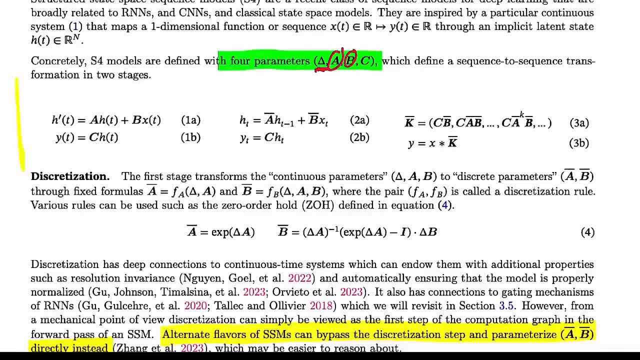 how one hidden state is propagated forward this here controls how much of the input is propagated into the new hidden state and this here controls how the hidden state is is processed into the 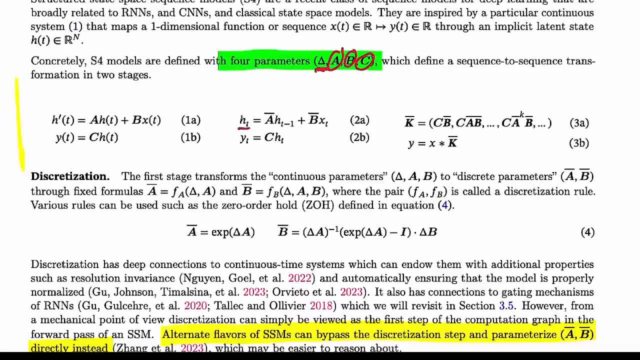 output state so you can see the next hidden state is produced from the last hidden state multiplied by what's called the 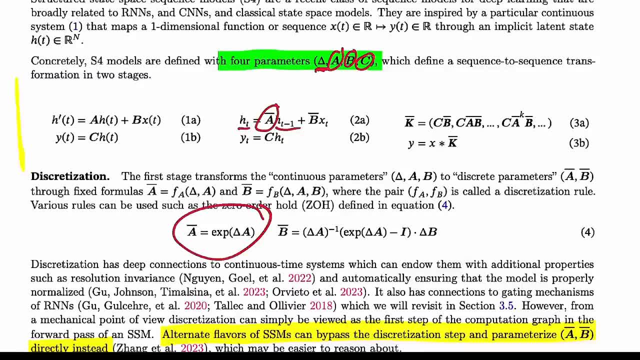 a bar and a bar is simply a computation that results from this discretization parameter and the a matrix again don't worry just consider if you want just consider this here to be a 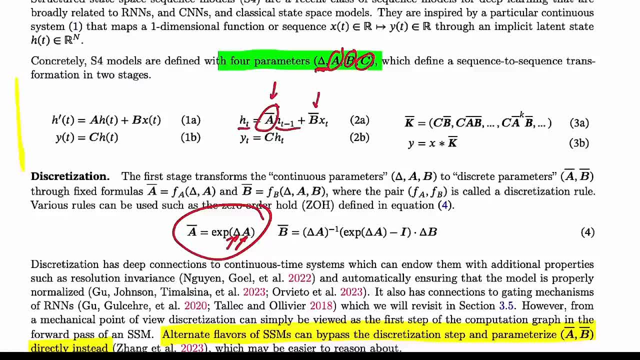 learnable matrix and this here to be a learnable matrix and in that you can see from this perspective 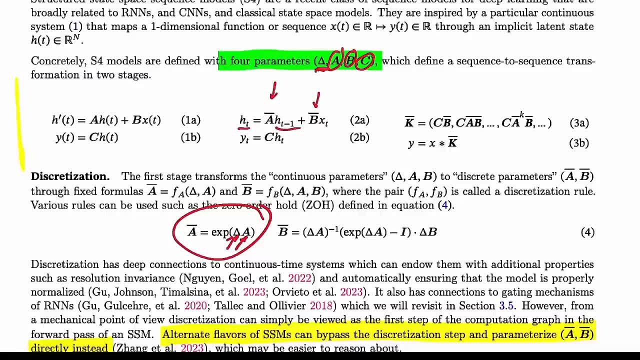 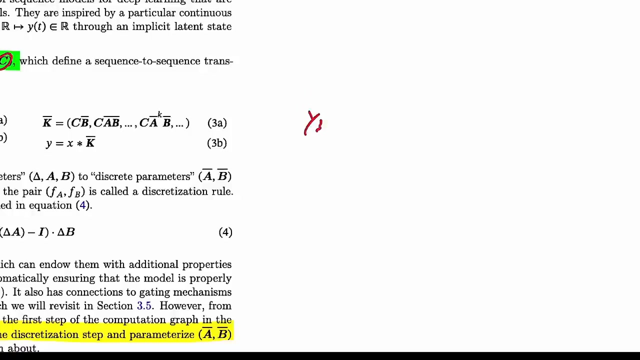 this is a super duper simple like the most plain recurrent neural network there is without even some any sort of non-linearity around here you can see this is just like a linear recurrent neural network if you will where you just kind of dampen in some way in some multi-dimensional way the last hidden state and then you add a a um projected version of the input the output is simply computed again as a linear function of the hidden state now since everything is linear you can what you can do is if you actually write this out, if you actually write out, I want to compute, sorry, I want to compute y3. What am I doing? I have an eraser. 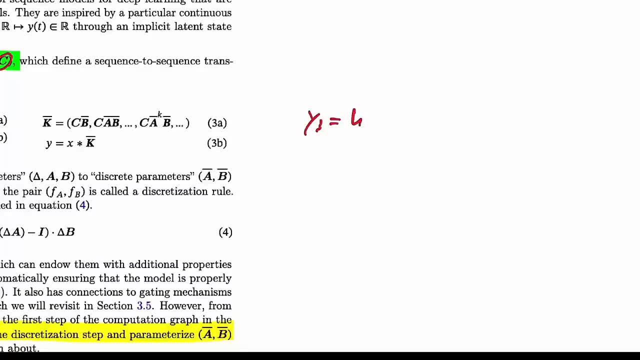 If you compute y3, you can say, oh, well, that's just h3, ah3 plus bx3. Oh, but what's h3? Well, h3 is just ah2. Oh, sorry, why is that multiplied by c, right? Well, that's just ah2 plus bx2. And what's h2? Well, that's just ah1 plus bx1. And so if I plug all of this in, I'm going to end up with y3 is equal to c times, c times a times a times ah1. Let's say that's the initial hidden state. Okay. 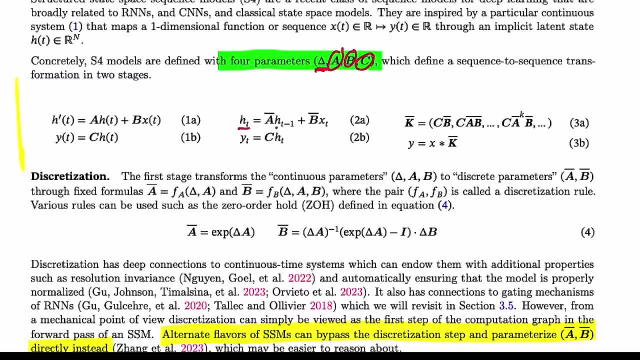 the next hidden state is produced from the last hidden state multiplied by what's called a bar, and a bar is simply a computation that results from this discretization parameter and the a matrix. again, don't worry, just consider, if you want, just consider this here to be a learnable matrix. 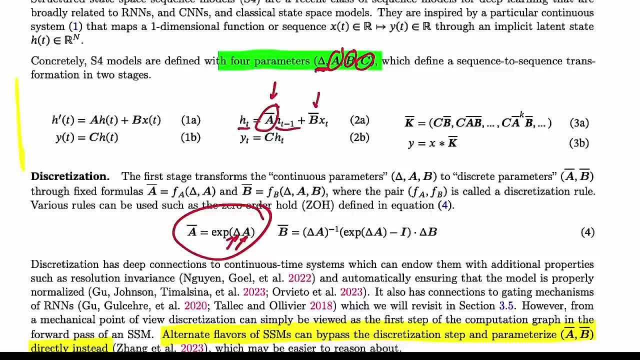 and this here to be a learnable matrix and in that you can see, from this perspective this is a super duper simple, like the most plain recurrent neural network there is, without even some any sort of non-linearity around here. you can see, this is just like a linear recurrent neural network, if you 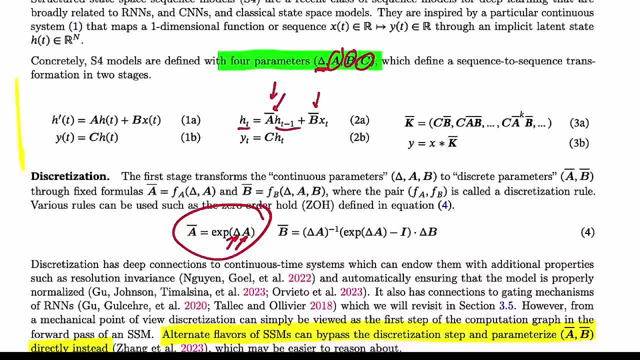 will, where you just kind of dampen in some way, in some multi-dimensional way, the last hidden state and then you add a, a projected version of the input. the output is simply computed again as a linear function of the hidden state. now, since everything is linear, you can, what you can do is: 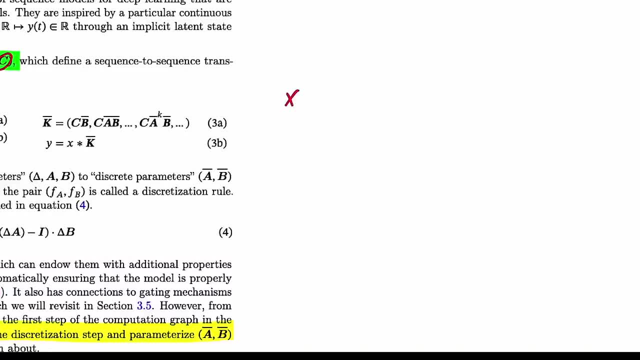 if you actually write the linear function of the hidden state, you can write the linear function of this out. you actually write out. i want to compute, sorry, i want to compute y3. what am i doing? i have an eraser. if you compute y3, you can say: oh well, that's just h3, uh, ah3 plus bx3, oh, but what's h3? 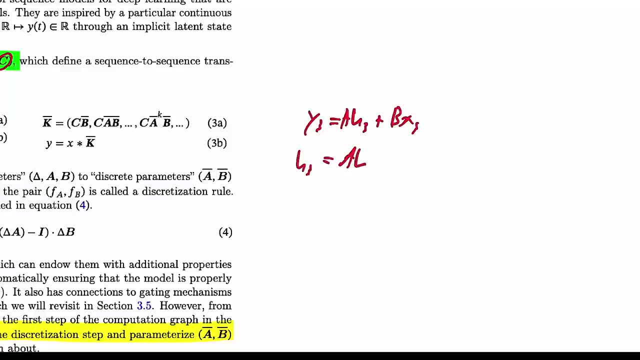 well, h3 is just ah2. oh, sorry, why is that that multiplied by c, right? well, that's just ah2 plus bx2. and what's h2? well, that's just ah1 plus bx1. and so if i plug all of this in, i'm going to end up with 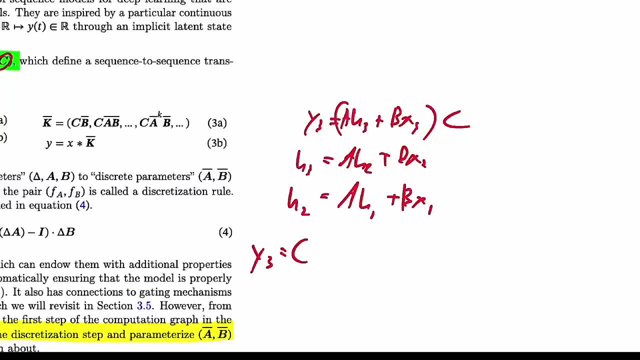 y3 is equal to c times um, c times a times a times a of h1. let's say that's the initial hidden state. so you can see. you can multiply this out. what you'll end up with is, like you can, you'll end up with like c a, a, a, a, b, x1, c plus c a, a, a, b, x2 and so on, so plus. 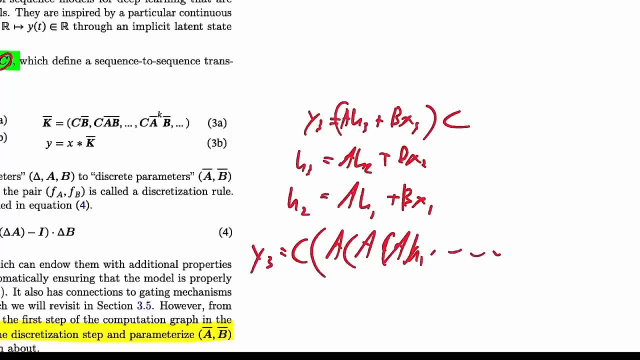 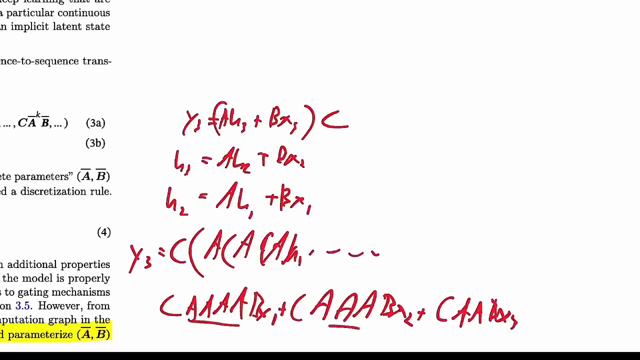 So you can see you can multiply this out. What you'll end up with is like, you'll end up with like c a a a a bx1, c plus c a a a bx2, and so on. So plus c a a bx3. So there's kind of the number of a's just different depending on how many time steps that particular x is in the past. But you can see I can multiply, I can multiply all of this out. And what that allows me to do is, that allows me to say, well, all of this here is just constant. No, not this. All without x. All of these matrices here are just constant learnable parameters. This too. This too. 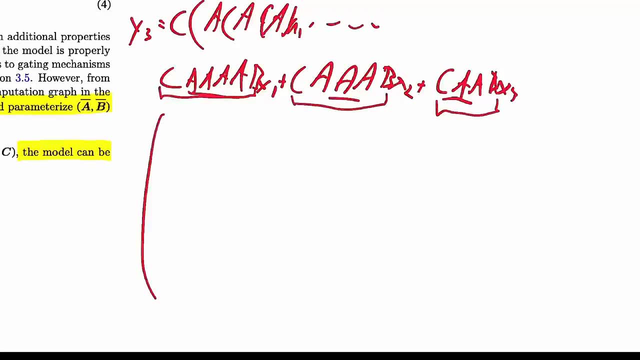 So I can just consider this as a vector, a dot product of c a a a a b, c a a a b, c a a b, and so on, 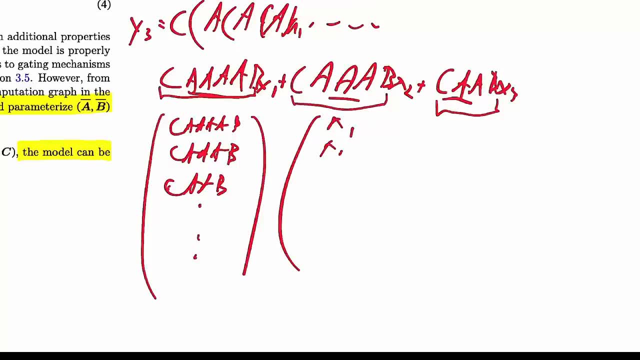 with, x1, x2, x3, and so on. 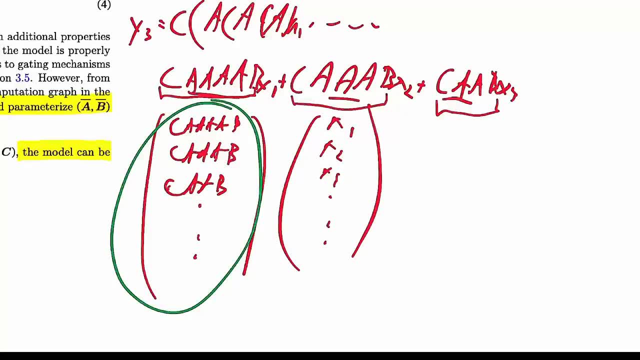 And this here, I can perfectly pre-compute. 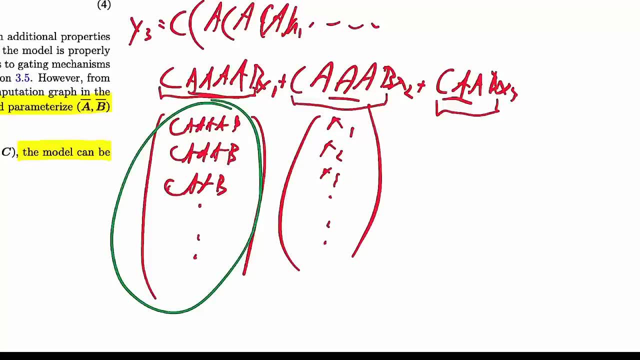 You know, I just, after each learning step, these are just learned parameters. Therefore, I can perfectly pre-compute that. 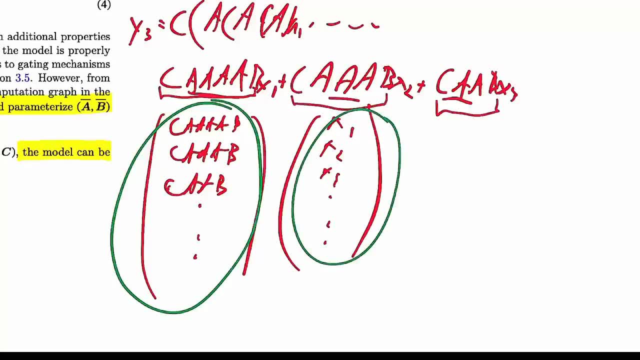 And when a new sequence comes, I just dot product it in, and I have the full output. I have the output available instantly. 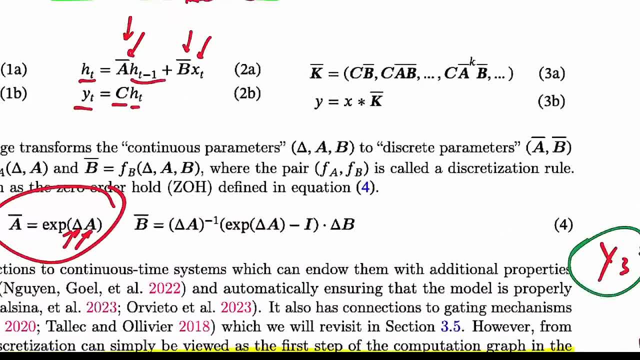 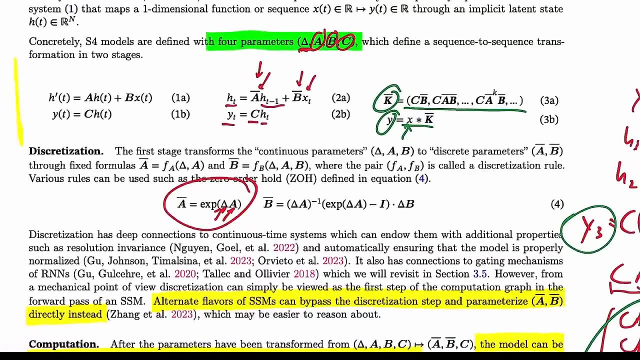 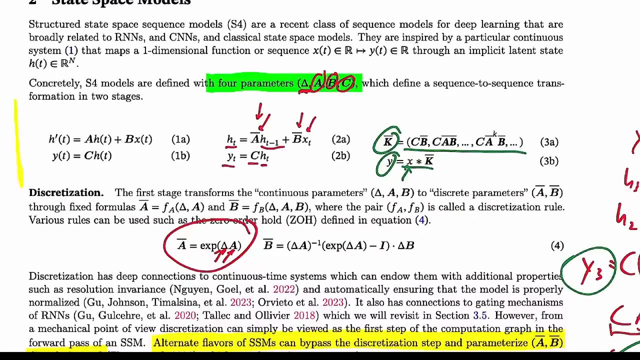 And that's what they do over here. So you can see they built this kernel out of this. And then they can say, well, the output is simply going to be a multiply the input as a vector by my kernel. And bada boom, I just have it all, I have it all available, right? And that's, and that is why, and you can hopefully see that this is a convolution. 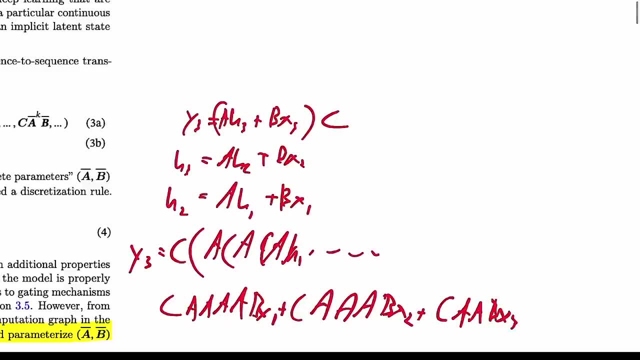 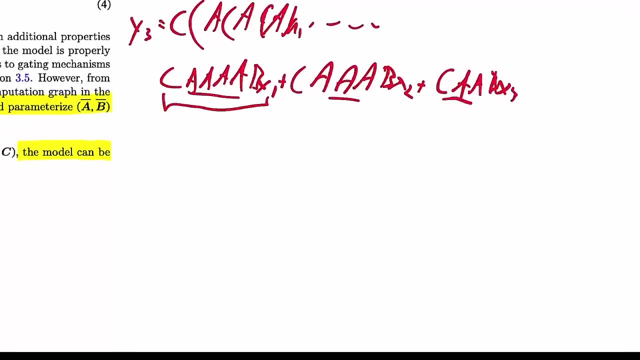 c, a, a, b, x3, so there's kind of the number of a's just different depending on how many time steps that particular x is in the past. but you can see, i can multiply all of this out and what that allows me to do is that allows me to say: well, all of this here is just constant. no, not this all without x. 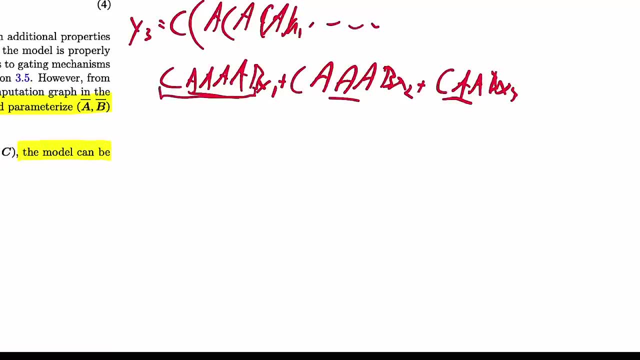 all of these matrices here are just constant learnable parameters. this too, this too. so i can just consider this as a vector, a dot product of c a a a a b, c a a a, b, c a a b and so on, with x, x1, a a, c, and so on. and this here i can perfectly pre-compute. you know, i just after each learning, 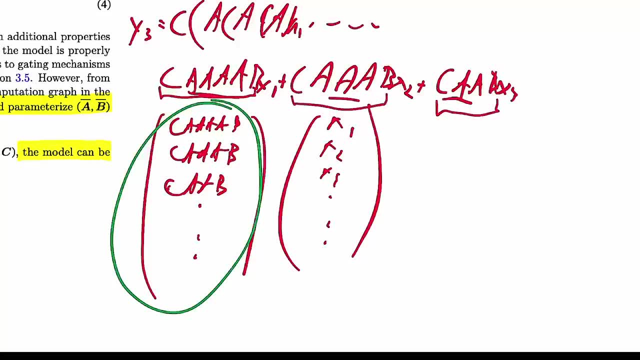 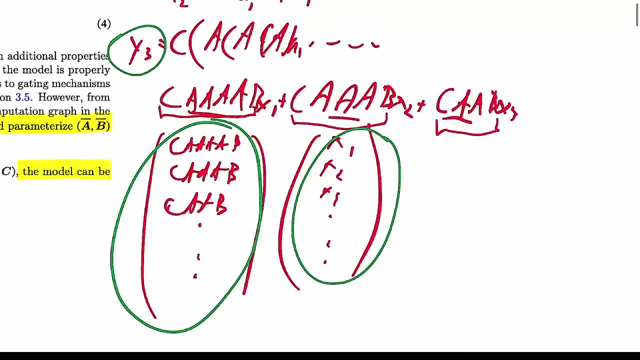 step. uh, these, these are just learned parameters. therefore, i can perfectly pre-compute that and when a new sequence comes, i just dot product it in and i have the full output. i have the output available instantly and that's what they do over here. so you can see they built this kernel. 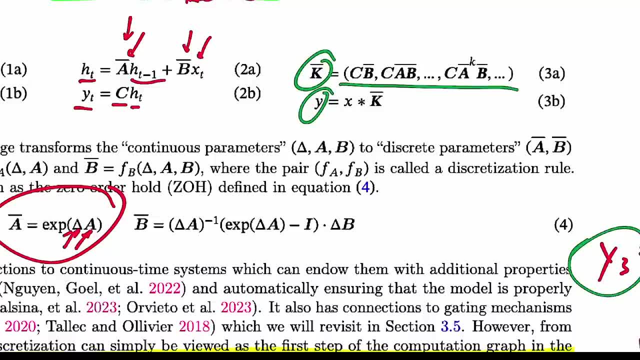 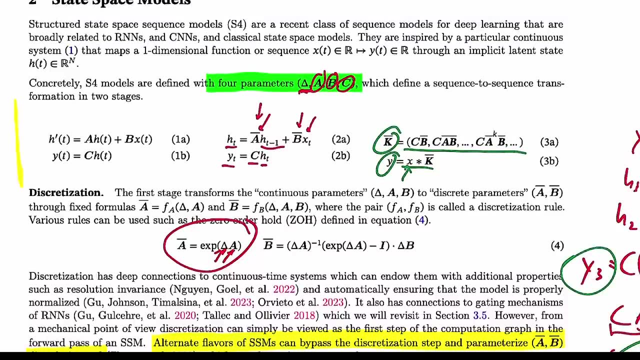 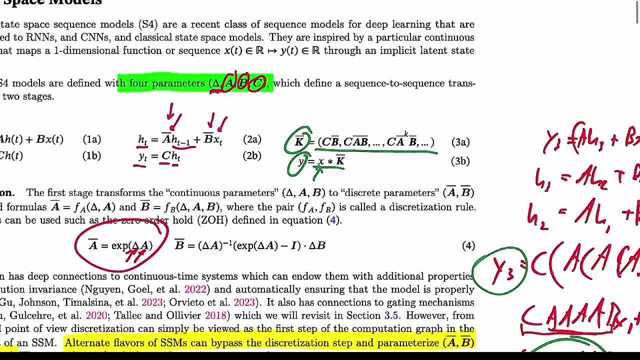 out of this and then they can say: well, the output is simply going to be: I multiply the input as a vector by my kernel and, ba-da-boom, I just have it all available, and that is why you can hopefully see that this is a convolution. so if you not only want one output, but you actually want each of the output, of each of the 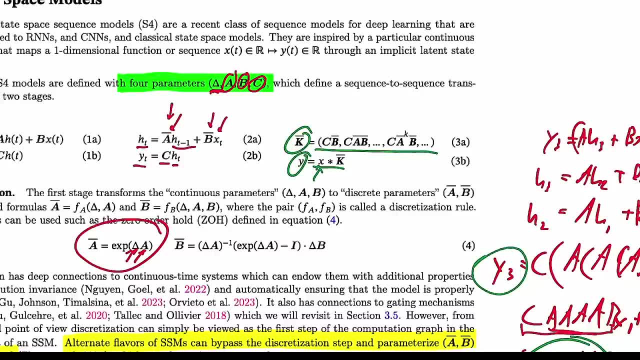 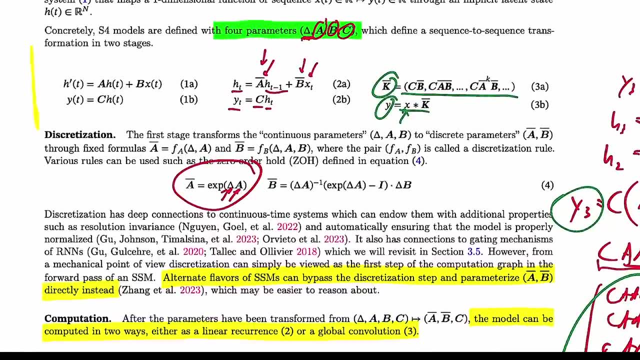 time steps. this just results in a convolution operation that you can do, and that's why the S4s and so on were so extremely efficient, because you can just compute all at the same time. all is linear, all is fixed, just forward. prop is one convolution. 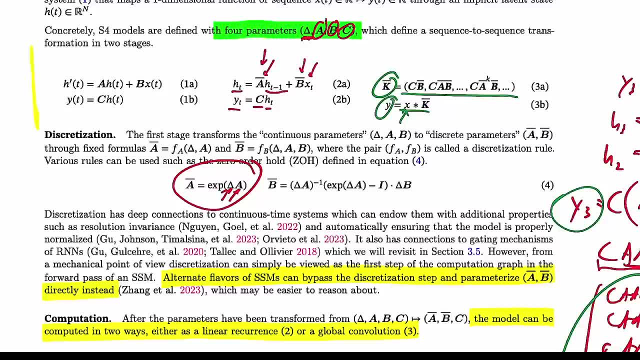 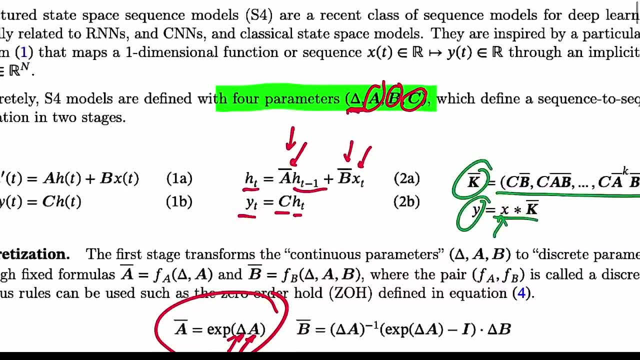 back prop. super easy. okay, that's it. and essentially in Mamba or in structured state spaces, all we're doing is we're making A, B, C and this delta here input dependent. that's it. that's the whole thing. 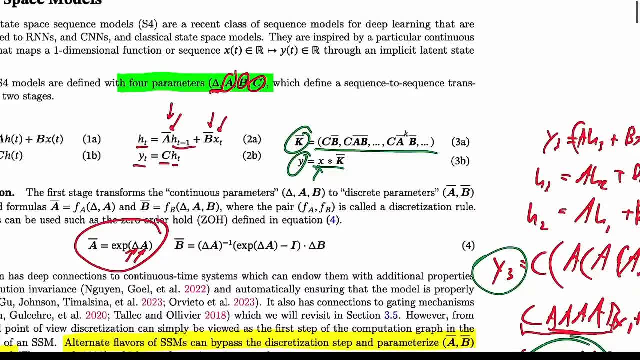 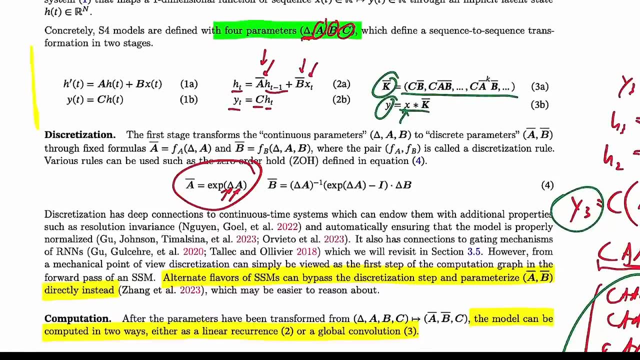 So if you now, if you not only want one output, but you actually want each of the output of each of the time steps, this just results in a convolution operation. That you can do. And that's why the S4s and so on were so extremely efficient because you can just compute all at the same time. All is linear, all is fixed. 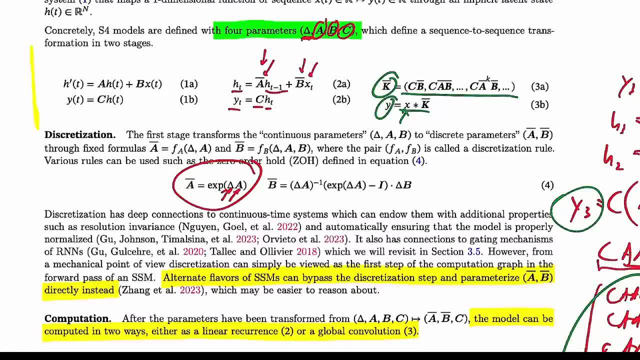 Just forward prop is one convolution, back prop, super easy, right? Okay. That's it. 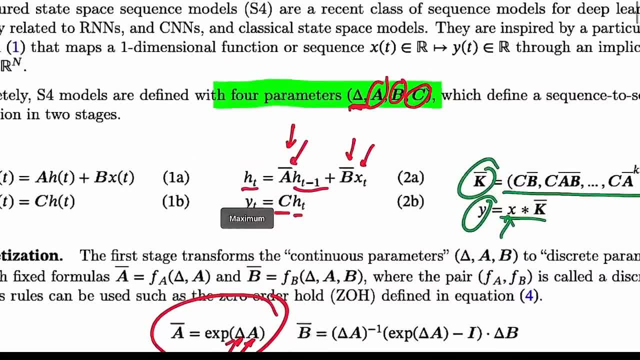 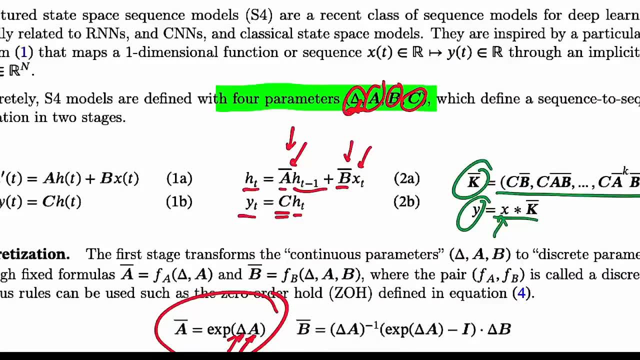 And essentially in Mamba, we're not, we're in structured state spaces. All we're doing is we're making A, B, C, and this delta here input dependent. 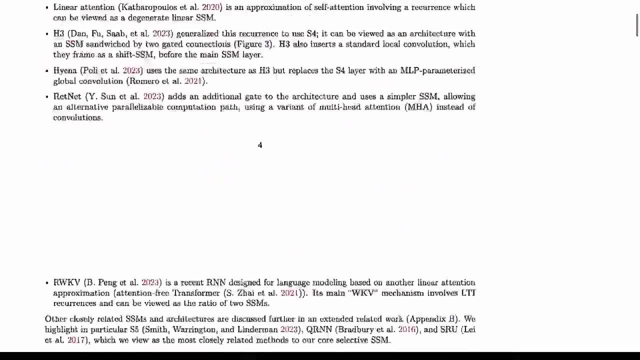 That's it. That's the whole, that's the whole thing. 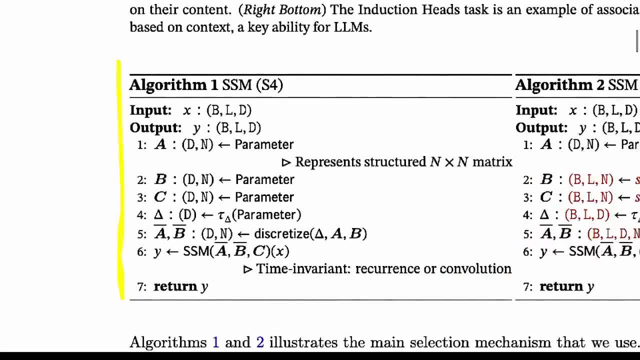 You can see this in the algorithm here. You can see you have the SSM here. A, B, C go into it. In fact, no, sorry, A bar and B bar are computed from this thing right here. 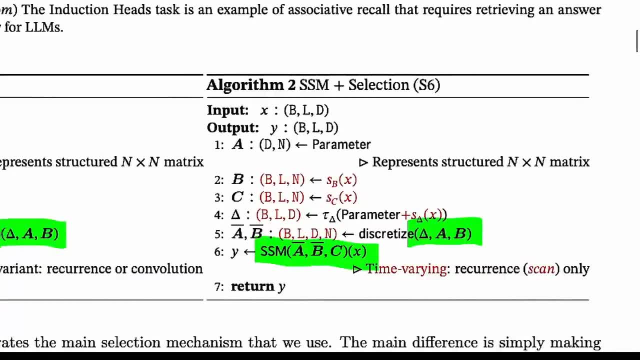 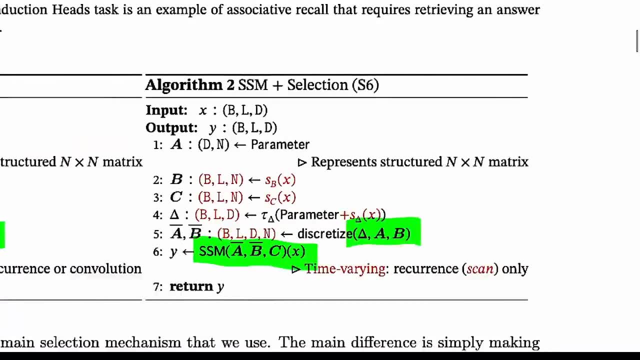 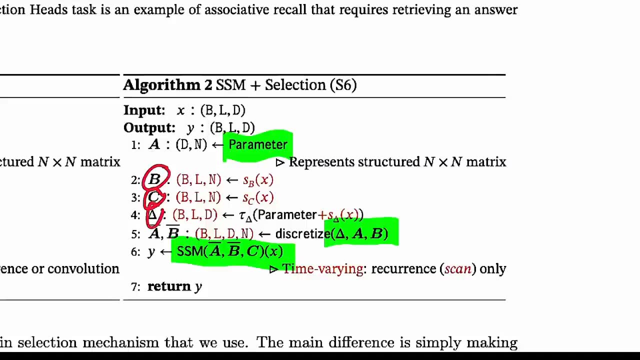 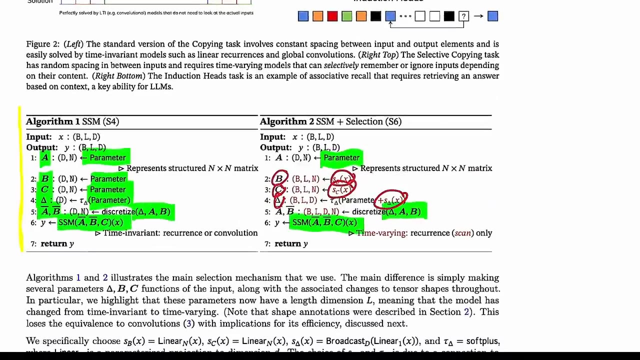 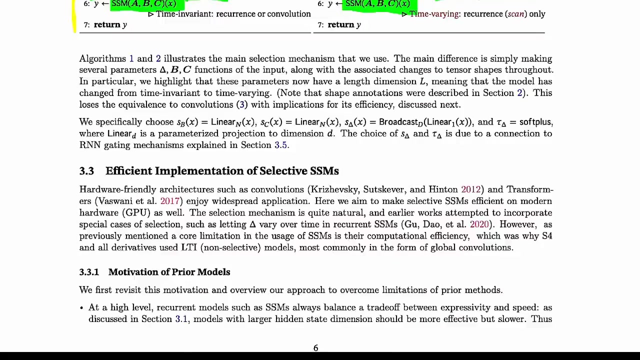 That's exactly the same here and here. But now instead of B, C, this, and A being just simple parameters, A is still a parameter. However, everything else you can see, B, C, delta is computed from the input. Okay. And that means, it still means you can do the zoom thing, but the zoom thing, now you have to make that input dependent. 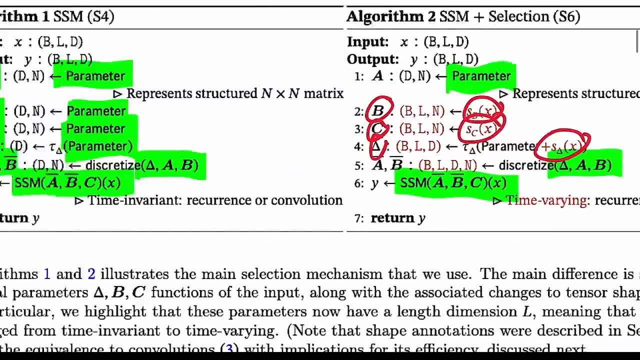 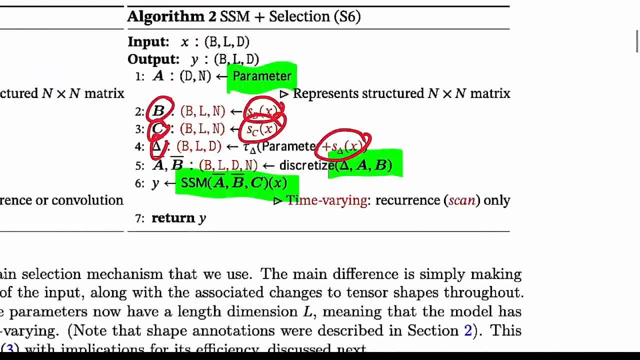 And specifically, specifically, everything gets, it gains a dimension. So here, see, this has no, this is the same for each time step. This now is different for each time step. Okay. 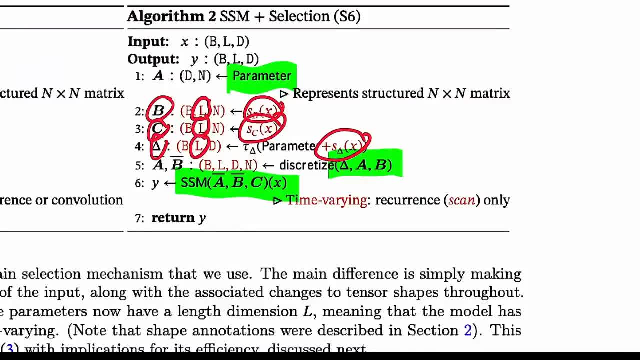 Because each time step has a different input and therefore these things gain an extra dimension. 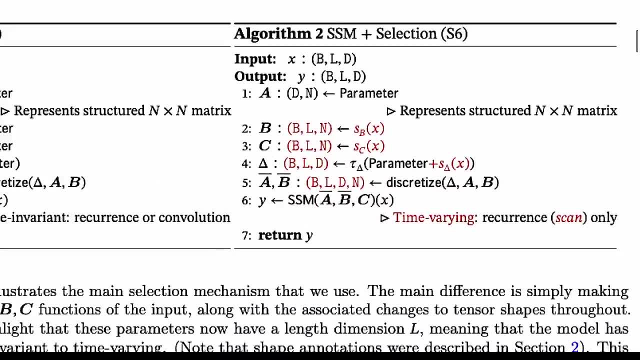 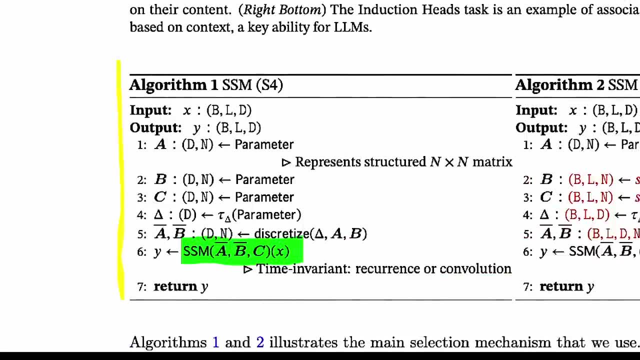 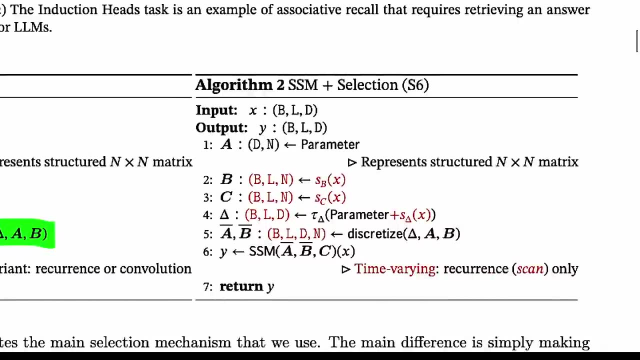 you can see this in the algorithm here. you can see you have the SSM here. A, B, C go into it. in fact, A bar and B bar are computed from this thing right here. that's exactly the same here and here, but now, instead of B C, this: 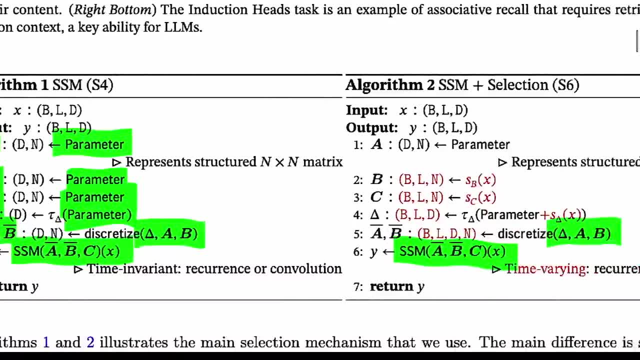 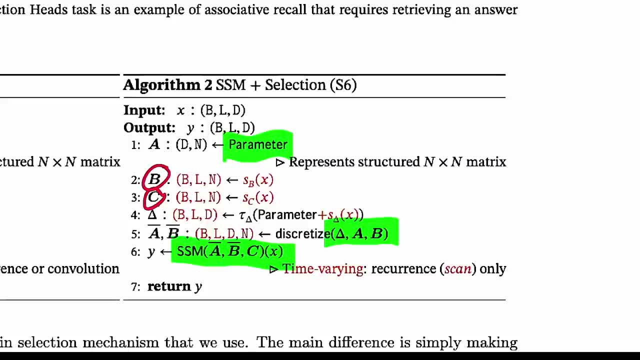 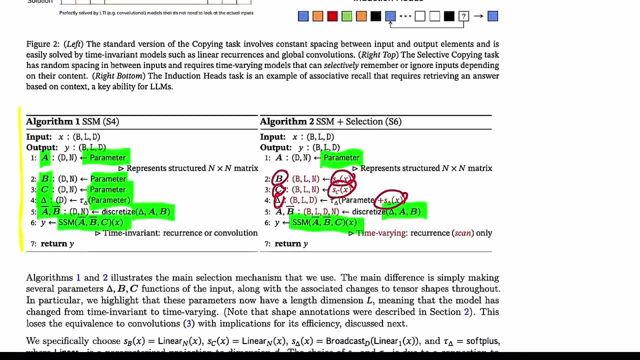 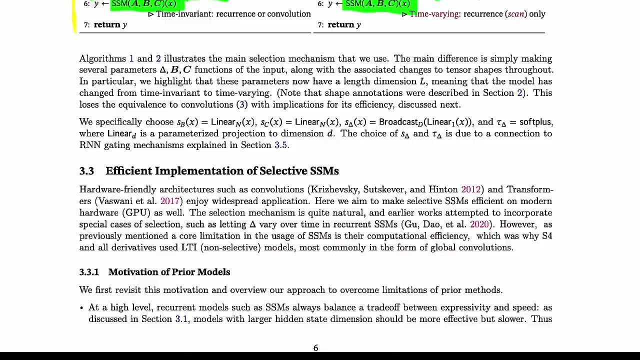 and A being just simple parameters. A is still a parameter. however, everything else you can see- B, C, delta- is computed from the input and that means it still means you can do the zoom thing. but the zoom thing now you have to make that input dependent. 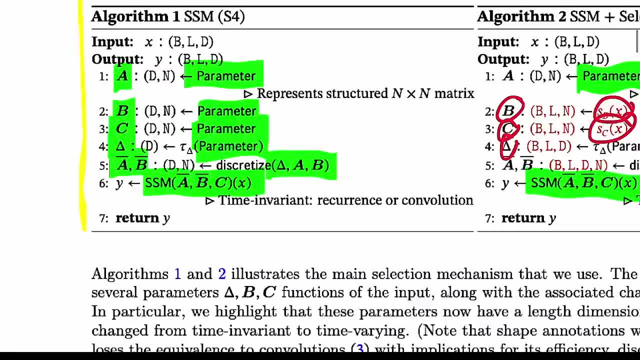 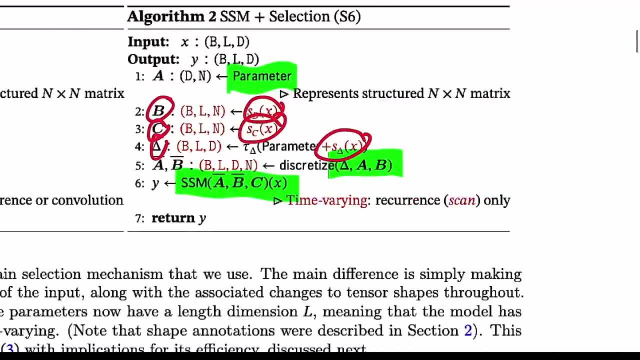 and specifically, specifically, everything gains a dimension. so here see, this has no, this is the same for each time step. this now is different for each time step. okay, because each time step has a different input and therefore these things gain an extra dimension. 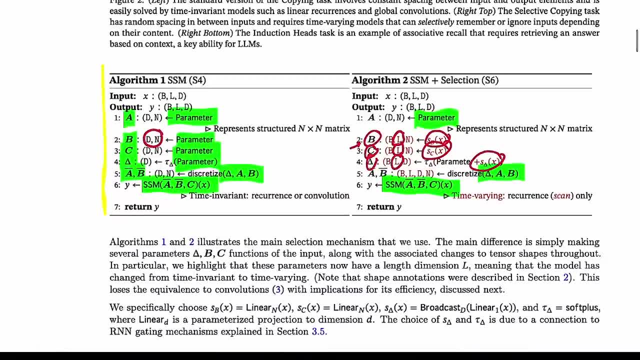 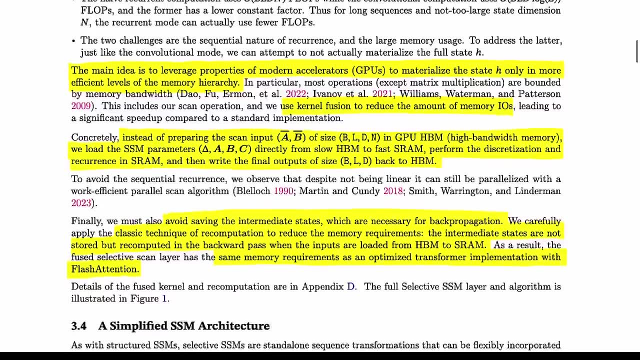 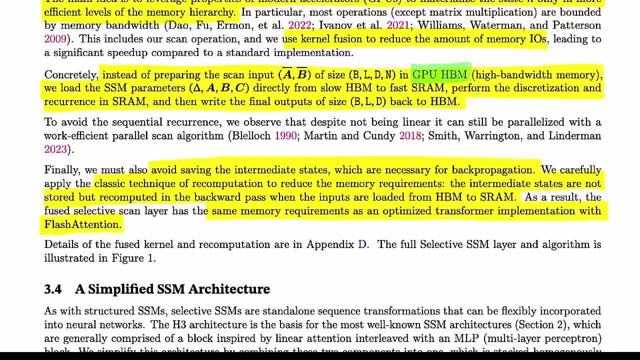 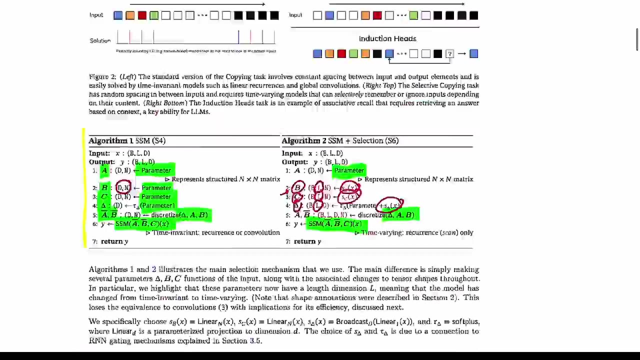 and that's kinda bad because that makes them L times bigger than previously. so what do we do in order to make that still fast? they differentiate right. they differentiate now between two things: GPU, high bandwidth memory and what's called SRAM. so GPUs have two different types of memory. 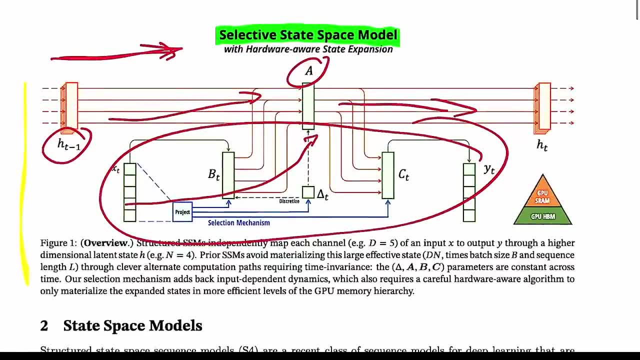 I didn't know before this paper but they have the main memory is kind of the slow memory that's this right here. that's high bandwidth memory, but that's slow even though it's high bandwidth. well, I guess high bandwidth doesn't mean low ping. 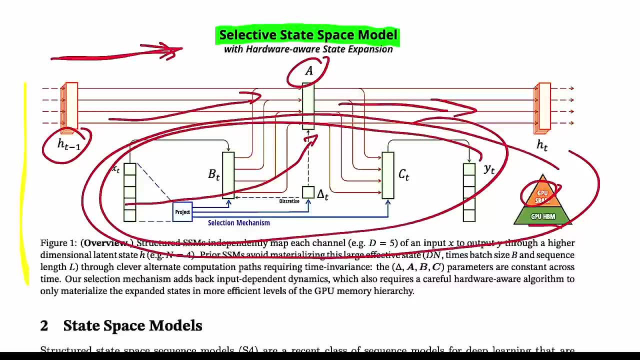 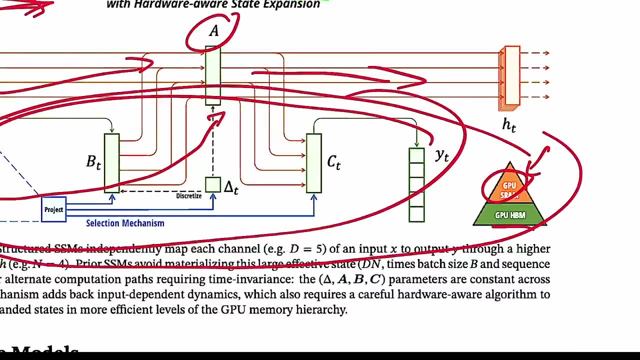 alright, that's low. and then SRAM is really small but it's really fast. and they realize, hey, if we want to do the matrix multiplications, these happen in this SRAM. that's essentially the cache, that's the fast stuff. the bulk of work is actually moving stuff. 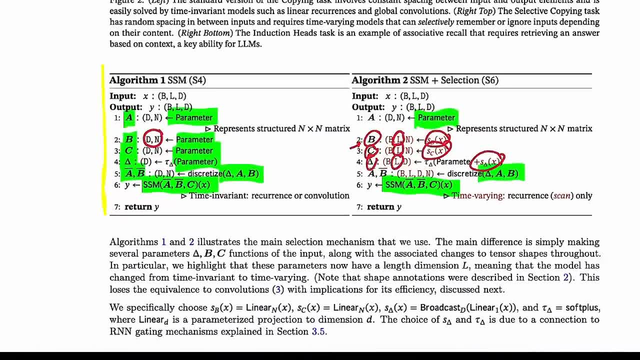 And that's kind of bad because that makes them L times bigger than previously. 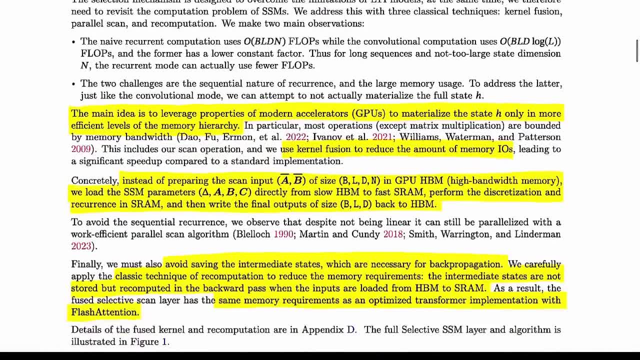 So what do we do in order to make that still fast? 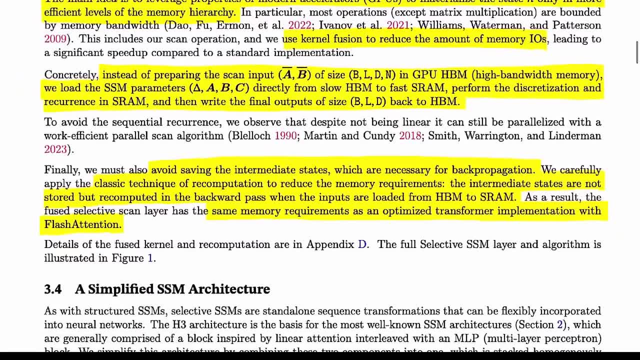 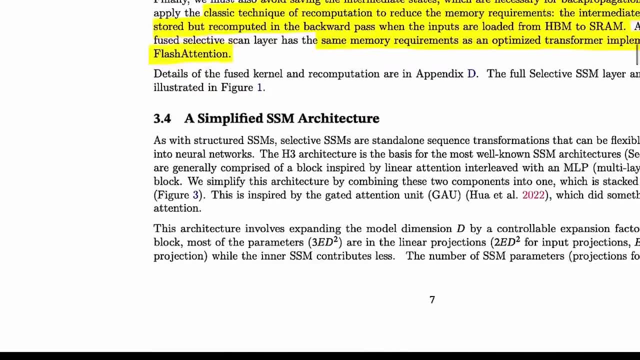 They differentiate now between two things. GPU high bandwidth memory and what's called SRAM. So GPUs have two different types of memory. 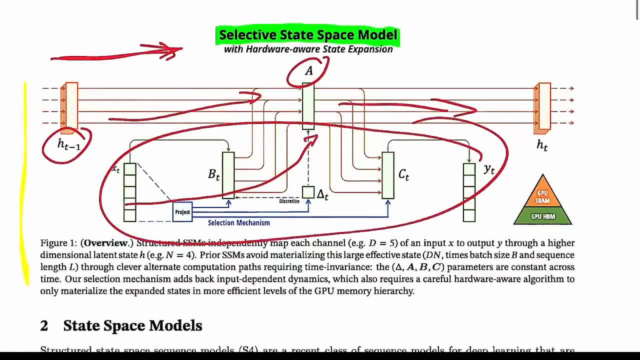 I didn't know before this paper, but they have, the main memory is kind of the slow memory. That's this right here. That's high bandwidth memory, but that's slow, even though it's high bandwidth. Well, I guess high bandwidth doesn't mean low ping. All right. 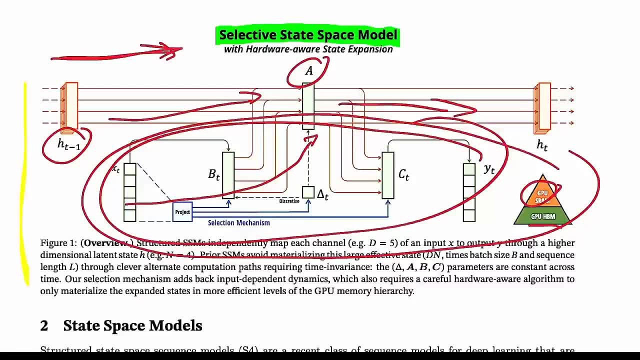 That's slow. And then SRAM is really small, but it's really fast. And they realize, hey, if we want to do the matrix multiplications, these happen in this SRAM. That's essentially the cache. That's the fast stuff. 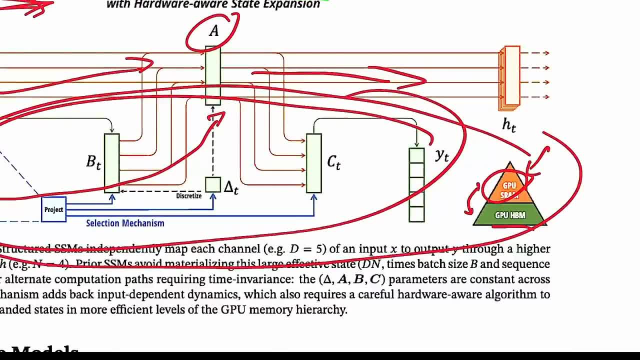 The bulk of work is actually moving stuff between the two types of memory. 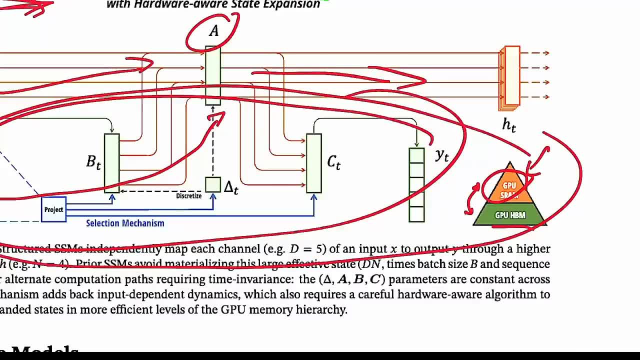 Moving stuff between the two is the slow thing. And therefore we've just made that L times bigger. And therefore we made that moving L times slow. Because the multiplications aren't that slow. 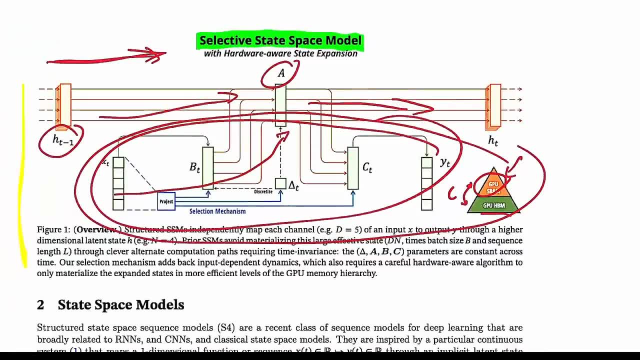 It's actually moving the stuff around. And therefore they come up with a scheme where they don't have to move as much stuff. 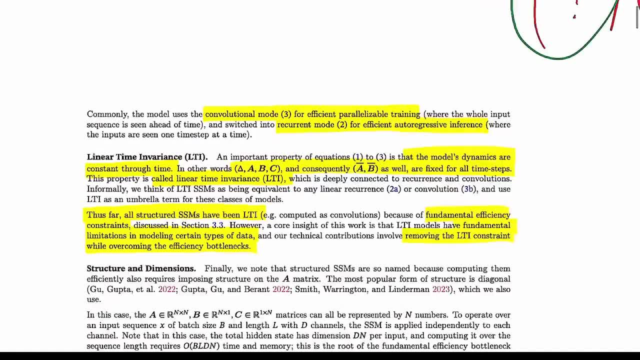 That's essentially it. You can look at the code, but in the end, it just comes down to that. 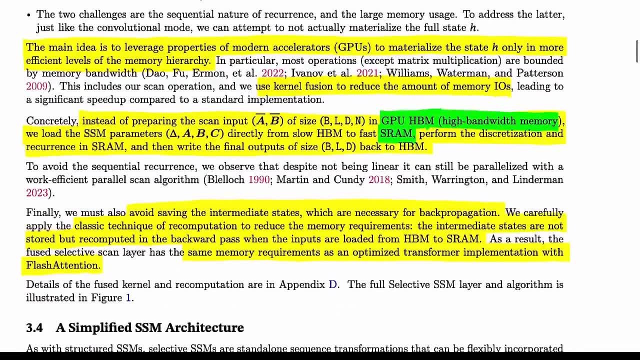 It comes down to moving stuff around, moving big stuff around is slow. And therefore they say, you know, 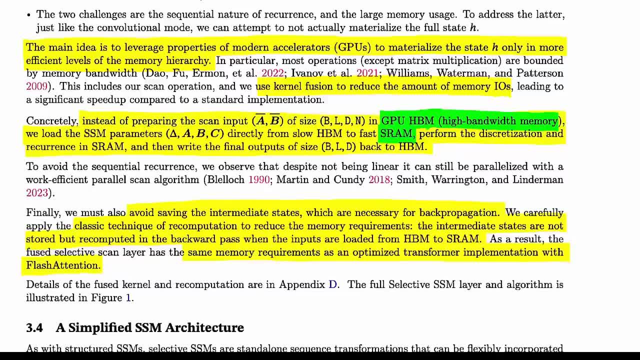 instead of computing this kind of stuff, this kind of scan inputs in GPU, 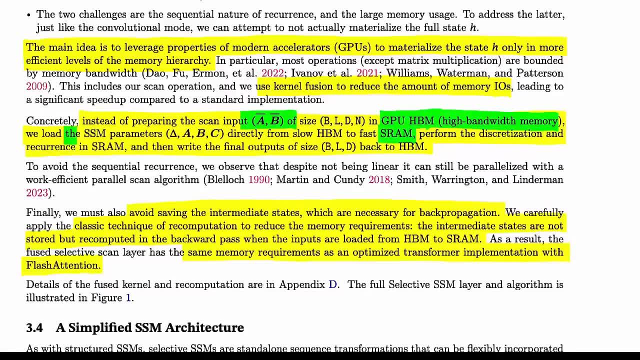 HBM, we load the parameters themselves directly to fast SRAM, perform the discretization and recurrence in SRAM, and then write the final outputs back to HBM. 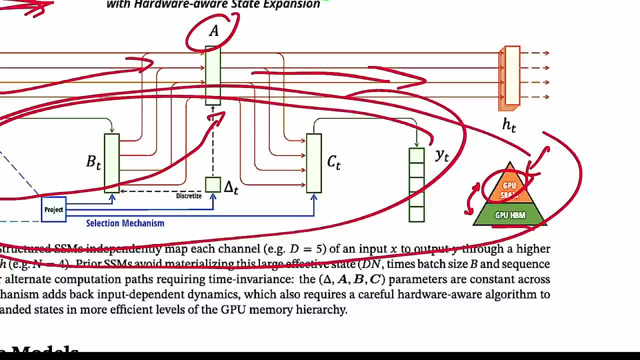 between the two types of memory. moving stuff between the two is the slow thing and therefore we've just made that L times bigger and therefore we made that moving L times slower because the multiplications aren't that slow, it's actually moving the stuff around. 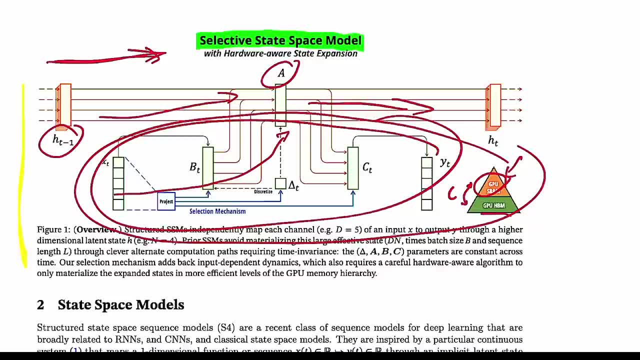 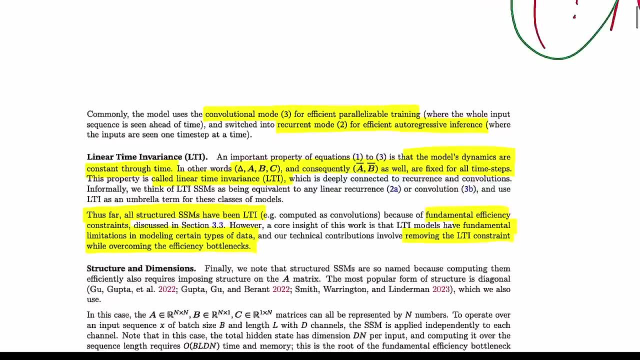 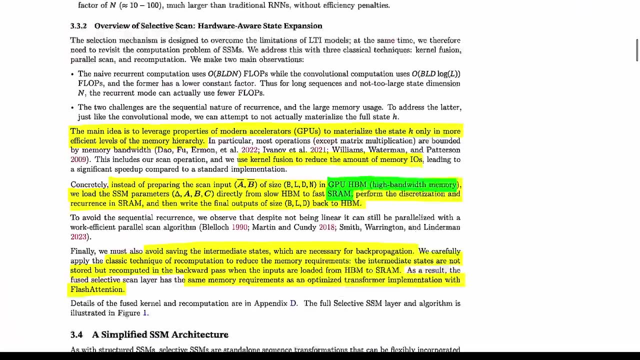 and therefore they come up with a scheme where they don't have to move as much stuff. that's essentially it. you can look at the code, but in the end it just comes down to that. it comes down to moving stuff around. moving big stuff around is slow. 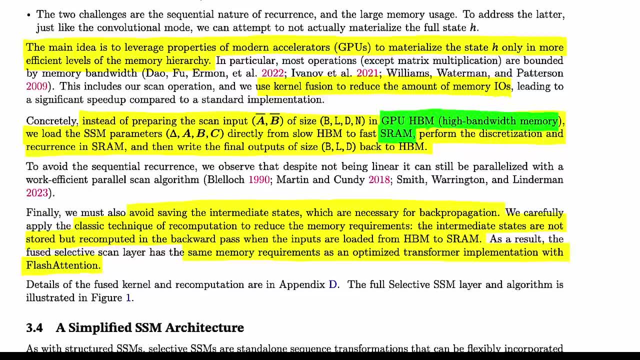 and therefore they say: instead of computing this kind of stuff, this kind of scan inputs, in GPU HBM, we load the parameters themselves directly to fast SRAM, perform the discretization and recurrence in SRAM and then write the final outputs back to HBM. they save themselves. 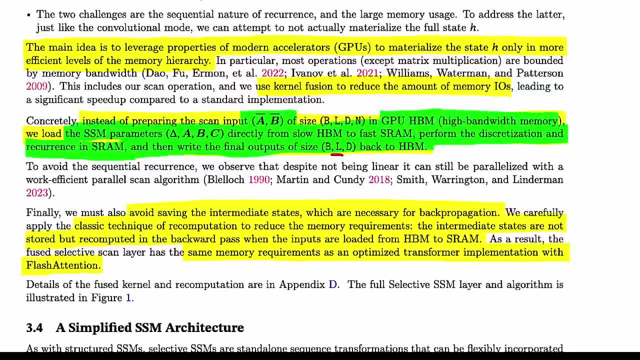 they actually don't save themselves an L, they save themselves an N, and N is the discretization expression, which is the expansion factor. so during this discretization you kind of need to expand dimensionality, expand some of these things and they save themselves that expansion and therefore are a lot faster. 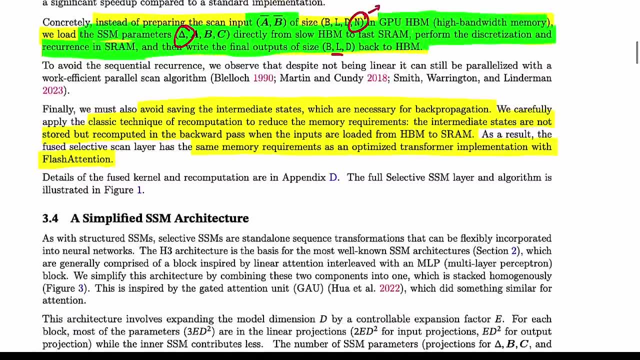 I'm not going to go deeper into this, except saying what they say down here. they make use of this reduction of data movement plus a recomputation of intermediate states, and that results in that the used selective scan layer has the same memory requirements as an optimized transformer implementation. 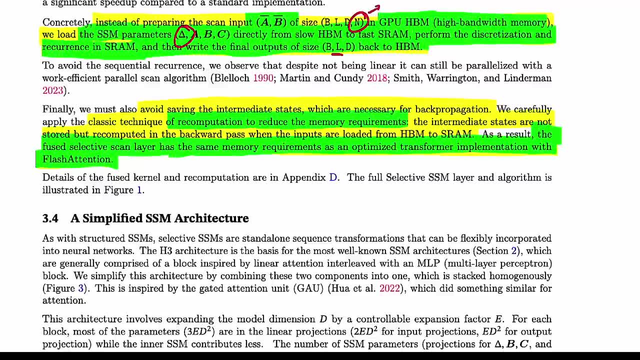 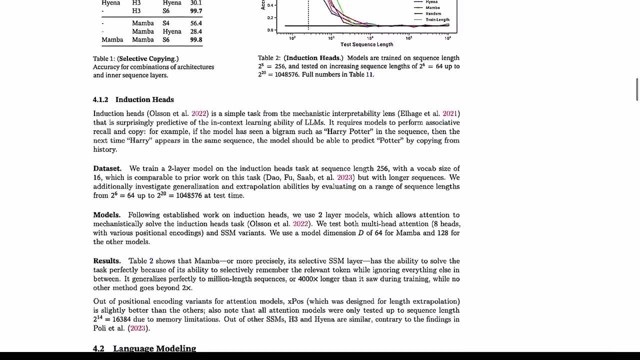 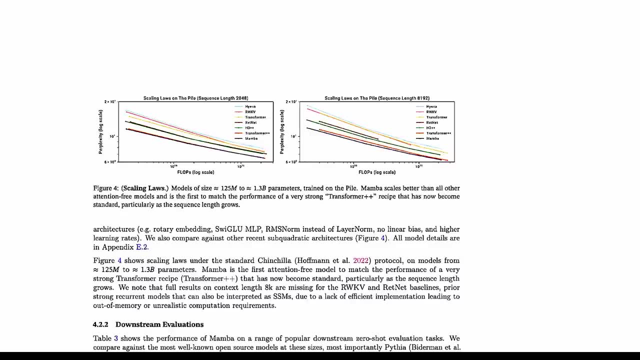 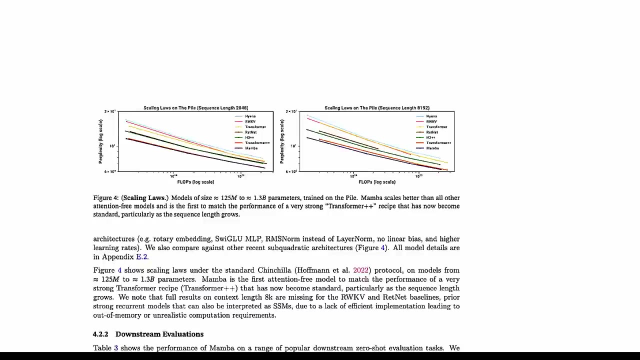 with flash attention, and I believe that should give you a good good idea of the combination of what kind of is required right here. so again, they can still do the zoom, except now the elements are input dependent and therefore they have to do the zoom differently. and they do the zoom using, not the convolution. 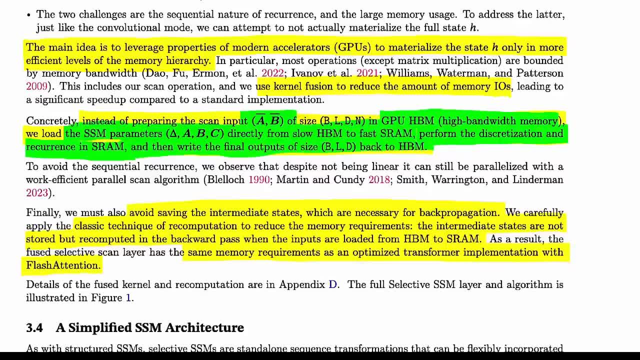 They save themselves. They actually don't save themselves an L. 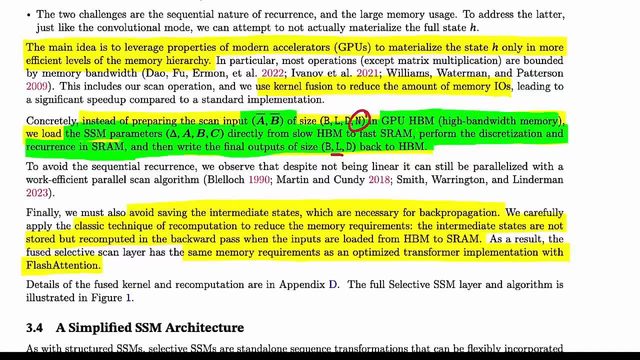 They save themselves an N. And N is the distance discretization expansion factor. So during this discretization, you kind of need to expand dimensionality, 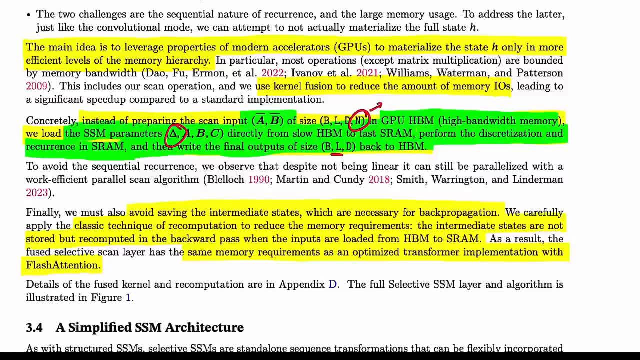 expand some of these things, and they save themselves that expansion and therefore are a lot faster. 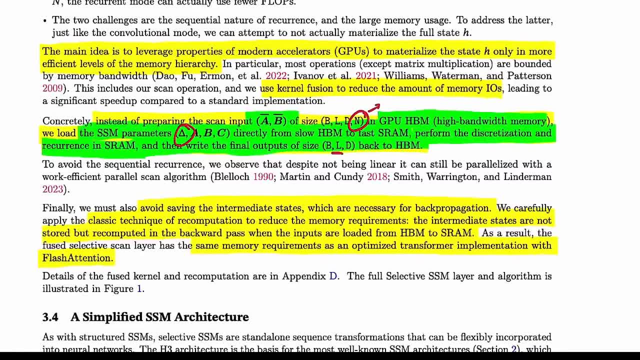 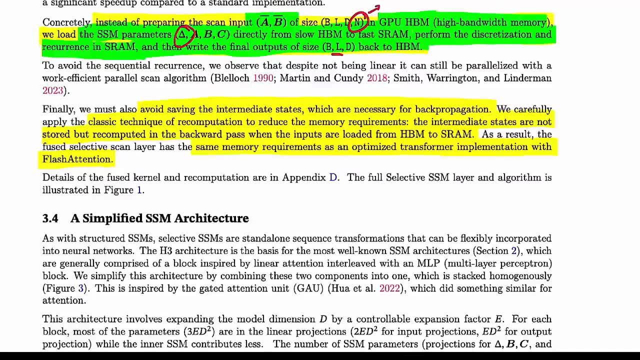 Yeah. So I'm not going to go deeper into this, except saying what they say down here. You know, they make use of this, this reduction of data movement, plus a recomputation of intermediate states. And that results in that the used selective scan layer has the same memory requirements as an optimized transformer implementation with flash attention. 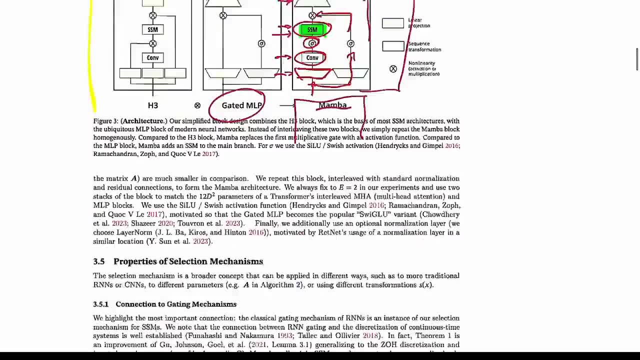 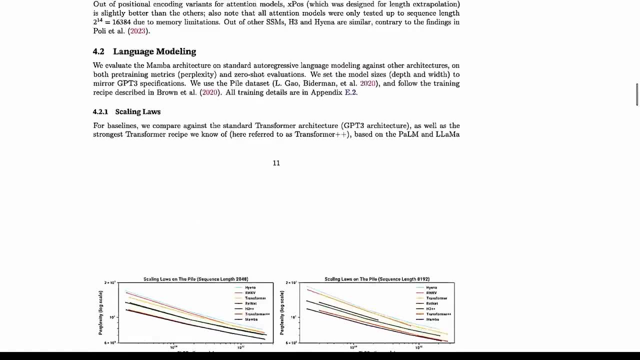 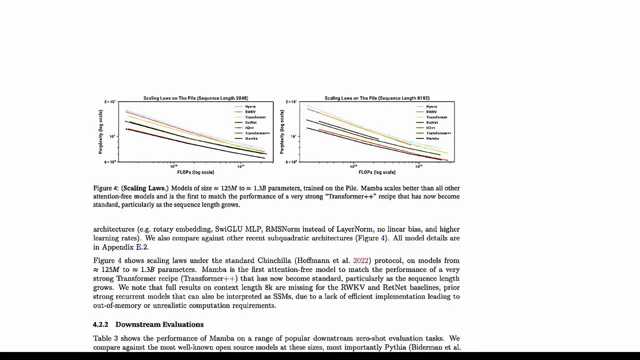 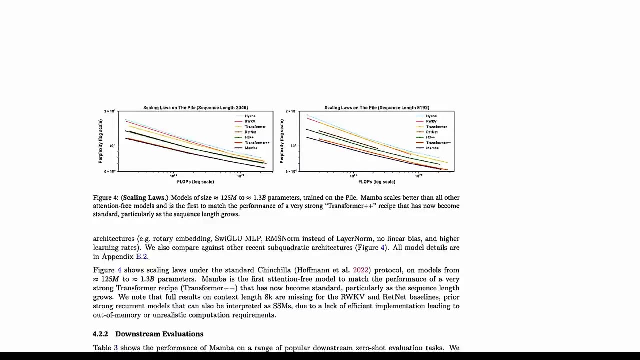 And I believe that should give you a good, good idea of the combination of what kind of is required right here. So again, they can still do the zoom, except now the elements are input dependent, and therefore they have to do the zoom differently. And they do the zoom using not the convolution, because the convolution would require the kernel to be constant, but they now do it via what's called the prefix sum. 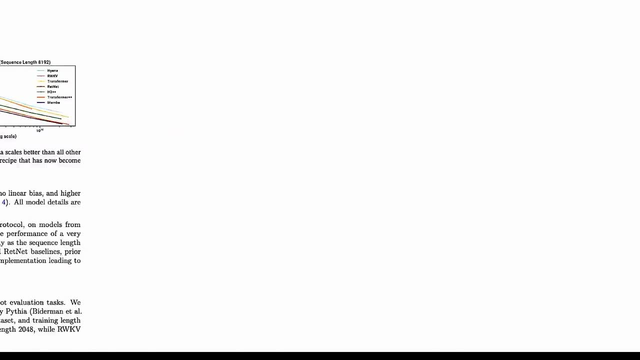 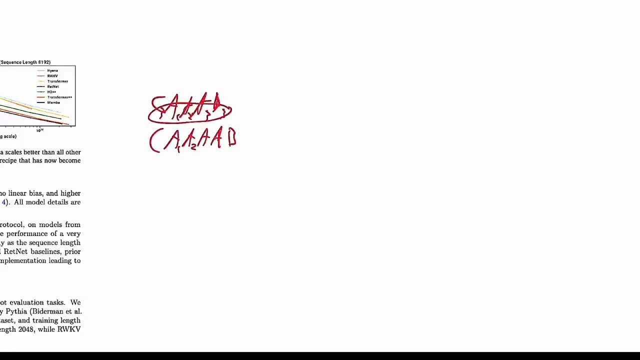 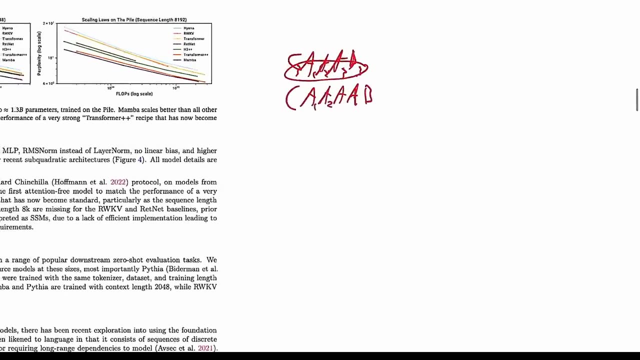 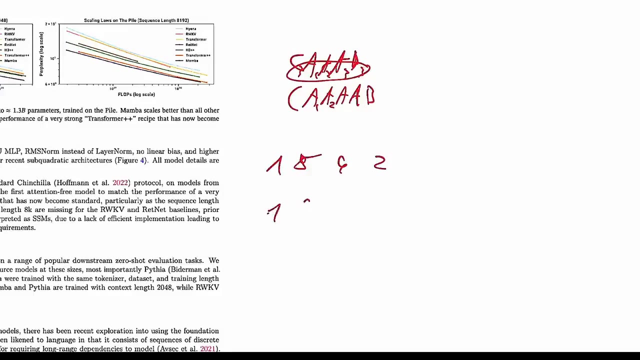 So you can see all of these are now different. So you can't do like the tricks from before anymore. And what they do is a prefix sum, and the prefix sum is just, the simplest form is when you have an array like one, five, nine, two, to compute the sum, the cumulative sum, like one, six, 15, 17. 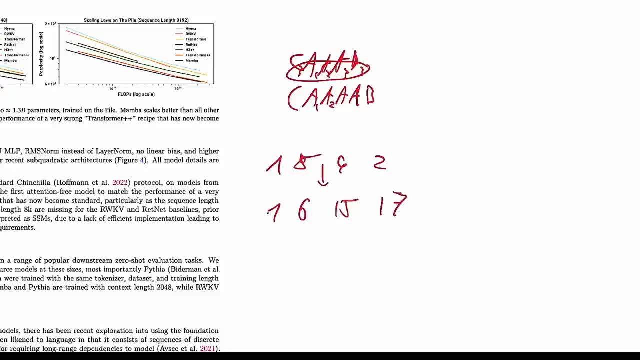 So the way you compute this in an efficient manner, you can then use this down here for various things. 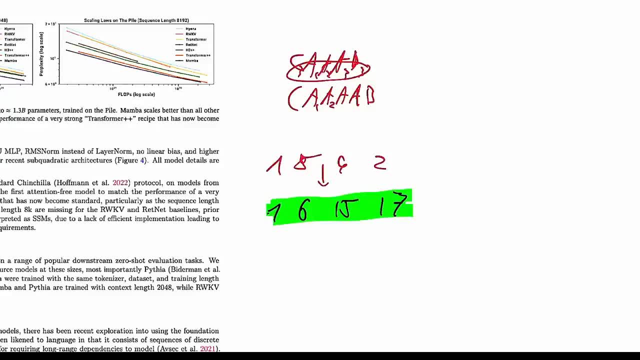 It's very simple, right? And this is useful in a lot of algorithm, but to avoid recomputing a lot of this stuff, you can use prefix sums to kind of pre-compute all of the sums, or in this case, all of the multiplications of different things together. 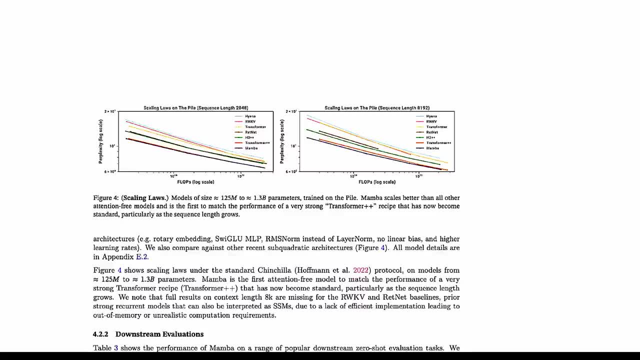 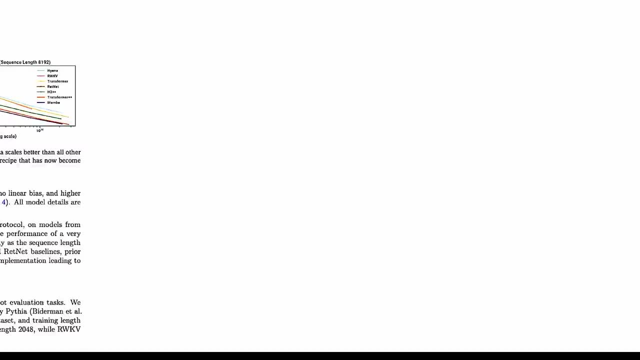 because the convolution would require the kernel to be constant, but they now do it via what's called the prefix sum. and the prefix sum is, and they call it, a parallel scan, but it's essentially the thing that computes this a times a times, a times b, and then c, a, a, a, b. 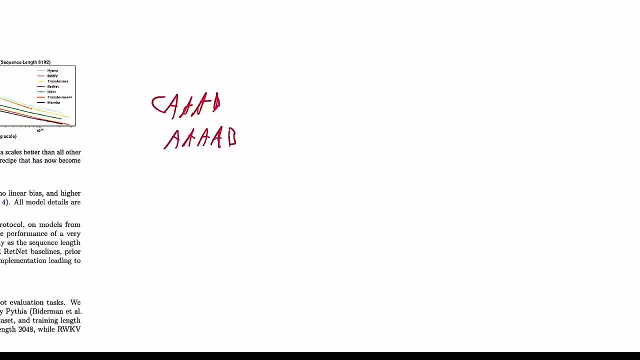 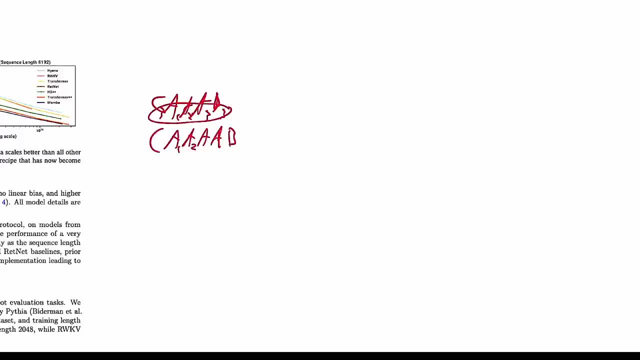 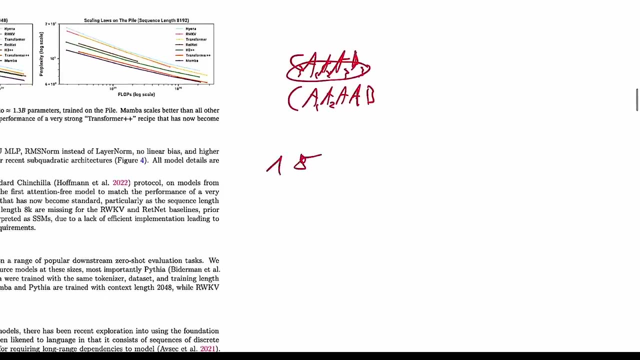 so you can't do the tricks from before anymore, and what they do is a prefix sum, and the prefix sum is just the simplest form, is when you have an array like 1,, 5,, 9,, 2 to compute the sum, the cumulative sum. 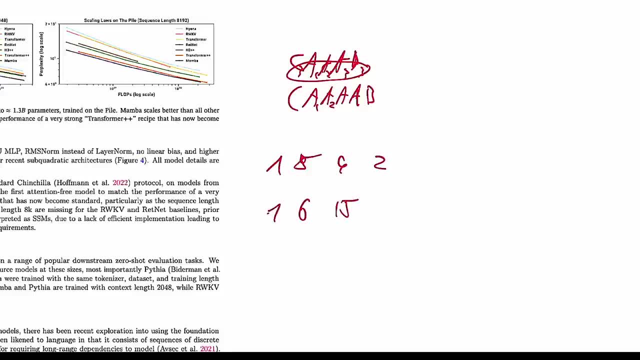 like 1,, 6,, 15,, 17. so the way you compute this in an efficient manner. you can then use this down here for various things. it's very simple, right, and this is useful in a lot of algorithms. but to avoid recomputing a lot of this stuff, 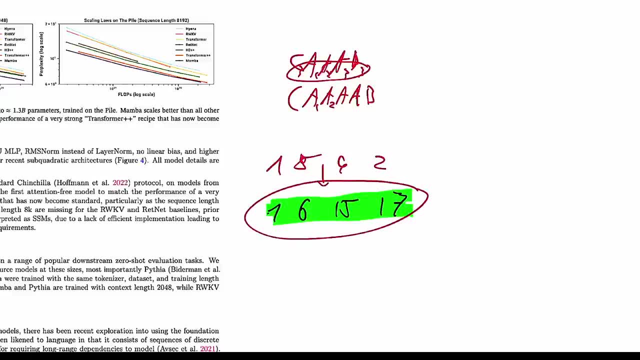 you can use prefix sums to kind of precompute all of the sums or in this case, all of the multiplications of different things together, and then you can use those and for example, if you say what's the sum from here to here, you can just subtract. 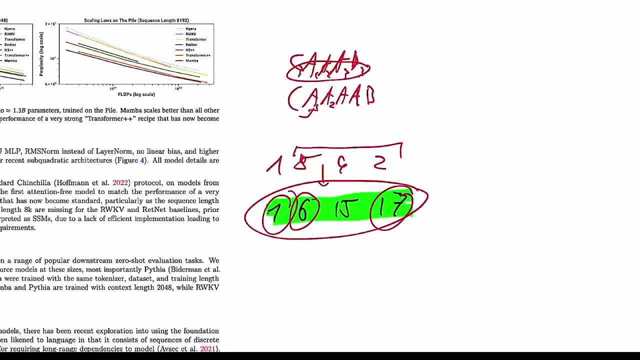 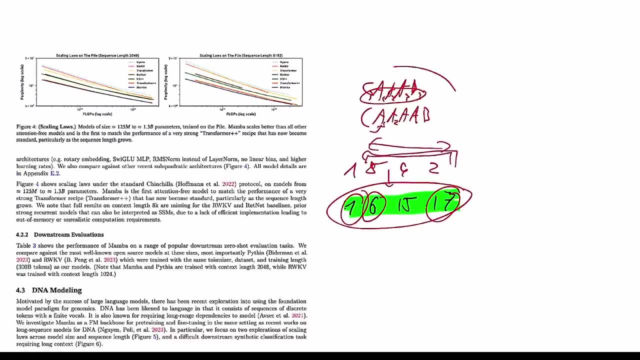 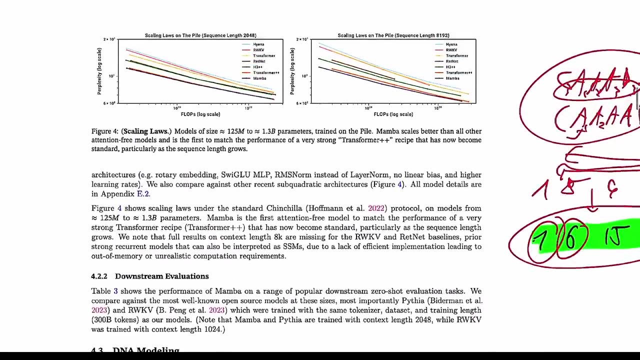 from 17, you can subtract 6 or 1, sorry 1- and you can say the sum here is 16 without having to compute it again. same principle goes for how they make this here fast. the scaling laws look really scaly. so they the perplexity in. 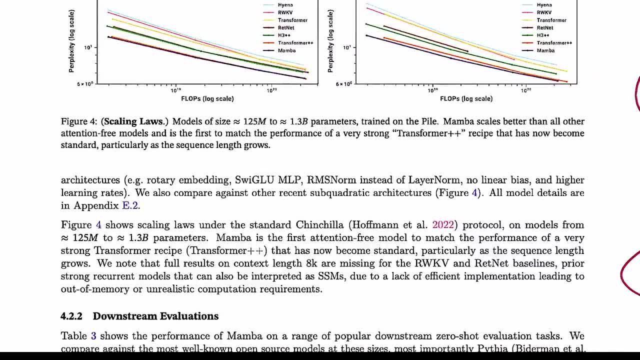 language modeling, and that is models trained on the pile up to 1.3 billion parameters, scales better than all other attention free models and is the first to match the performance of a very strong transformer++ recipe. that has now become the standard, particularly as the sequence length grows. 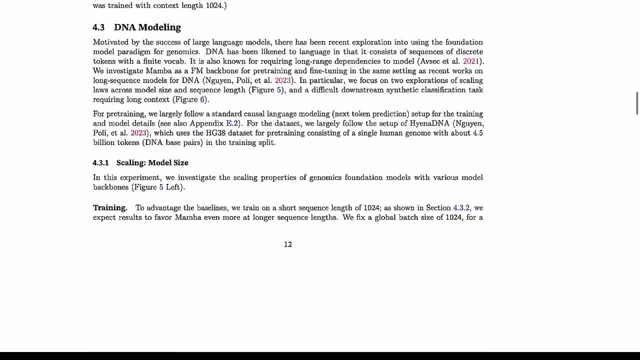 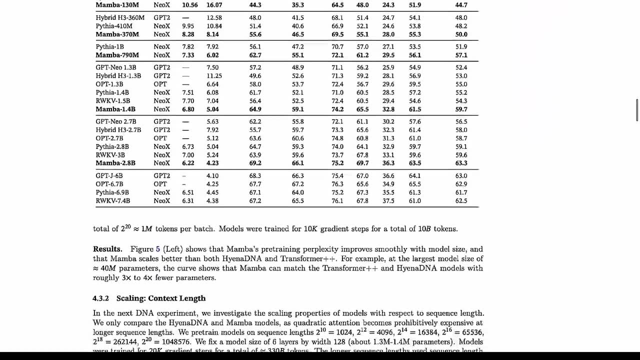 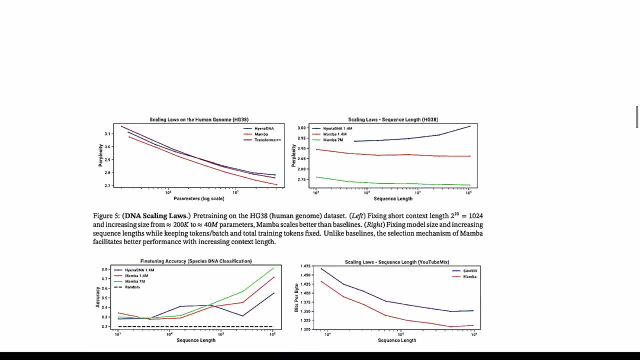 so the jury is still out at really large scales, but already at this scale this looks quite promising. DNA modeling and so on, mamba superior to other things? yeah, because long sequence lengths are really the strength of these kinds of models. and again, we'll have to see. 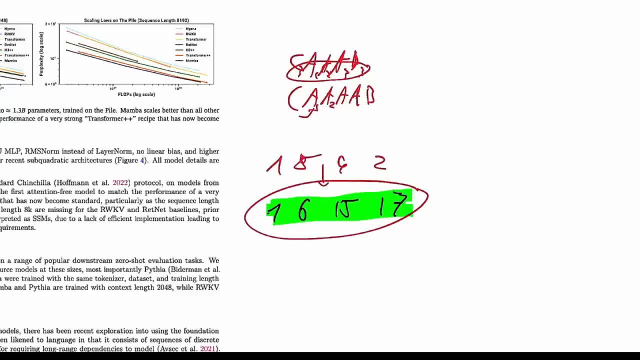 And then you can use those. And for example, if you say, what's the sum from here to here, you can just subtract from 17, you can subtract six or one, sorry, one. And you can say, oh, the sum here is 16 without having to compute it again. 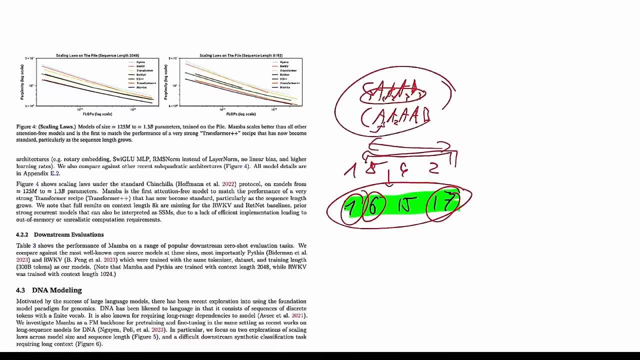 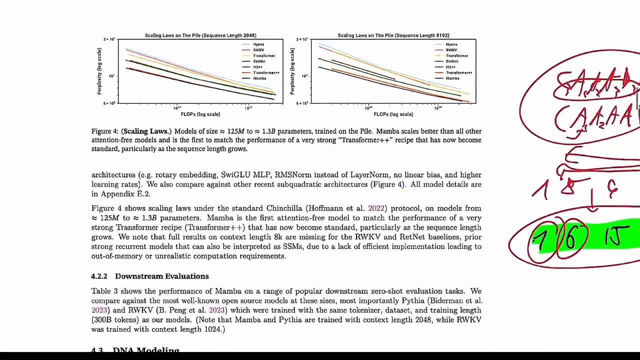 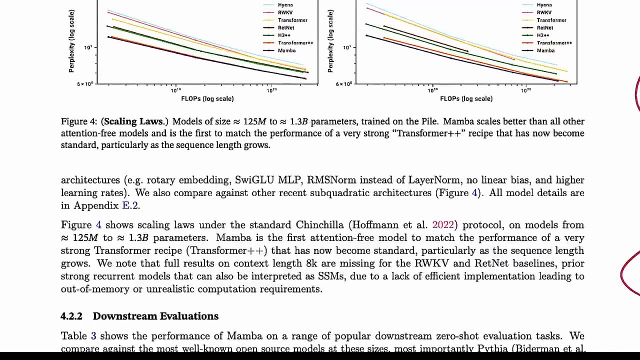 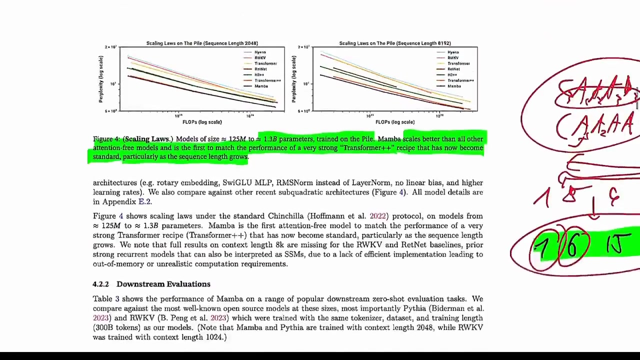 Same principle goes for how they make this here fast. The scaling laws look really scaly. So the perplexity in language modeling, and that is models trained on the pile up to 1.3 billion parameters, scales better than all other attention-free models. And there is the first to match the performance of a very strong transformer plus plus recipe that has now become the standard, particularly as the sequence length grows. So the jury's still out what happens at really large scales, but already at this scale, this looks quite promising. 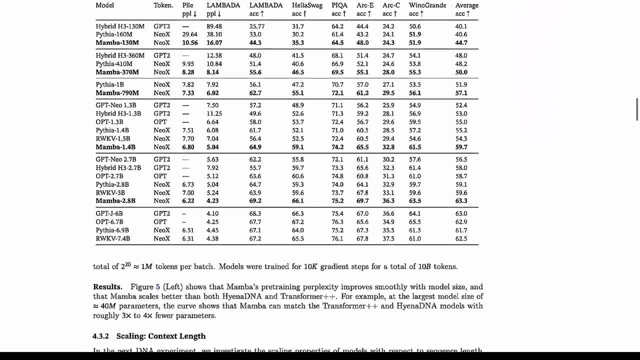 DNA modeling and so on, Mamba superior to other things. 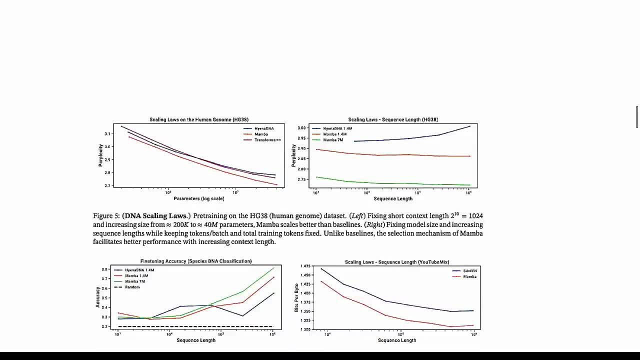 Yeah, because long sequence lengths are really the strength of these kinds of models. 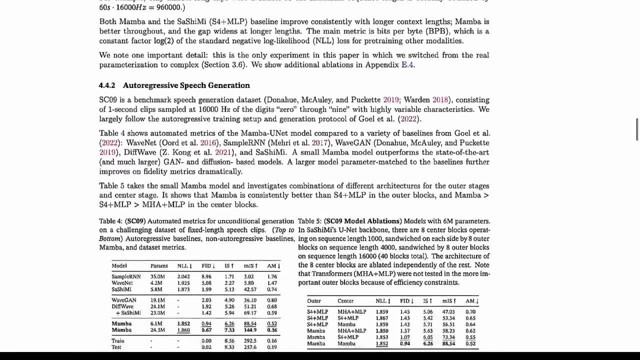 And again, we'll have to see what the exact trade-off is going to be, 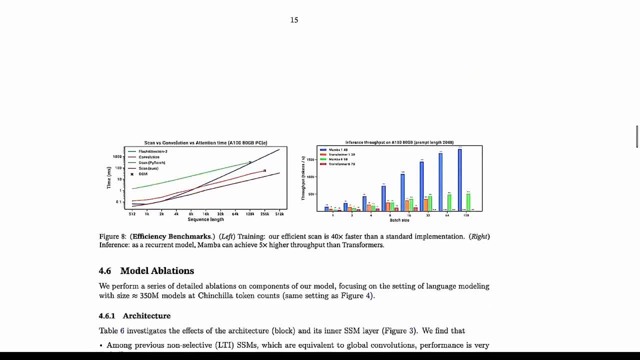 whether we need to make the, the transformation, transitions input dependent or not. 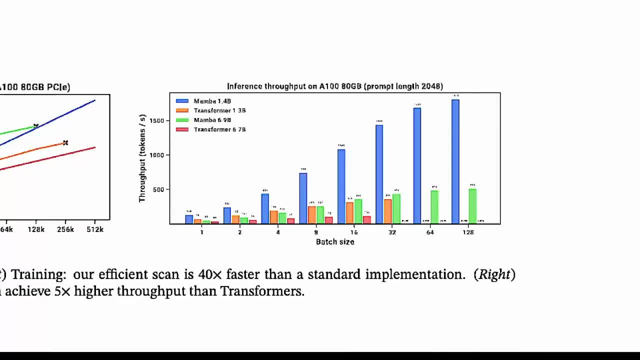 And yeah, you can see that inference throughput on an A100 is good and actually gets more drastic 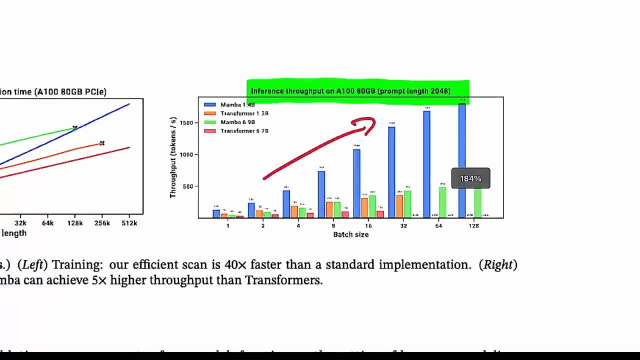 and drastic as the batch size increases when you compare them to transformers. 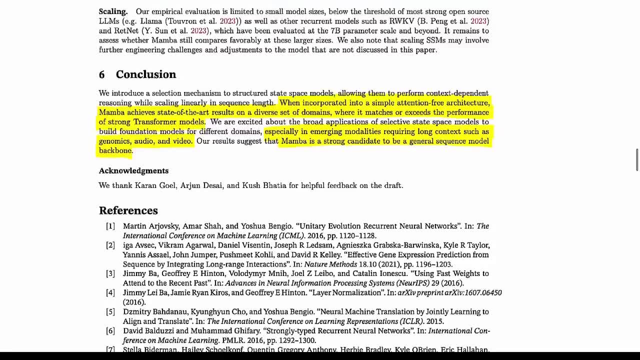 All right. They have some ablations here. They say Mamba is a strong candidate to be a general sequence model backbone. 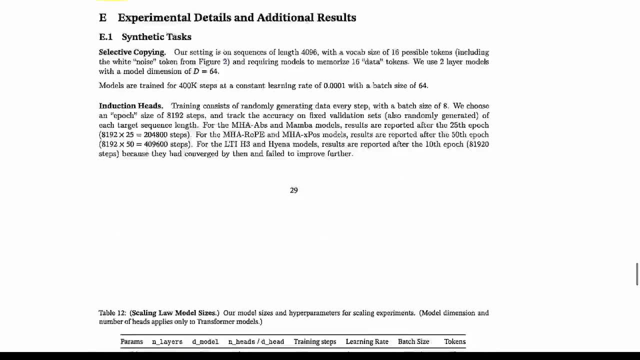 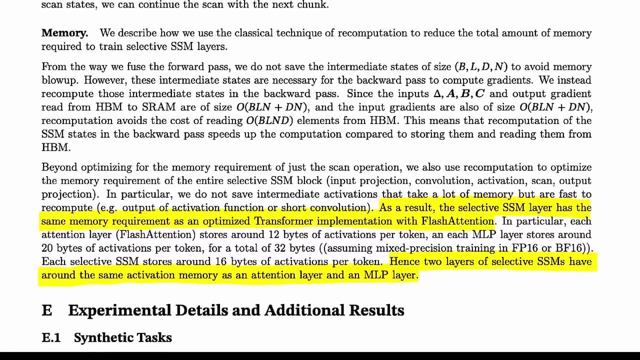 And lastly, I think I have one more highlighted section where they discuss the intricacies of the, of the, of their efficient implementation. 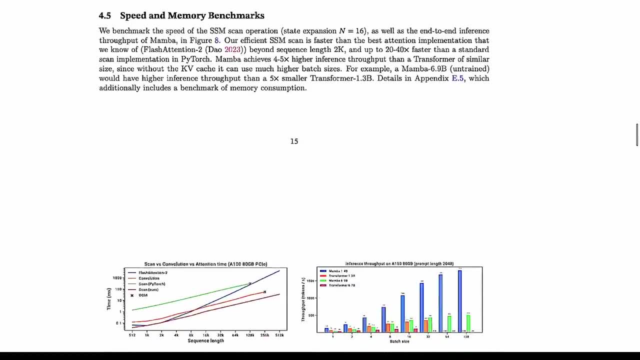 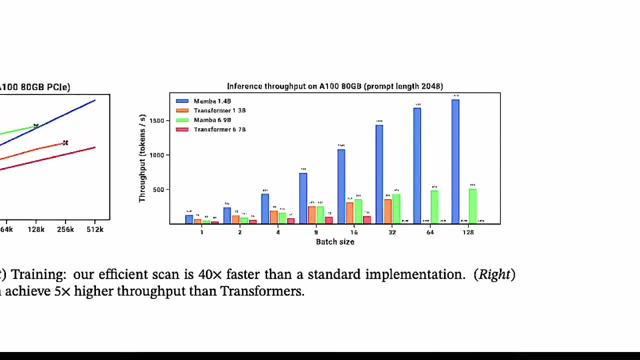 what the exact trade off is going to be, whether we need to make the, the transitions, input dependent or not. and yeah, you can see that inference throughput on an A100 is good and actually gets more drastic and drastic as the batch size increases when you compare them to. 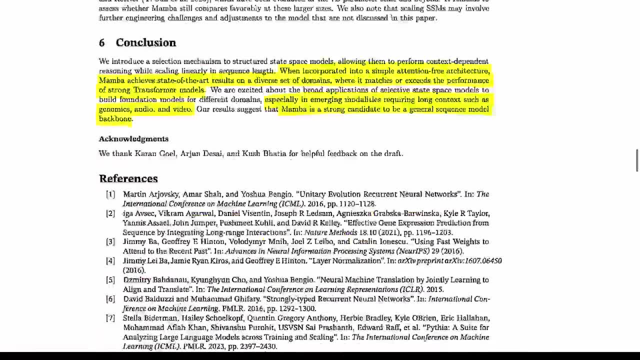 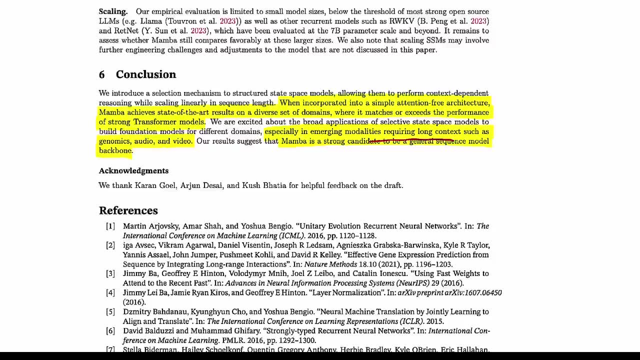 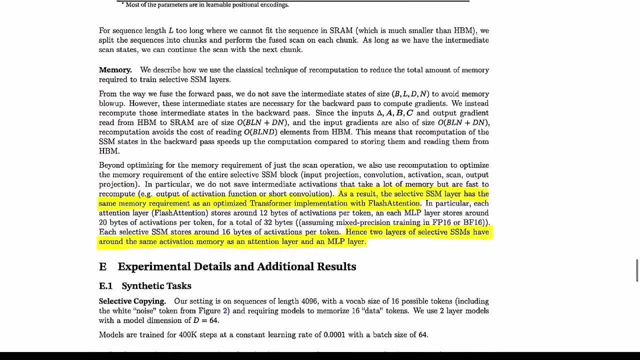 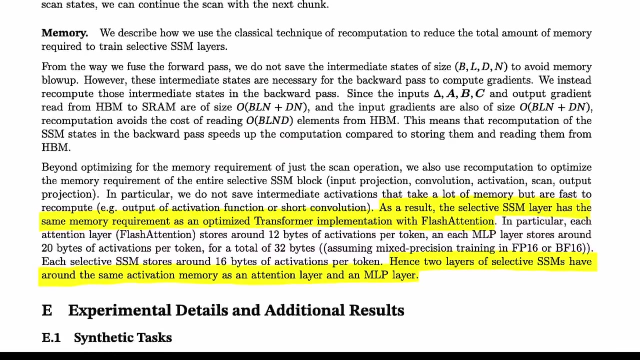 transformers. alright, they have some ablations here. they say mamba is a strong candidate to be a general sequence model backbone. and lastly, I think I have one more highlighted section where they discuss the intricacies of the of the of their efficient implementation. this section is also good. 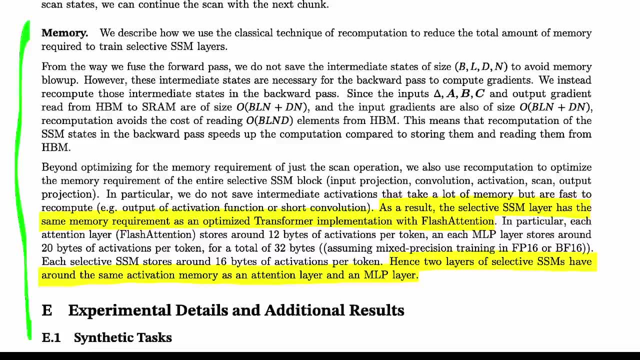 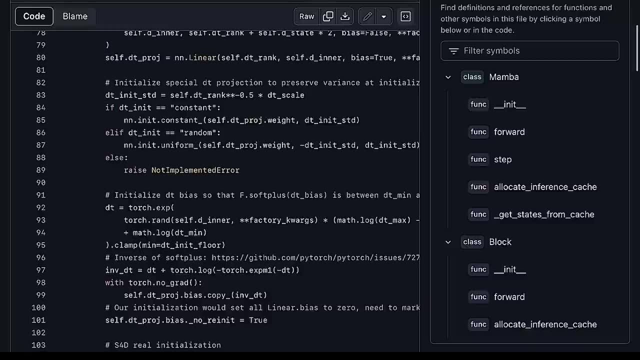 if you wanna dive deeper into this, you can go into this section especially. they discuss what they transfer, how much elements they transfer, what that costs and so on, so really reducing that memory transfer. and lastly, you can also dive into the code here on github, if you do. I invite you to look at this mamba simple. 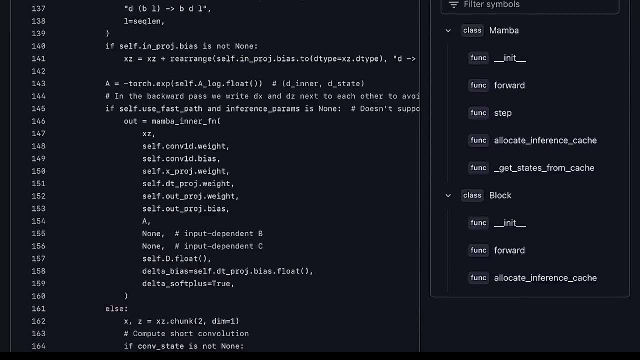 and in fact in this codebase the same thing is going to be implemented multiple times: one time for python, one time for gpu, and then again one time for inference, where you do things recurrently, and one time for training, where you compute everything kind of at the same time. 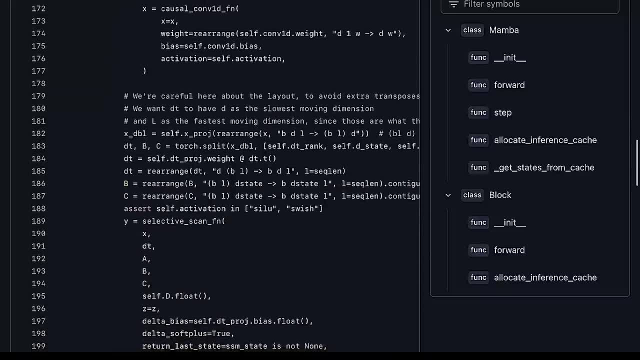 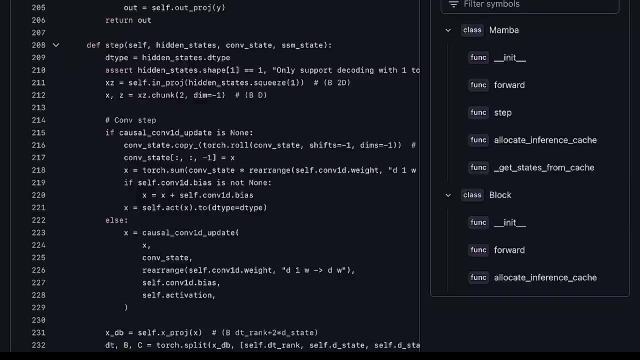 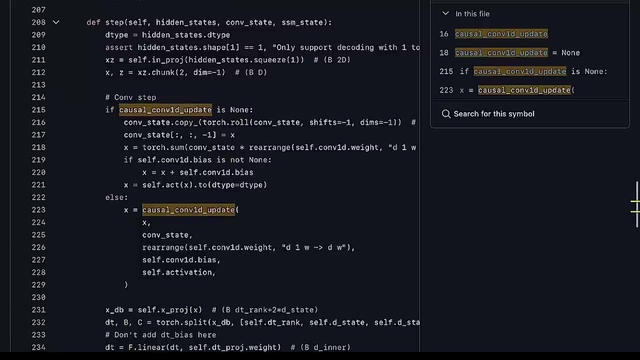 and so you'll find the same code written many, many times in different ways. I invite you to look at this step function right here, which is really, really good, and just assume you don't have any of the extras, so like this. causal conv 1d update. 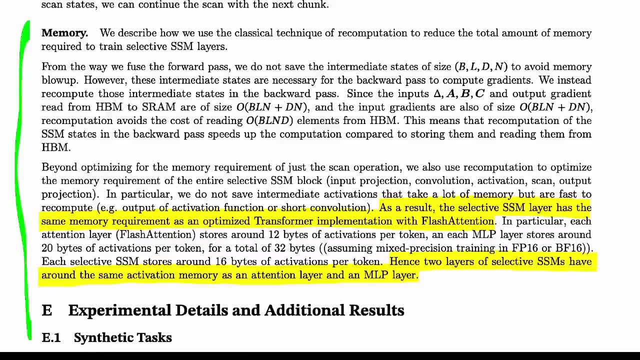 This section is also good. If you want to dive deeper into this, you can go into this section, especially they discuss what they transfer, how much elements they transfer, what that costs and so on. So really reducing that memory transfer. And lastly, you can also dive into the code here on GitHub. 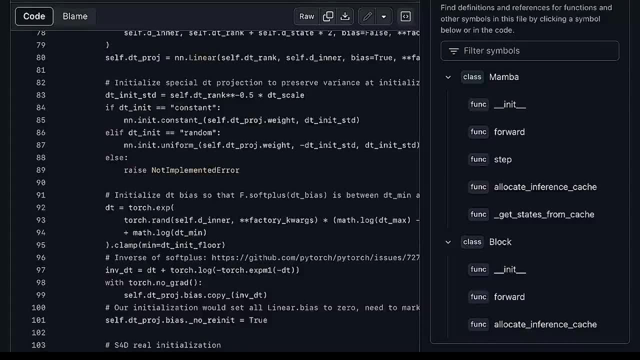 If you do, I invite you to look at this Mamba simple pie first. 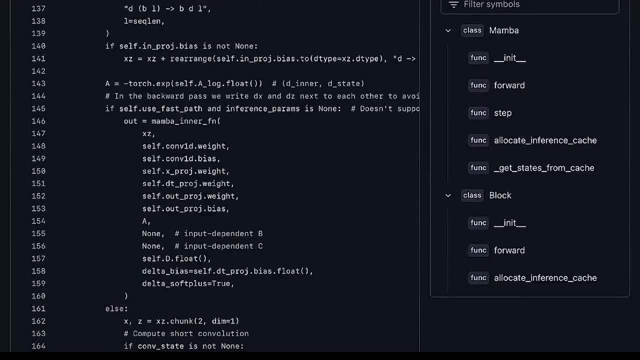 And in fact, there in this code base, the same thing is going to be implemented multiple times, one time for Python, one time for GPU. And then again, one time for inference where you do things recurrently and one time for training where you compute everything kind of at the same time. 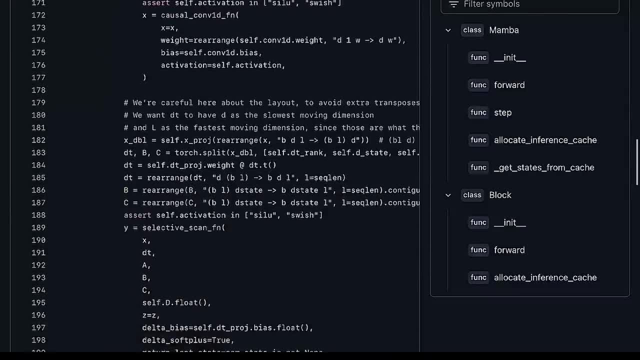 And so you'll find the same code written many, many times, in different ways. 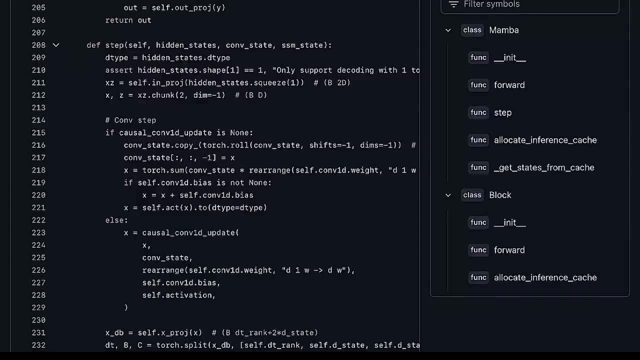 I invite you to look at this step function right here, which is really, really good. And just assume you don't have any of the extras. 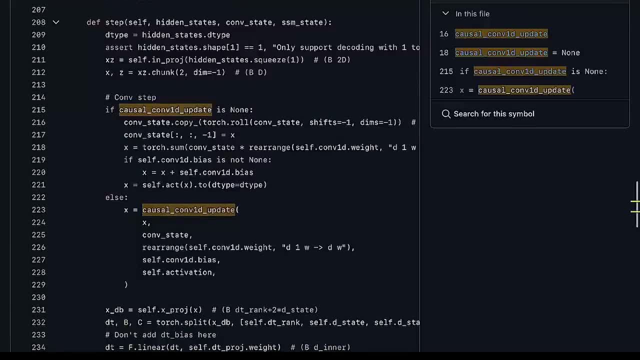 So like this causal conv 1D update, because that gives you a good idea. So see, there's first an input projection. 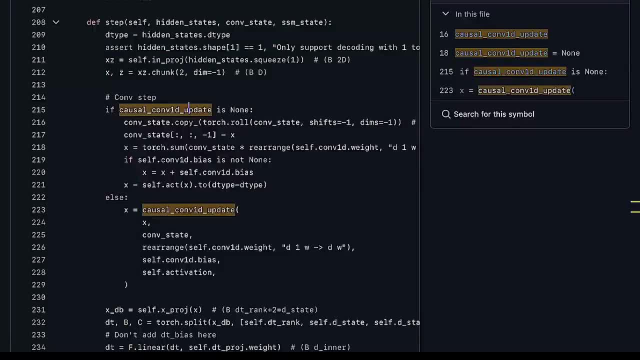 Then there is a conv 1D, like a convolution, 1D convolution. 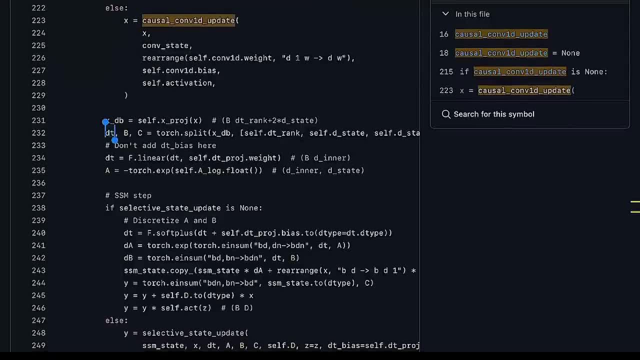 Then there is, then the, the parameters here are, this DT, they talk about sort of projecting this down and up and kind of putting it through a dimensionality bottleneck. 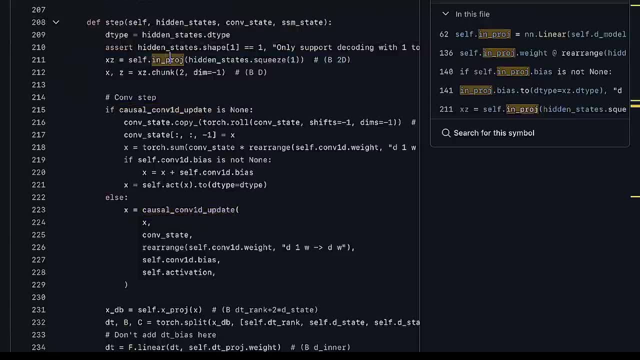 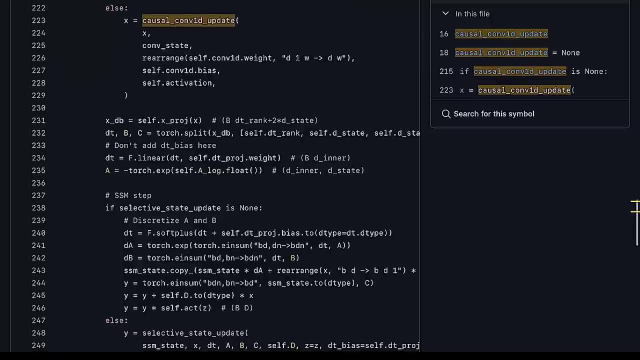 because that gives you a good idea. so see, there's first an input projection, then there is a conv 1d like a convolution 1d convolution, then there is then the parameters. here are this dt- they talk about sort of projecting this down and up and kind of putting it through. 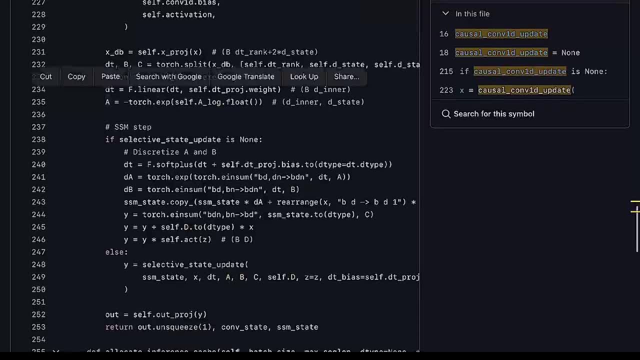 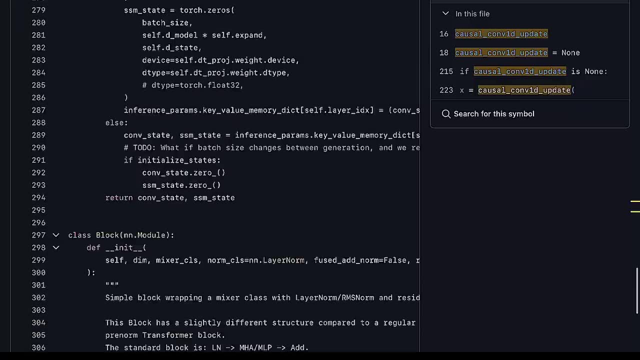 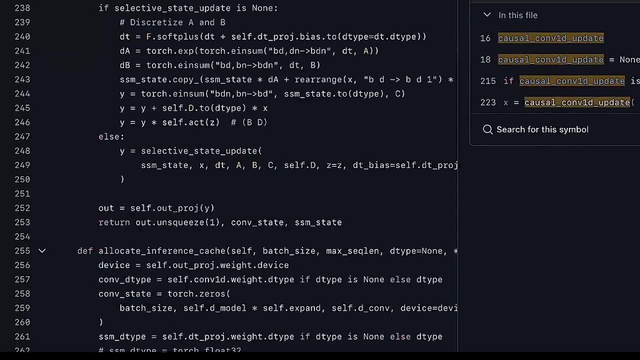 the three dimensionality bottleneck. the matrix A is a parameter. it's just stored as log A and not as A itself. where was I? where was I? oh, here then we do the discretization. the discretization goes, you can see, here discretization is done by multiplying. 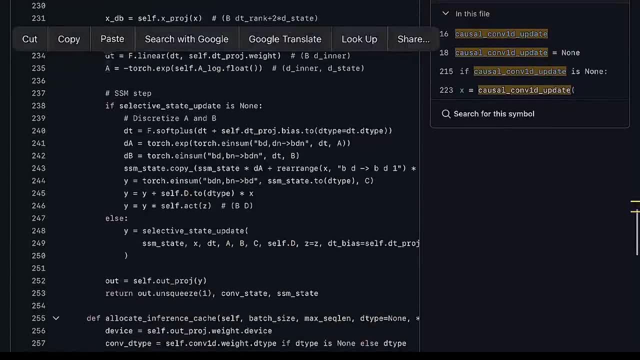 The matrix A is, is a parameter. 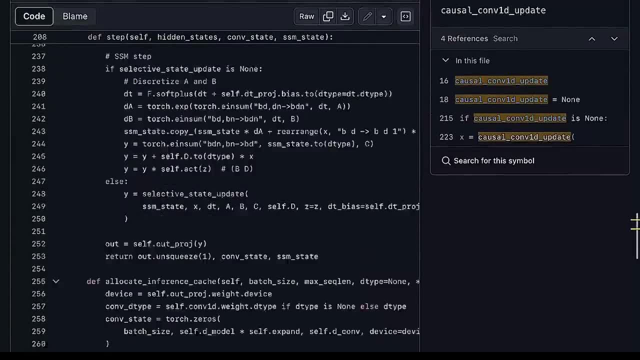 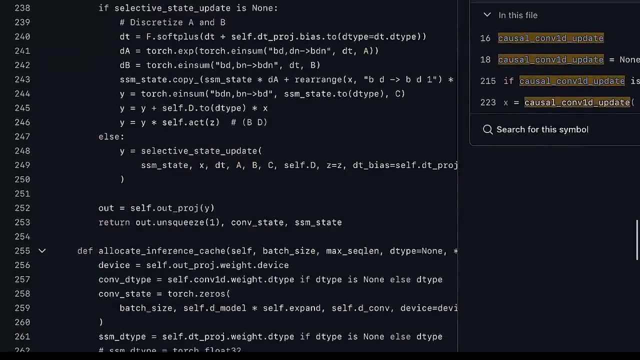 It's just stored as log A and not as A itself. Where was I? Where was I? Oh, here. Then we do the discretization. The discretization goes, you can see here, discretization is done by multiplying this DT to A. 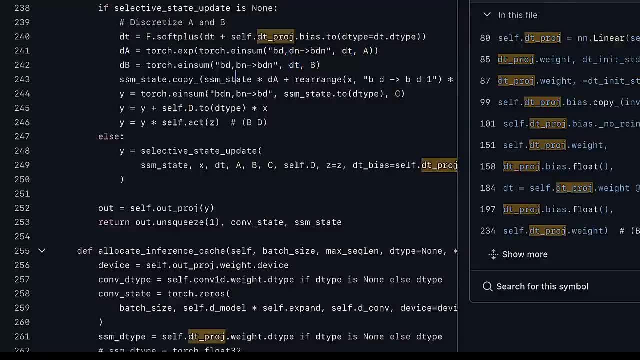 This DT to B. Then the recurrence is calculated. 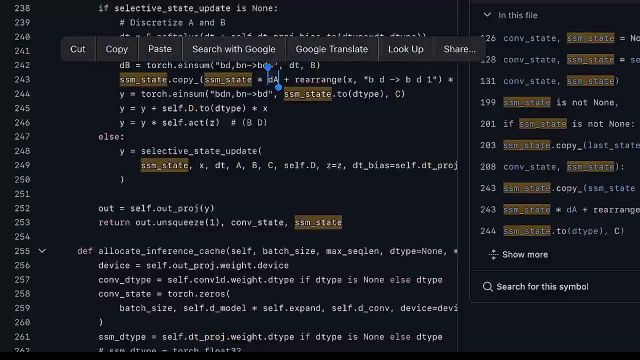 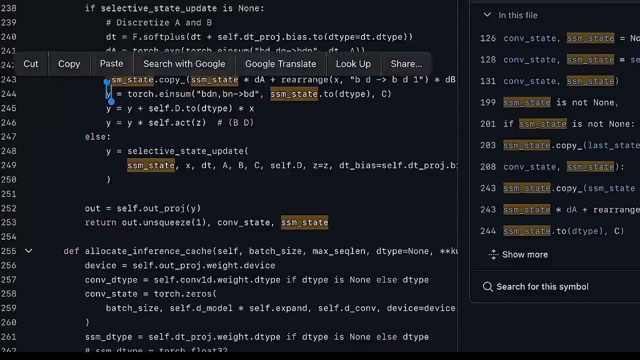 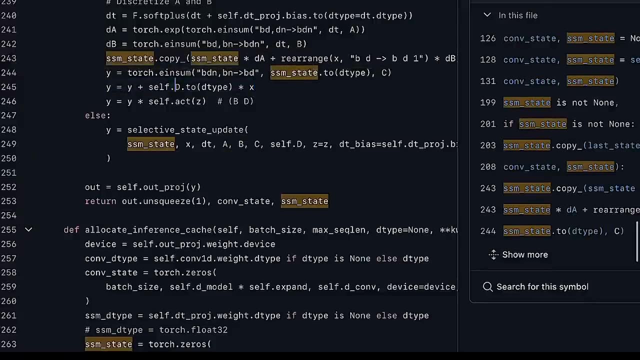 The state times DA plus X times DB. So this is the main recurrence for the hidden state. The output is calculated by just multiplying the hidden state by C. And lastly, there, there's a recurrent, there's this gating connection in D, which is exactly what we saw in the paper in this architecture diagram. 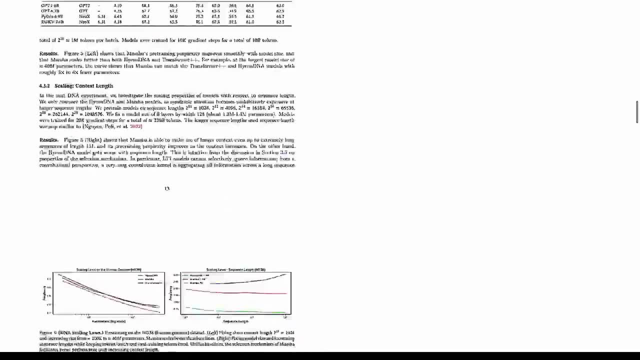